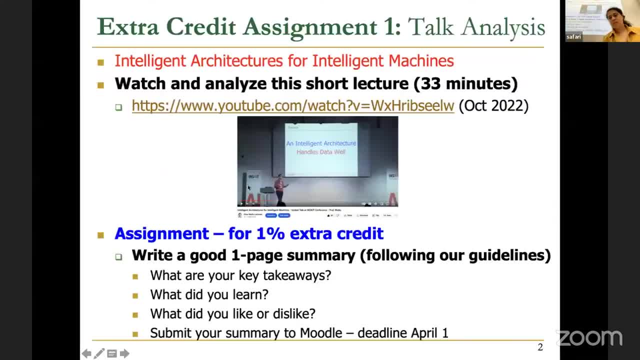 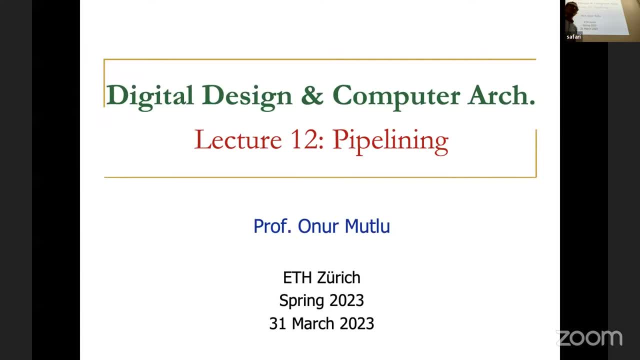 Okay, And can people online hear us? I hope so. Okay, good, So let's get started. Too many technical issues again. Wow, that's a small group today. Is it because of the weather? Because of something else? I don't know. 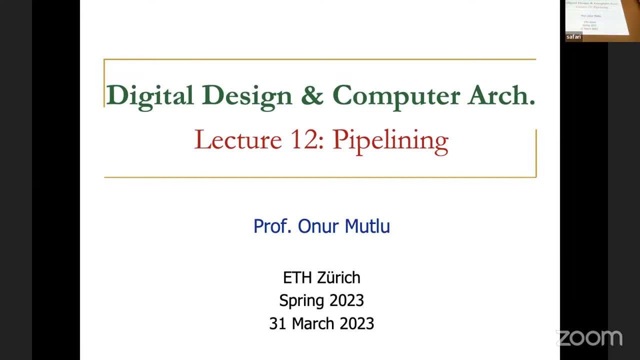 Okay, hard to tell, Maybe there are people online, But this is an important topic. Okay, everything works fine, That's good. So, yeah, this is an important topic that we're going to discuss. As I mentioned yesterday, we're going to improve performance. 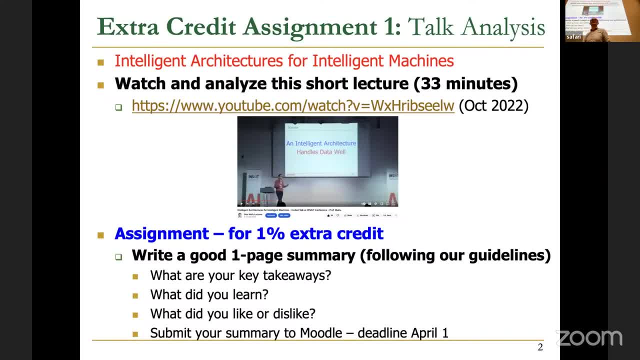 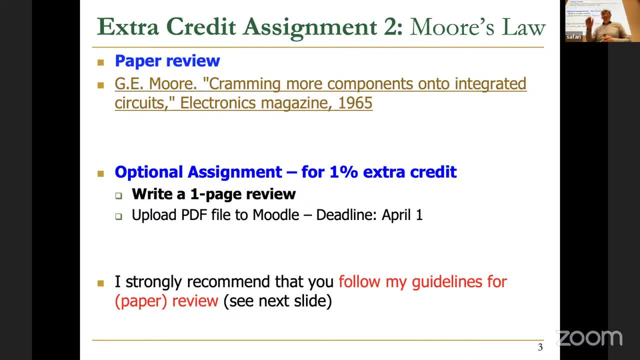 But before we do that, I guess, a final reminder, because this is due today or tomorrow. Hopefully you're doing it. How many people did these reviews? Okay, that's good. Maybe I should stop reminding people, But they're always stragglers at the end. 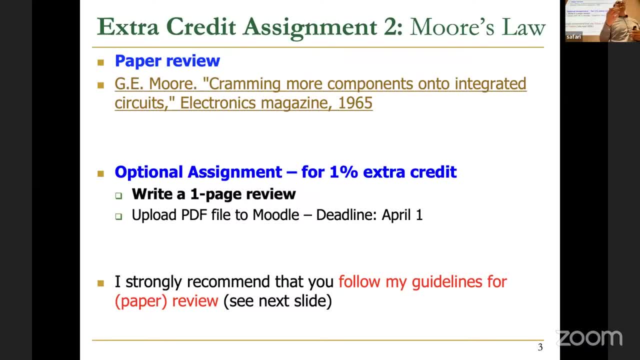 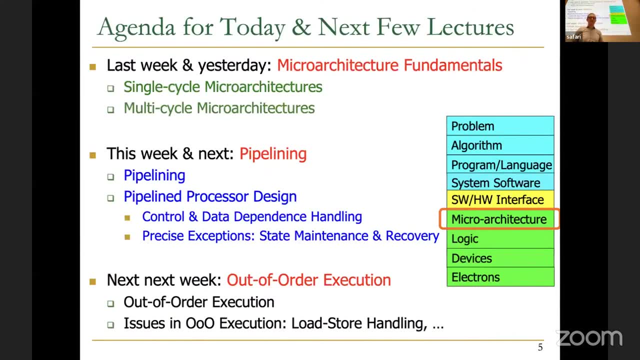 Did you enjoy reading the papers? Yeah, They're a bit old, But well, the story The second one is a bit old. This is relatively new actually. Yeah. Okay, Let's not waste more time. We've already discussed Moore's Law. 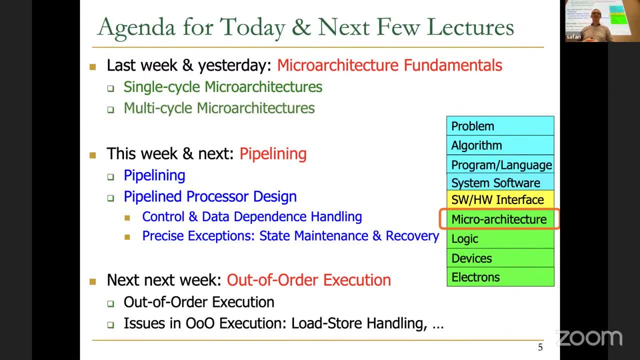 But today we're going to jump into pipelining: Now that we've covered the basics of microarchitecture fundamentals, develop single cycle architectures, microarchitectures and then multi-cycle microarchitectures to improve on single cycle. Today we're going to improve on the multi-cycle microarchitectures. 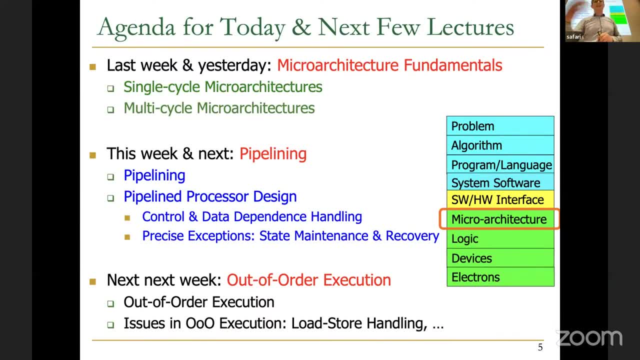 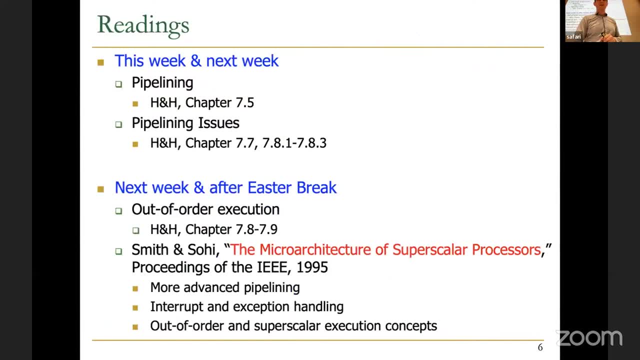 And then we're going to continue with this next week, And then next next week, meaning after Easter break, we're going to talk about out-of-order execution and precise exceptions, potentially during that time as well. And these are your readings. 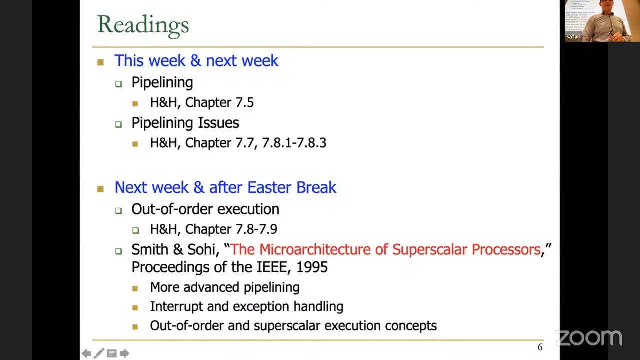 I'd recommend doing them, And we're going to cover things that are not covered very well in your books from now on, especially after Easter break. This paper is a very nice overview of how modern processors work. So they talk about advanced pipelining, inter-epidemic exception handling. 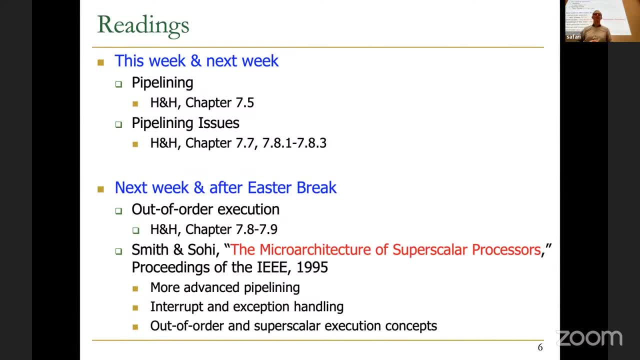 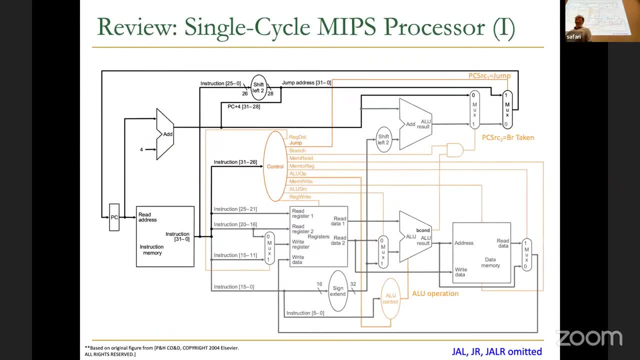 out-of-order and superscale execution, So this is a paper that I would strongly recommend that you read. Okay, this was the single cycle MIPS microarchitecture that we developed in lectures. Everybody remembers this. This is easy by now, mostly. Okay, that's good. 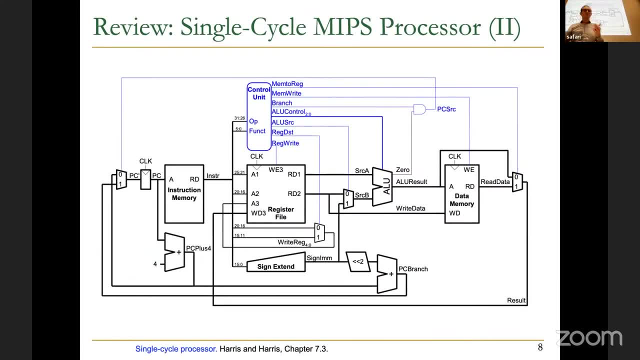 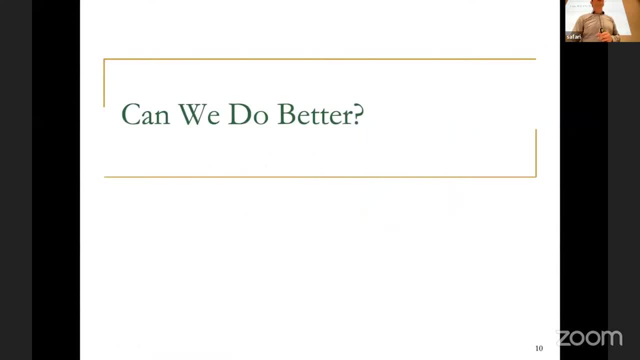 And this is the single cycle MIPS processor that we somewhat looked at, but it was mainly in your book. And this is a single cycle MIPS finite state machine And we asked the question: can we do better compared to single cycle? And we developed multi-cycle. 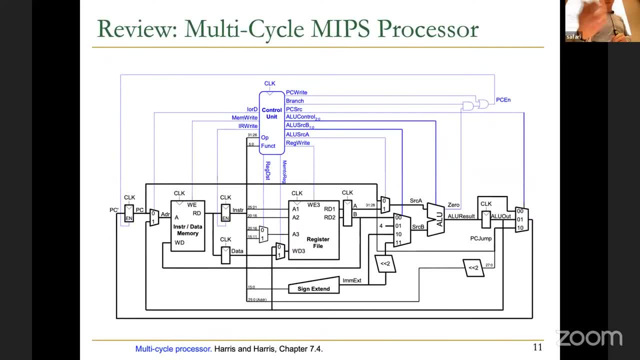 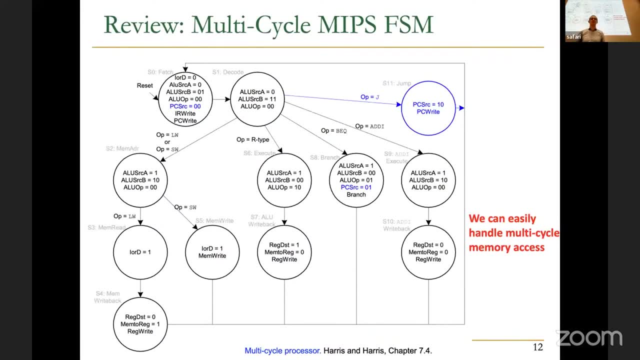 MIPS- microarchitectures or microarchitectures in general- And we actually developed this almost in full and we covered this yesterday. And we also developed this multi-cycle MIPS- finite state machine- in full And we actually said that we can easily handle multi-cycle memory access. 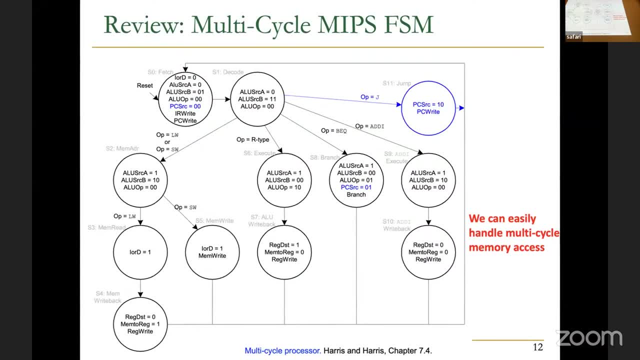 with this sort of machine or very long memory accesses, by staying in the memory access state long enough, such that you get the data back from memory. So this is a lot of advantages that we discussed last time, But now the question is: can we do better? right? 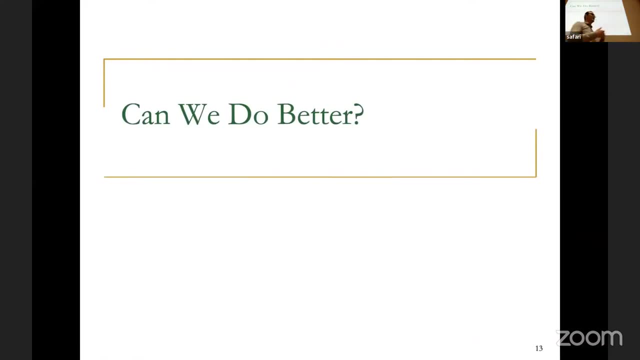 We never are content with what we do. We want to do better, and better in this case is mainly for performance. Can we improve the performance of this multi-cycle machine and do something? let's say higher performance? So this of course, requires you to critically think. what are the limitations in this design? 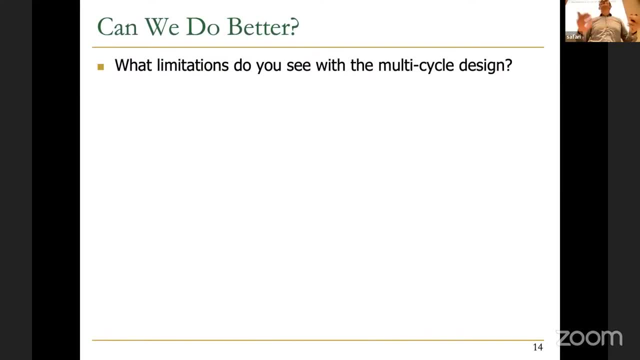 in this multi-cycle design, Anybody? Do you see something obvious that you can improve? Okay, Yes, say it again. Yeah, you need registers to save the data. Maybe you can reduce those. That's what you're saying, but I'm asking for performance. 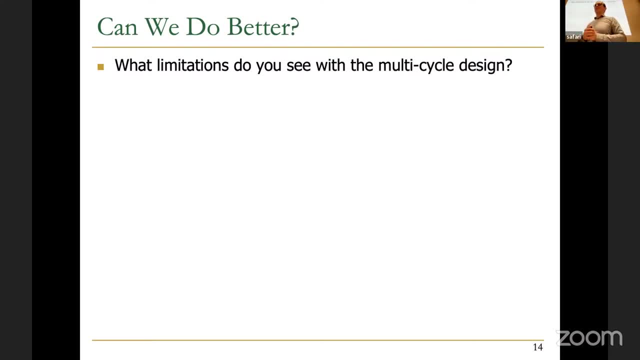 That's true, You can. Yeah, that's true. That's true, It does. That's the cost you pay for being multi-cycle. I would say: What else? Yes, Exactly, That's one thing. basically, You're doing nothing while you're waiting for the memory. 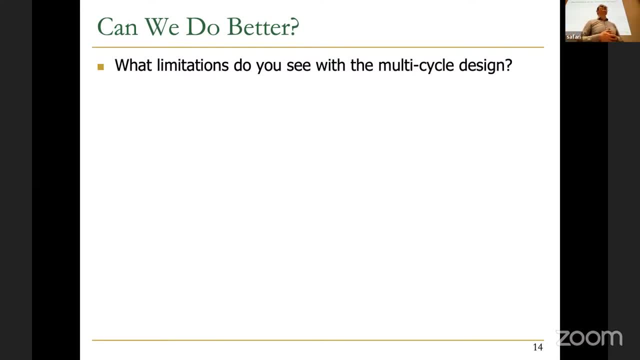 So you're not executing Basically, you're not exploiting the concurrency that may be present in the hardware right Enough, And I would say it's not just memory, It's actually other parts of the pipeline as well, And that's the main thing we're going to try to improve. 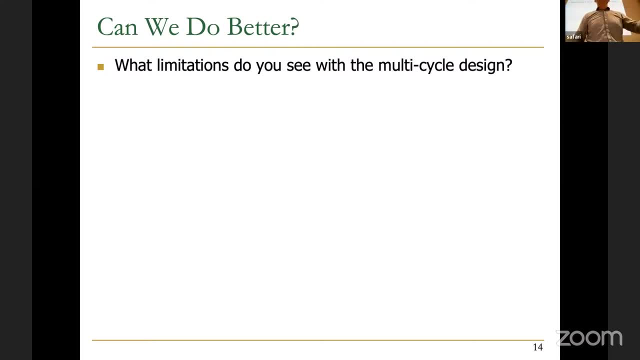 We're not going to specifically tackle the memory part, though That's going to still bite us in the future, as we will see, Yeah, Before the end of this class. So basically, we have limited concurrency. What does that mean? 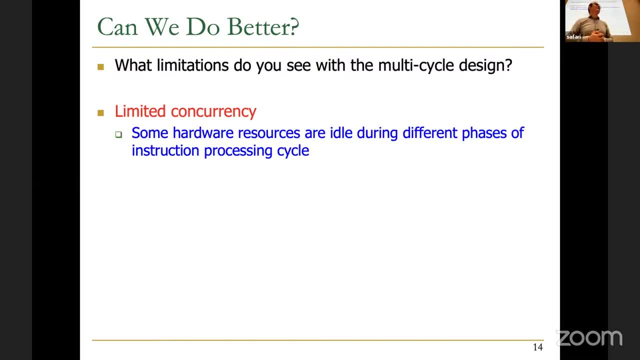 Some hardware resources are idle during different phases of the instruction processing or execution cycle. Let's look at an example. For example, the fetch logic that's at the front end of the machine that we have seen is idle when an instruction is being decoded. 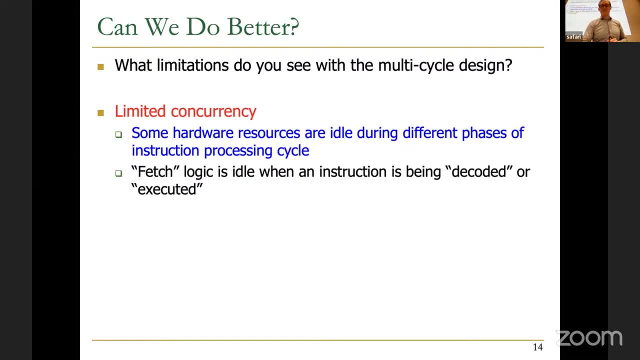 or it's being executed or it's doing a memory access right And most of the data path is idle. when a memory access is happening, actually You're accessing memory On the side And most of the data path is doing nothing, as your fellow student stated. 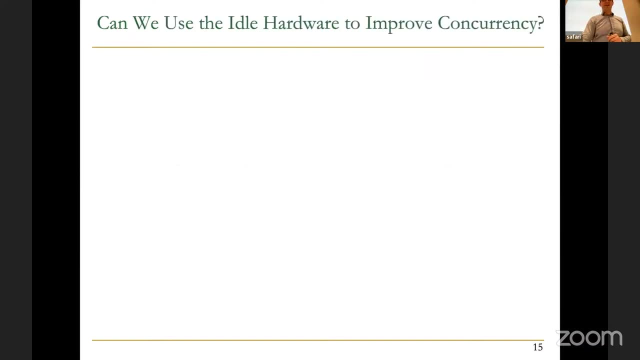 What's your name? Luis? Okay, As Luis stated. Okay. So basically, the key question to ask: once you realize this, you can improve on this, of course. right, And the key question to ask is: can we use this idle hardware to do something that would improve performance? 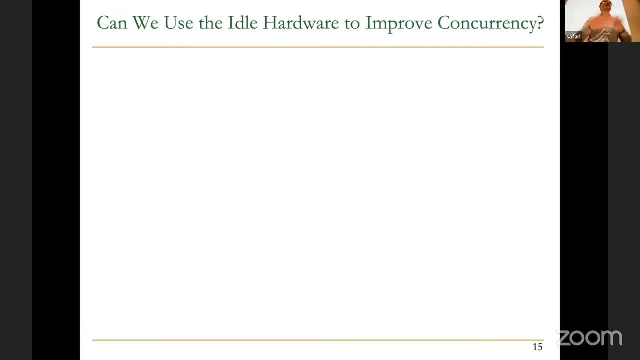 Basically to improve concurrency of processing, And we're going to violate the von Neumann principle at the microarchitecture level to do this. Basically, our goal is to have more concurrency. This will enable us to get higher instruction throughputs in the pipeline. 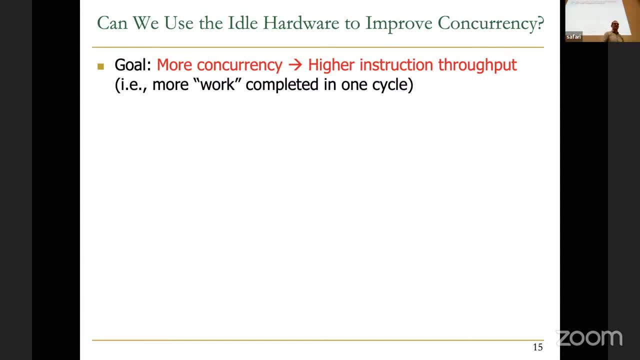 Throughput is work completed per unit time. That's the definition Basically. we want to do more work per cycle, let's say, or per any unit time, if you will. We're going to talk about throughput and latency also. Throughput is basically things done per unit time. 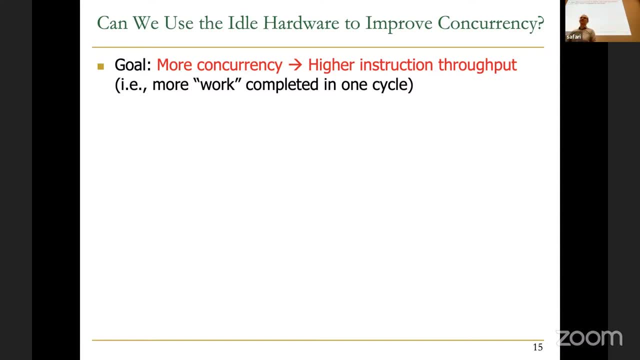 For example, number of data items fetched per second, gigabytes per second, for example. That's the throughput of memory. That's the unit with which the data is being processed. Right Throughput of memory is measured, But in terms of instruction processing- how many instructions you complete in a given cycle? 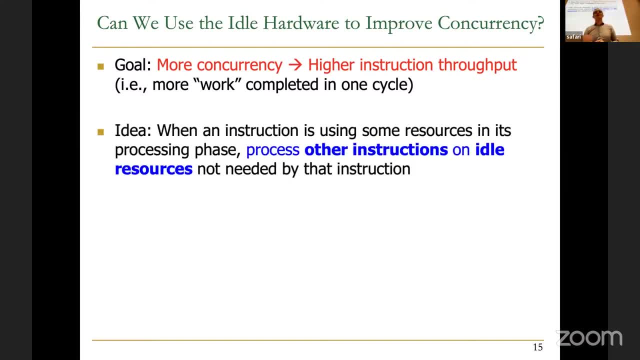 That's our throughput metric right now And you will see that. But basically the idea to improve this concurrency is, when an instruction using some resources in the processing phase it's currently in, why not process other instructions in the idle resources that are not needed by this instruction? 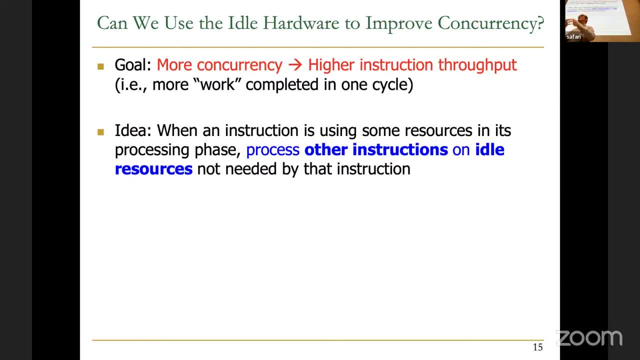 So we're going to bring in some other instruction to do, To be in some other phase of processing, while an instruction is another phase, And we're going to do this via pipeline. So, for example, when an instruction is being decoded, why not fetch the next instruction? 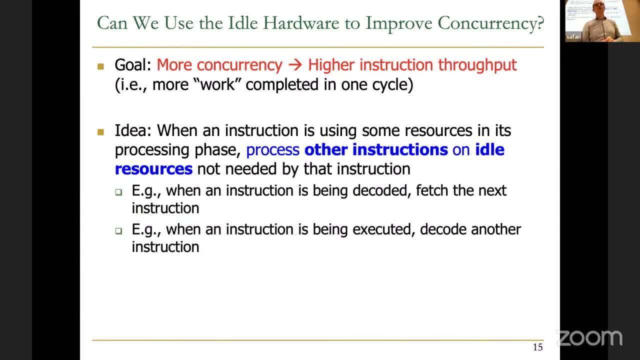 Because the fetch resources are idle When an instruction is being executed, why not decode another instruction, Probably the next sequential instruction, right? And when an instruction is accessing data memory, when you're doing a load or store, execute the next instruction. 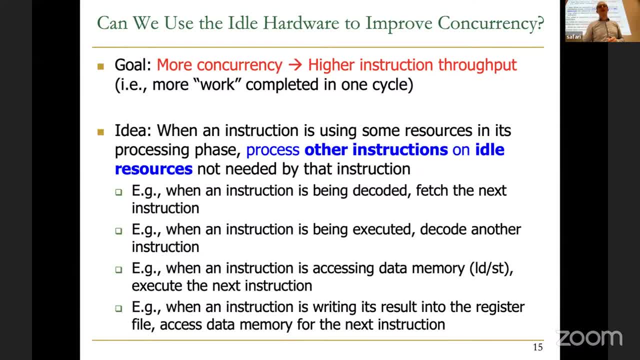 It could be in the execute phase, the next instruction, And when an instruction is writing its result into the register file, access the data memory for the next instruction. So basically you can pipeline the instruction processing this way, similar to an assembly line. 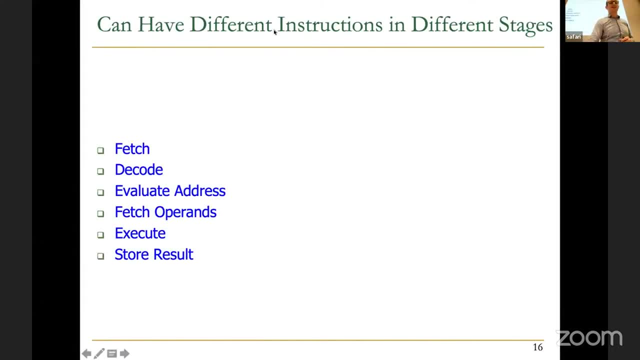 So let's take a look at this pictorially. Basically, these are the six different processing stages we have in the instruction processing cycle, And we've kind of reduced this to five when we designed the single cycle, microarchitecture and the multi-cycle. 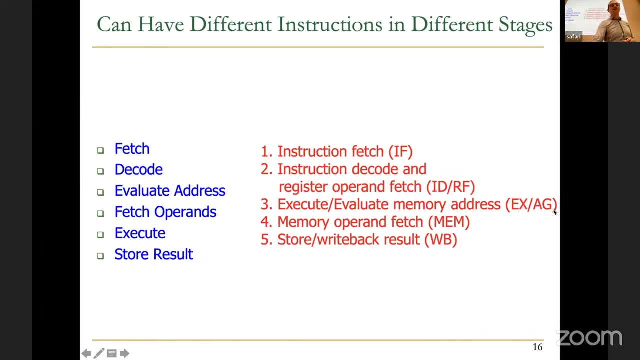 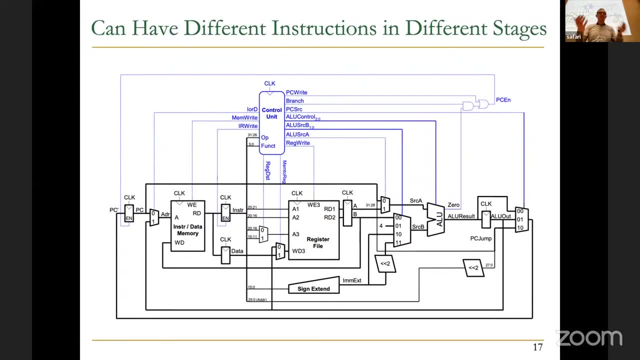 Basically fetch, decode and read register file And then execute And then generate address. These can be done concurrently- And then memory access and write back. And this was our multi-cycle microarchitecture But we're going to go back to the single cycle also. 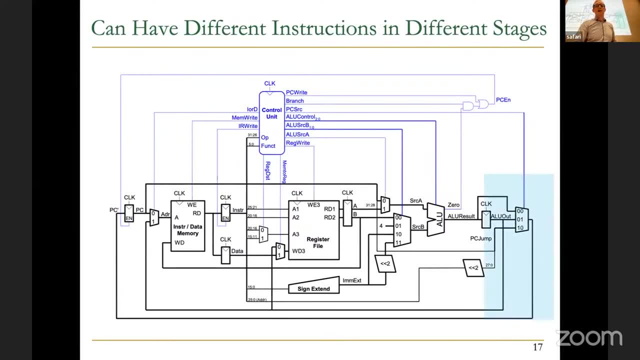 But it doesn't matter. The key idea is, while an instruction- this blue instruction- is writing back its results, a yellow instruction, which is the next instruction, is doing something in this particular stage. It could be executing in the ALU or it could be generating address, for example. 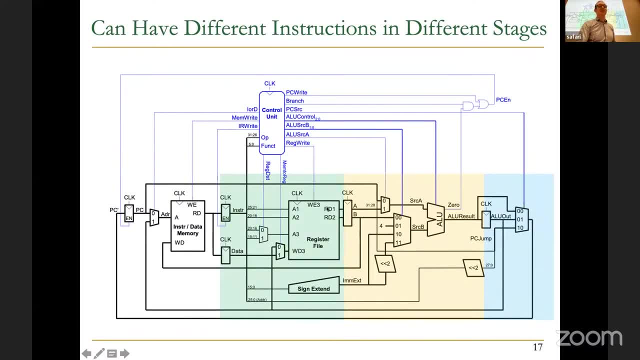 And a green instruction, Which is the next instruction in the sequence, is accessing the register file and being decoded, And a red instruction is being fetched at the same time. So that's the basic idea: Fill the hardware resources with different instructions, sequential instructions in this case. 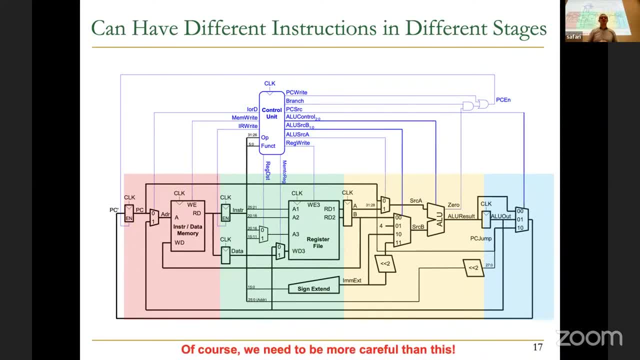 We're going to break that later on. Of course, we need to be more careful than this right, Because these instructions may be the next instruction, may be dependent on the previous instruction, Maybe using a register, for example, That an older instruction is producing. 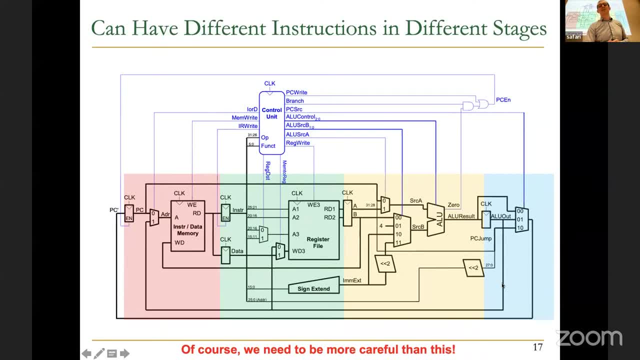 Right. So basically this, you can think of this as the oldest instruction in the machine. This is the next oldest, This is the next oldest And this is the youngest instruction, And I've just color coded them. So that's the idea. 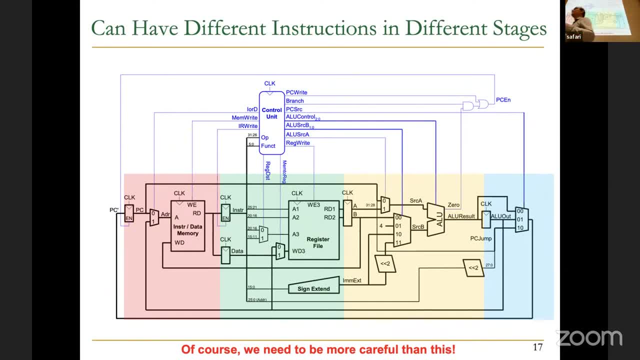 How do we, how do you bring more instructions into the machine such that they're concurrently processed? except different instructions are different stages of processing Make sense. Okay, That's how we can improve concurrency, And this is what's called pipelining. fundamentally, 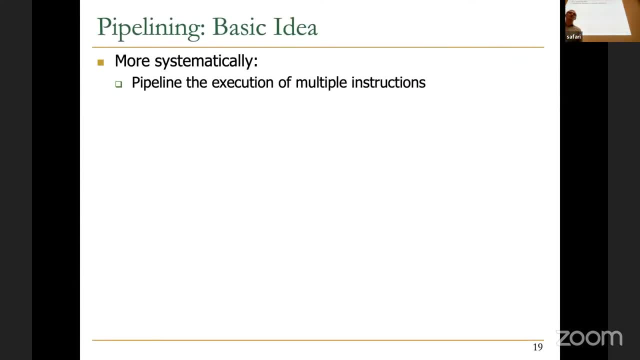 So basically, it's systematically, We would like to pipeline The execution of multiple instructions. It's, and the analogy is the assembly line, processing of instructions, And we're going to see some pictures from all the assembly lines, let's say, and new ones. 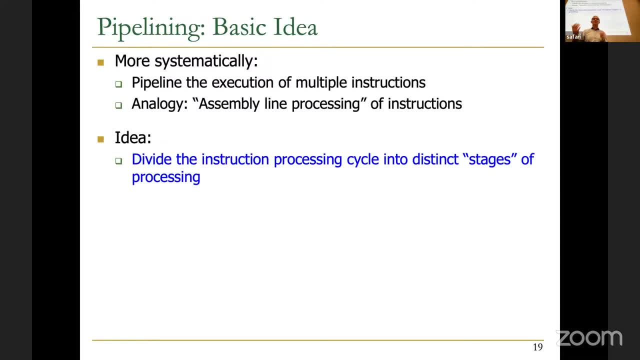 And the idea is to divide the instruction processing cycle into distinct stages of processing and ensure that there are enough hardware resources to process one instruction in each stage. That's going to be important, because we may need to replicate resources, as you will see, and to process a different instruction in each stage. 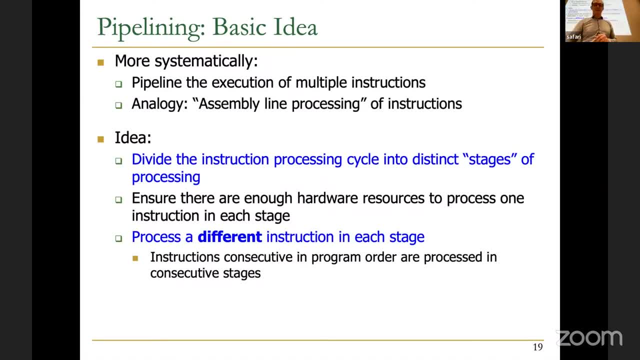 And instructions- Consecutive and program order- are processed in consecutive stages And the huge benefit is improving concurrency, In other words improving instruction processing throughput, In other words how many instructions you finish or complete per cycle, And we've kind of seen this right in the performance equation. 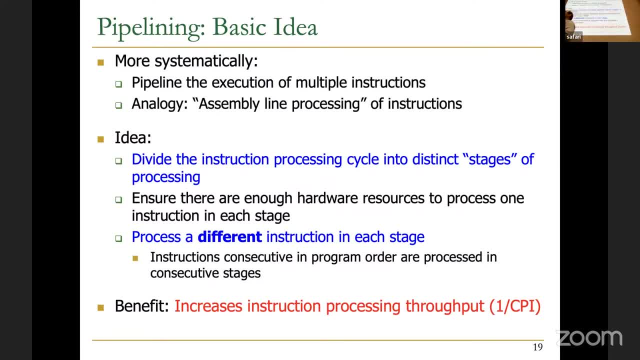 If you remember cycles per instruction, that's really the inverse of throughput: One over IP, one over CPI. is IPC basically CPI, How many cycles, how many a number? Uh, what is the average? The average number of cycles you, uh uh, you consume to actually finish an instruction, and IPC is how many instructions you finish per cycle. 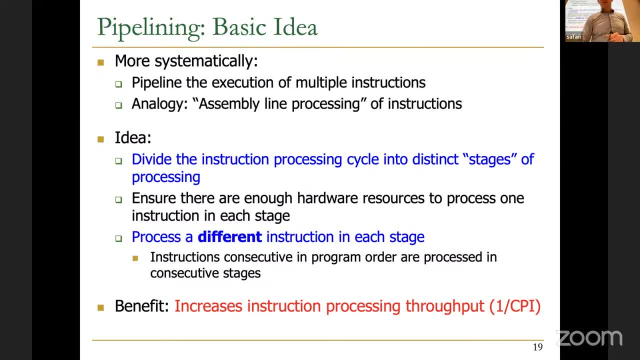 They're exactly immerses. Okay, So this is good, but remember, but I also said that whenever you do this, your flat clock frequency may hurt, and that it's actually true in this case also. uh, you will see that, but there are also downsides, and start thinking about this. whenever you actually have something like this, you're going to increase hardware a little bit. 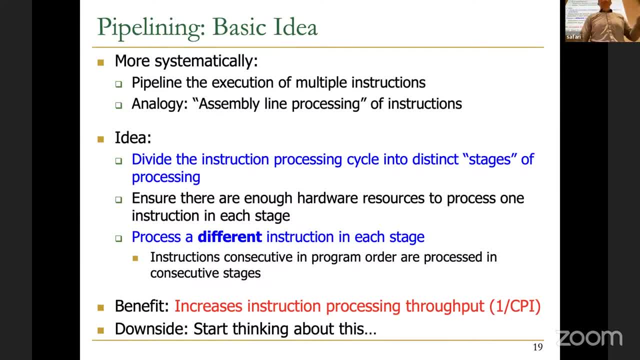 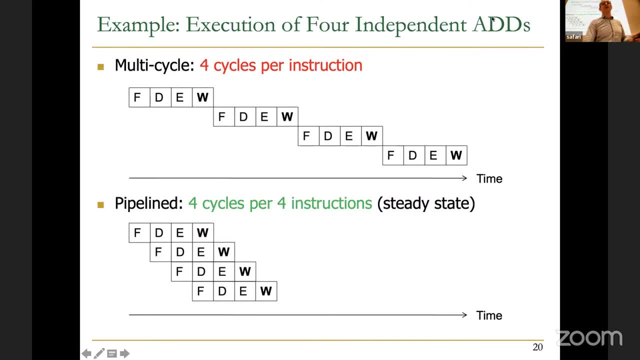 Okay, Any questions? now I give you the basic idea. The rest is going to be how we actually make it work. but let's look at it more conceptually a little bit more, with pictorial. let's say so. assume that we have four independent ad instructions and assume that in a multi-cycle processor each ad takes four cycles: fetch, decode, execute, write back. 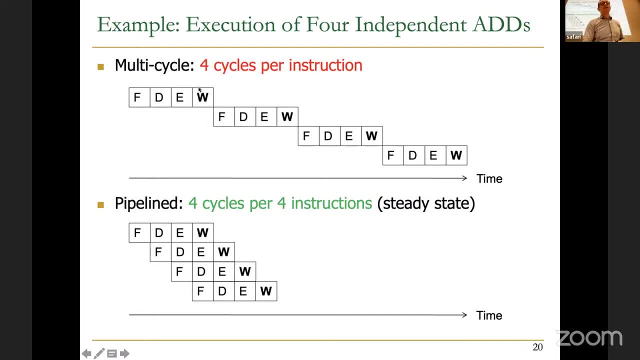 I simplified it a little bit: uh, in a multi-cycle processor, you finish four. uh, basically, you finish one instruction in four cycles. Uh, because you have no overlapping across different instructions. add one, add two, add three, add four. 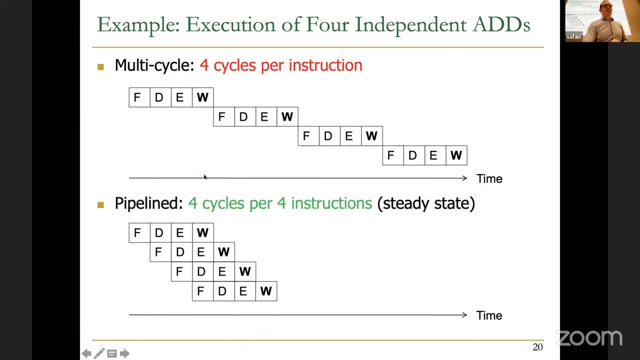 But- and I'm assuming that these are independent ads for now- Uh, if you have a pipeline processor, what you do is, while you're fetching the second instruction, while you're decoding the first instruction, you fetch the next instruction. While you're executing the first instruction, you decode the second one and fetch the next one. 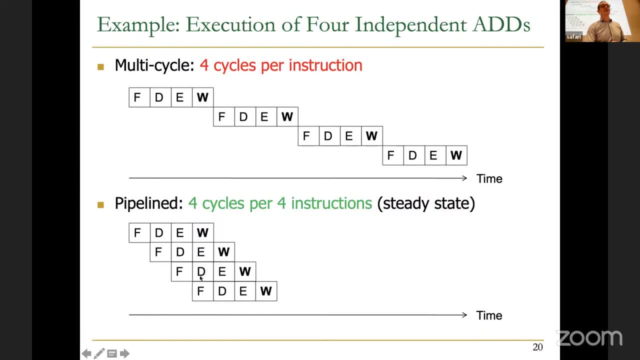 While you're writing back the result of the first one, you're executing the next one, decoding the next one and fetching the next one. So if you look at this, at this point your pipeline is full, meaning your processor is full with four instructions. assuming that you have four distinct stages like this, your processor is full with four instructions. 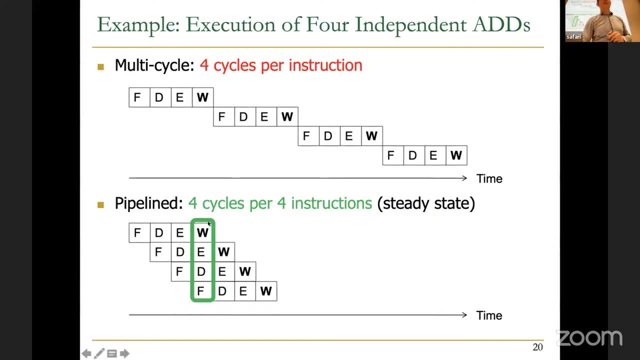 So, in the steady state, what you're doing is spending four cycles for four instructions. In other words, you're completing one instruction every cycle, right? You're completing this instruction, this cycle, this instruction, the next cycle, this instruction, the next cycle, this instruction, the next cycle. 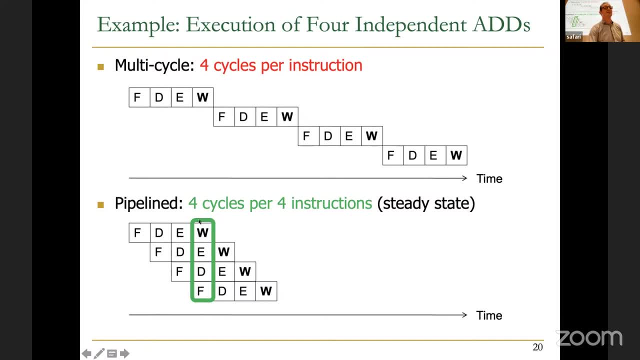 So it takes some time to fill the pipeline, as you can see. But once the pipeline is full, meaning the steady state you start completing one instruction per cycle Make sense And that's the throughput benefit. Now realize that we did not change the latency of a single instruction. 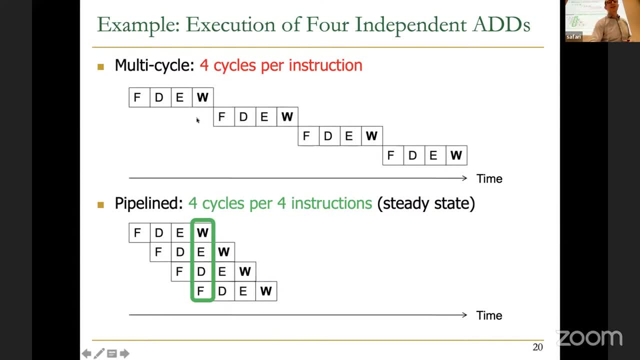 That's the difference between latency and throughput. The latency of each add is constant. You will take what we're going to discuss later on. It's basically four stages right. Each add takes the same amount of time, But overall the program takes shorter. 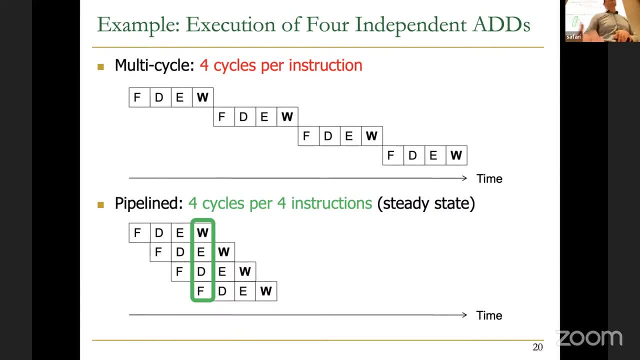 Because the throughput of instruction processing has improved, as we can see. Okay, so basically here you're completing one instruction per every cycle, every one cycle, which, as we just discussed, Whereas here previously we were completing one instruction every four cycles. 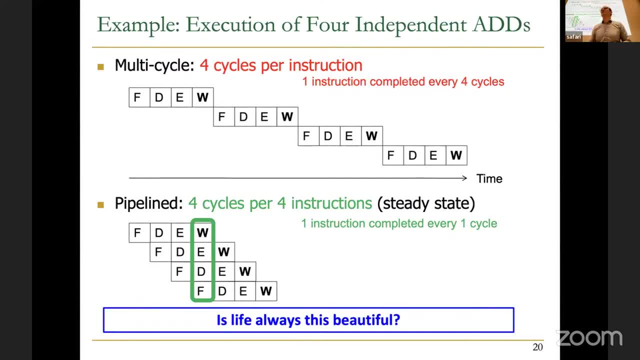 Okay, that sounds good. Of course, life is not always this beautiful right, So there are a bunch of assumptions that this makes. You have four independent adds. Pipeline is structured this way, So we're going to look at issues with pipelining. 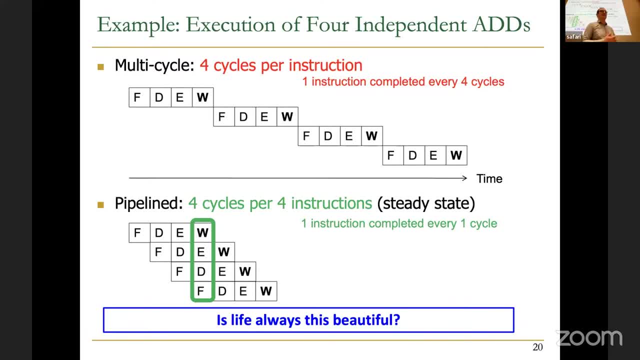 Can you always keep the pipeline full, for example? Can you always be in the steady state? Is that easy? What happens with branch instructions? What happens with control flow instructions? That's going to cause a lot of headaches for us, But that's going to also make us very creative in terms of how we handle things in the pipeline. 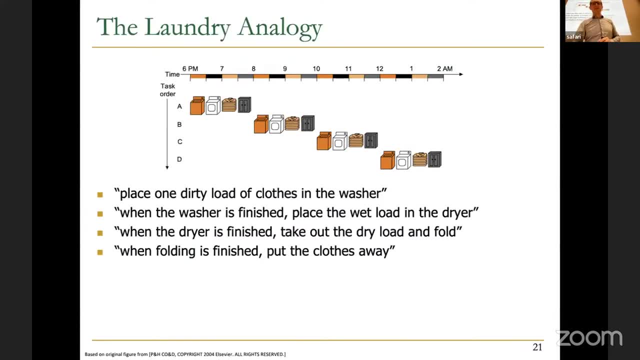 Make sense. Okay, so let me give you an analogy. How many people do laundry here? How many people do not do laundry? I want the hand because I want to learn from you how not to do laundry, but I don't see any hands. 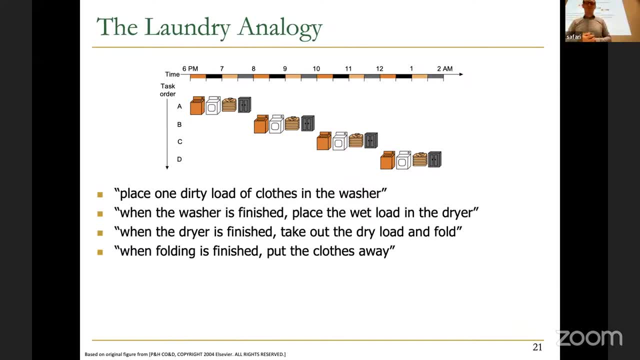 So that's good. Well, I don't know if it's good, I could have learned. I missed that opportunity. But basically, if you look at, this is another book- the Patterson and Hennessey book- that develops this analogy, which I like. 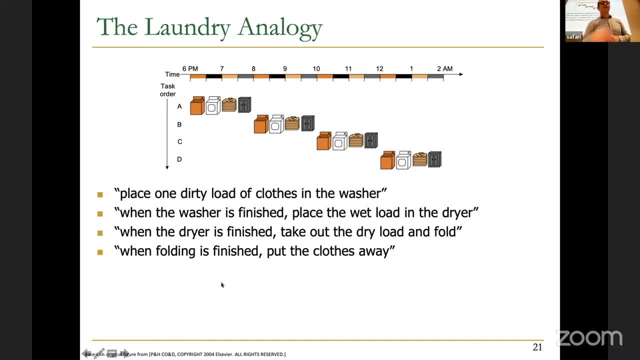 Essentially, there are four distinct stages of processing of a laundry load. You place one dirty load of clothes in the washer and then, when the washer is finished, you place the wet load in the dryer and then, when the dryer is finished, take out the dry load and fold somewhere. 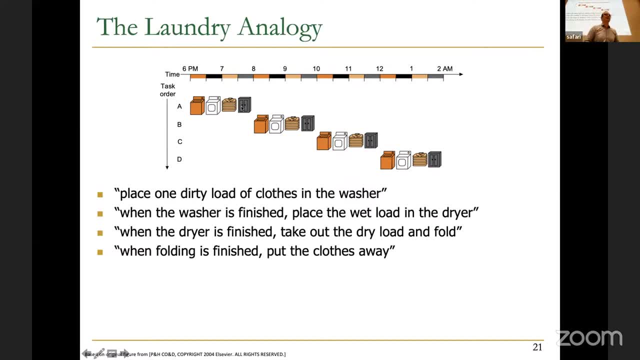 And then, when folding is finished, put the clothes away in the wardrobe, And, assuming that each of them takes 30 minutes, each load takes two hours, as you can see, And if you have four loads, this is what you would do. 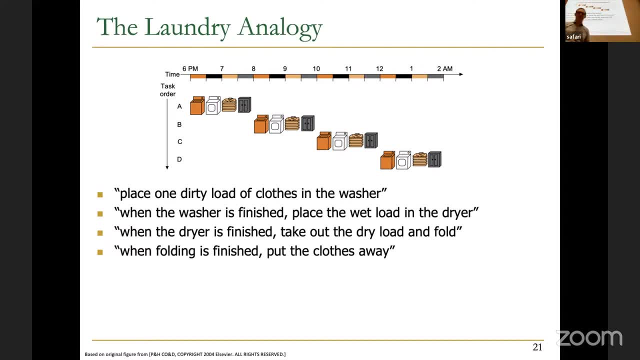 You would take eight hours for the four loads. Well, that's what a multi-cycle laundry machine does, But let's take a look at that before. So the steps to do that, The steps to do a load, are sequentially dependent, So you cannot start the dryer before you wash the clothes. 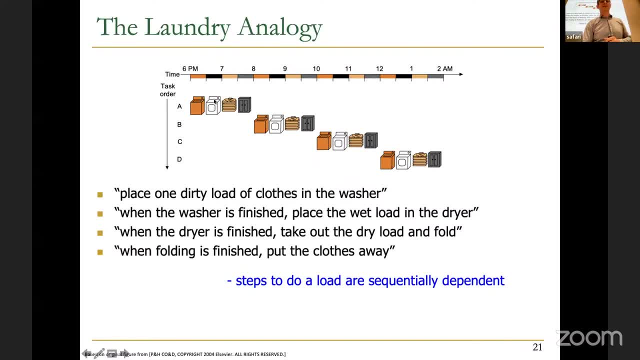 I guess you could, but there would be no point, And you cannot fold the things before you dry them, And then you cannot put the clothes away before you fold them, or at least gather them somewhere if you don't like folding. So there's no dependence between different loads. 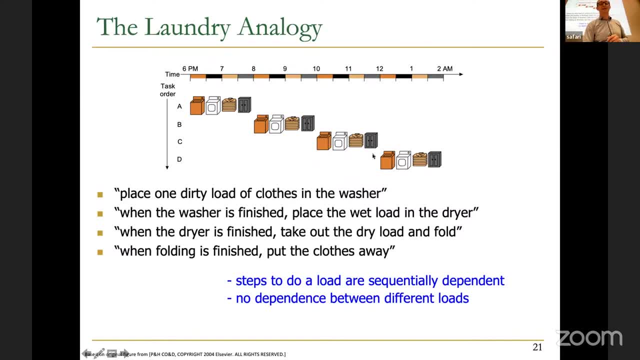 This is like our ads earlier. This load has nothing to do with this load right, And different steps do not require the same. So you can take a load, pick it up and then you can fold it over again. So it's very similar to our pipeline. 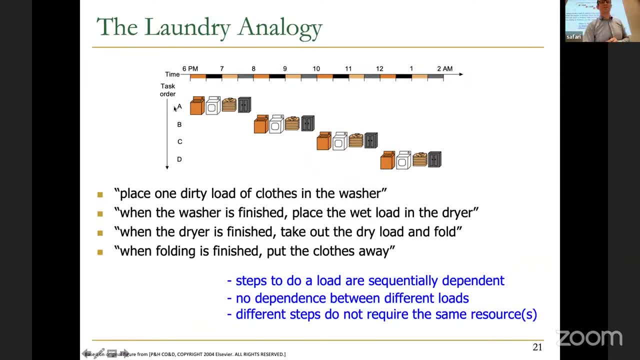 So it's very similar to the pipeline basically. We've got plenty of resources. That's good. Basically, washer, dryer, this folding, whatever components and the wardrobe are distinct, They don't share resources, So it's very similar to our pipeline basically. 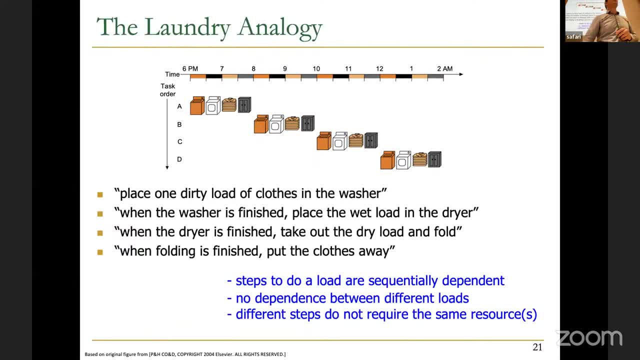 Yes, We're going to get back to this. I'm giving you an analogy. Okay, We're going to get back to it. The instructions are going to be slightly different. Okay, So how do we pipeline multiple loads of laundry? So the first step is to set up your own load, right? 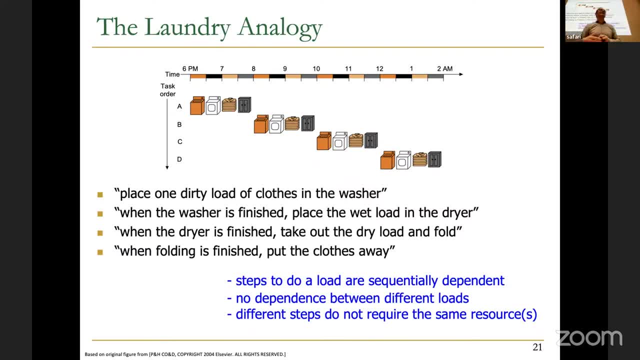 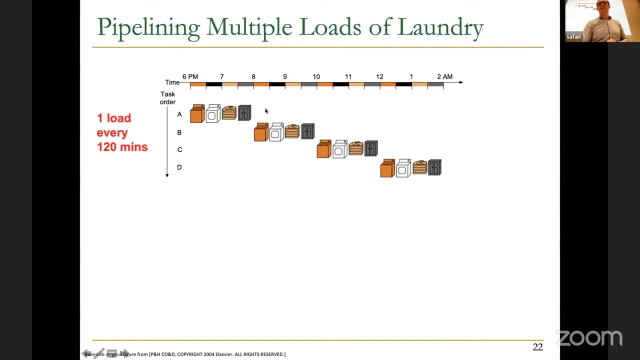 And then you have to decide what kind of load you're going to load, And then you have to decide what you're going to load. instructions are going to be slightly different, okay, so how do we pipeline multiple loads of laundry? as i said this here, you finish one load every 120 minutes, right, if you do it sequentially. 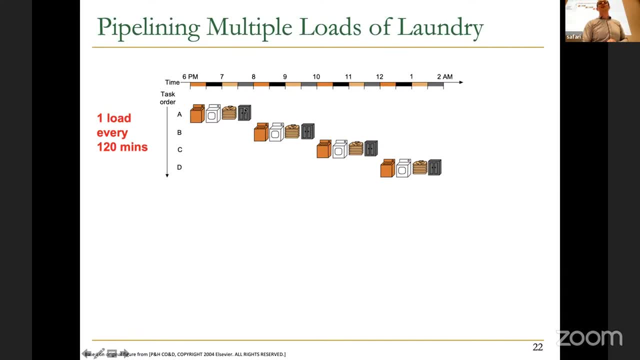 like this and you're not exploiting the concurrency. for example, while this instruction or load is using the dryer, the washer is idle and you're not exploiting that. if you pipeline the processing, it will look more like this: basically, right once one load finishes with the washer, you actually input or load the washing machine with the second load right once the first load. 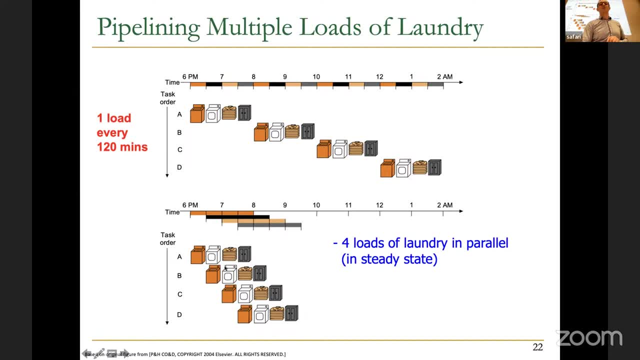 finishes with the dryer. you low you, you place the second load into the dryer, and so on. so this is very similar. this way, in the steady state, you can do four loads of laundry, as you can see, which is good, and you can finish one load every 30 minutes. 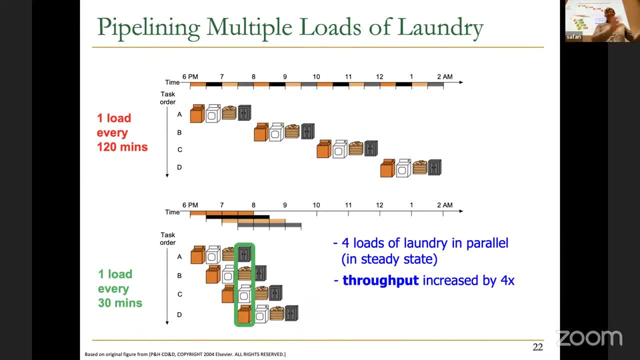 which means that your throughput just increased by 4x, very similar to the add operations that you've seen, but latency for a load is the same, so that's interesting. yeah, so that's the difference between throughput and latency, but the latency of the overall four loads is much shorter, as you can. 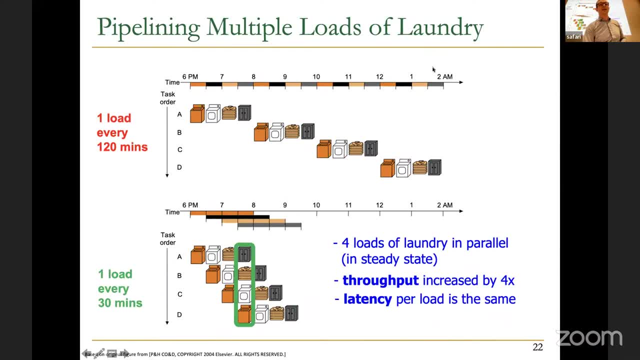 see right, it finishes uh over here, whereas this one finishes at 2 am. so instead of waiting until 2 am for four loads, you're waiting until 9: 30 pm. okay, and there are no additional resources. so in this particular case, uh, you don't need any additional resources to do the pipelining, so that's going to be a little bit. 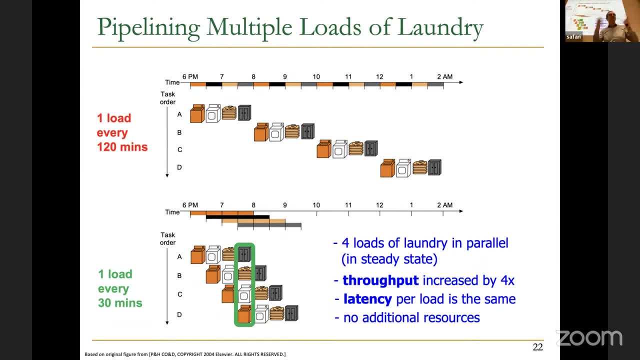 different, uh, in instruction processing, as you kind of guessed earlier. okay, so now, uh, if you've done laundry, uh, what's the worst stage over here? have you ever, if you, if you've done laundry in real life- which machine takes the longest or which stage usually takes the longest? 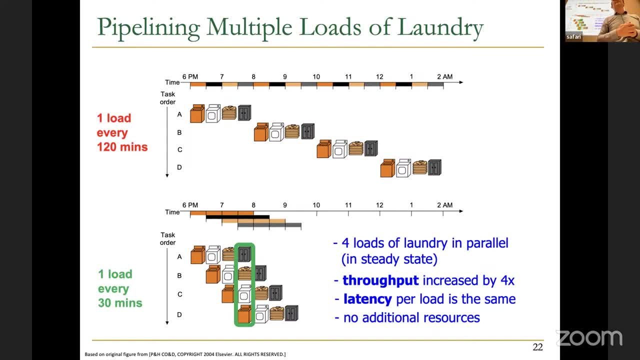 in your opinion anybody? i always have a problem with the dryer. damn, dryer never is fast, basically, and if you want to be really more energy efficient, it becomes even slower. this dryer- you may have seen that, but basically the real life may look like this: where the dryer 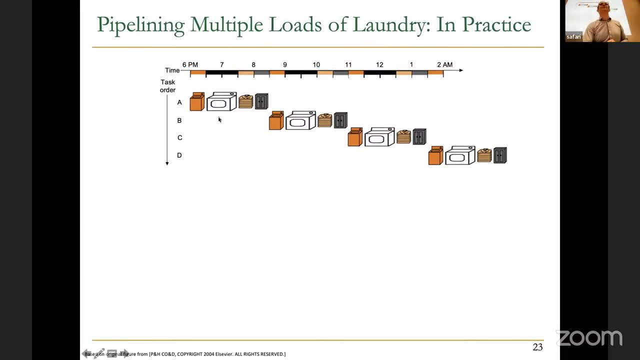 takes one hour as opposed to 30 minutes right now. if your dryer takes one hour as opposed to 30 minutes, and if you are sequentially doing these loads now, you have one load every 150 minutes. okay, so if you want to be more energy efficient, you can increase this by 30 minutes. uh well, yeah, uh well. 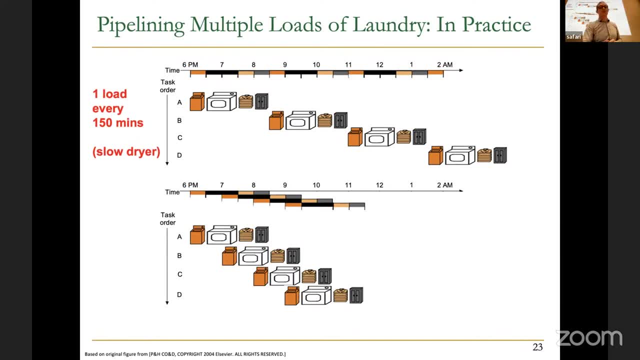 throughput. you reduce the throughput by a little bit, but this affects your pipeline uh also. basically, if you pipeline things, you cannot start drying the second load after the uh until the drying of the first load finishes. so this becomes your bottleneck. this dryer becomes your bottleneck, as you can see. 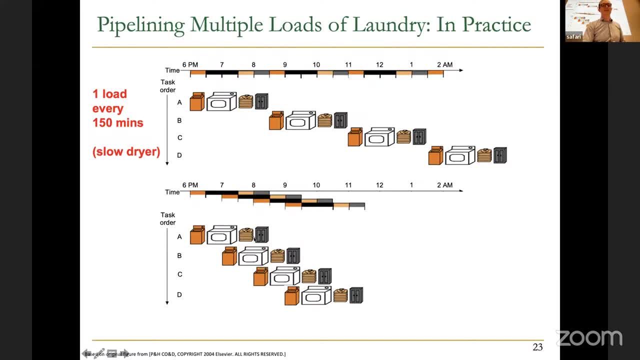 so you kind of have some empty time, if you will, that you don't use. so you can see that you're finishing one load every one hour, every 60 minutes, because of the slow dryer, right? so the slowest step, the dryer decides the throughput, and that's true for uh existing pipelines, uh instruction pipelines as well. so how do you solve? 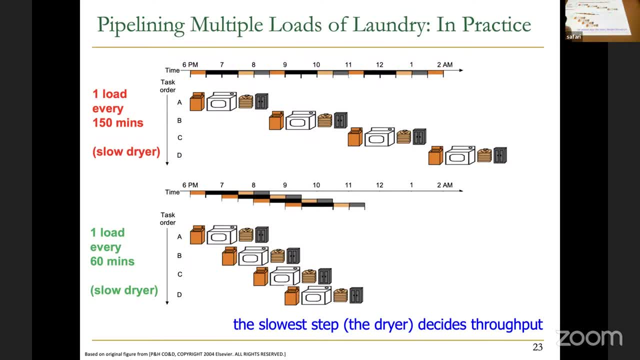 this problem. what do you do? buy a better dryer, much faster. that's much faster and that finishes in 30 uh minutes. that's one way of solving the problem. you pay cost. it's expensive, of course. right, yes, having two dryers would solve the problem also. basically, the first instruction would use the 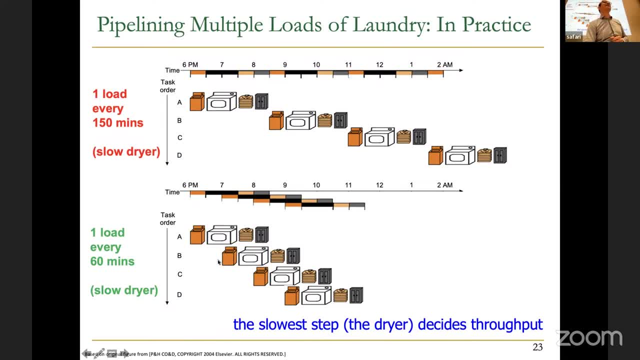 dryer a. the second instruction would use dryer b and it can now start over here. that's also costly, but maybe more it may be easier than actually buying a much faster driver, because faster dryer may be technologically not feasible, let's say potentially. so basically you can restore the 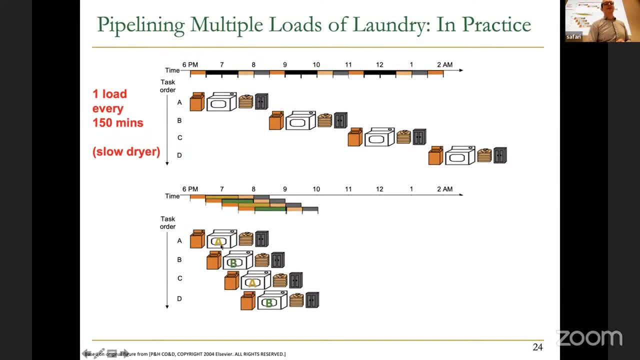 throughput by having dryer a and dryer b and alternating consecutive instructions between dryer and dryer b. that way you don't need to wait for one dryer to finish. now your throughput is restored to what we had: one load every 30 minutes with two slow dryers. so this is an example of the trade-off between performance and cost. right, you add more costs. 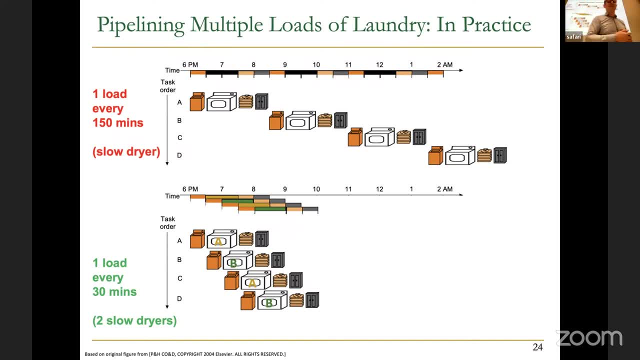 so that you have the same throughput in your pipeline as if you had a fast dryer. make sense, and this is a very common technique. that's done, okay, i already said this, so, okay, just to give you an idea. uh, clearly, computer scientists are not the first one to do this, i think. 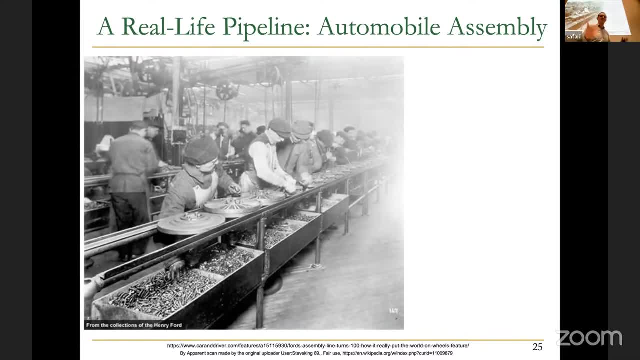 computer engineering and computer science can do a lot more by figuring out what's going on in the real world also. but this is an assembly line. do people know what this is? these things are? well, these things that are being produced in the assembly line of workers. this is the ford motor. 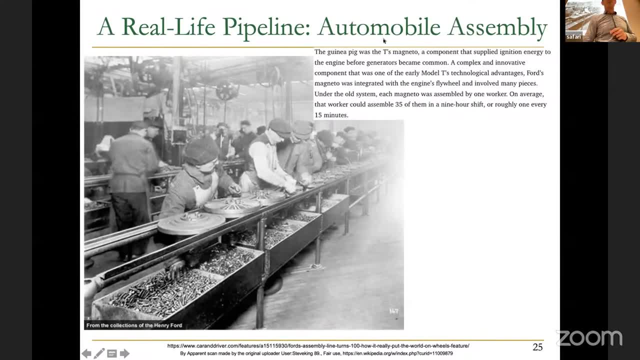 company. it's actually, uh, an important component at the time. it's called magneto. have you, have you heard of magneto in some other context? x-men, potentially okay, some people have okay, maybe. maybe x-men is too old, maybe i'm too old for you guys, i don't know. i don't know the. 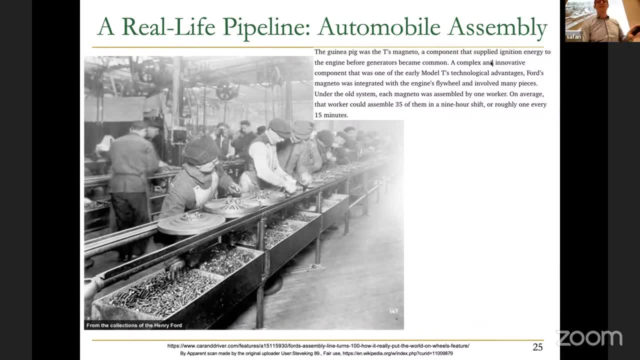 latest interesting thing. but basically this was a complex and innovative component in ford's early model t's advantages and uh, basically it's involved this sort of processing and on average, uh, they say the worker, uh, it was assembled by one worker before and it could assemble 30, this worker. 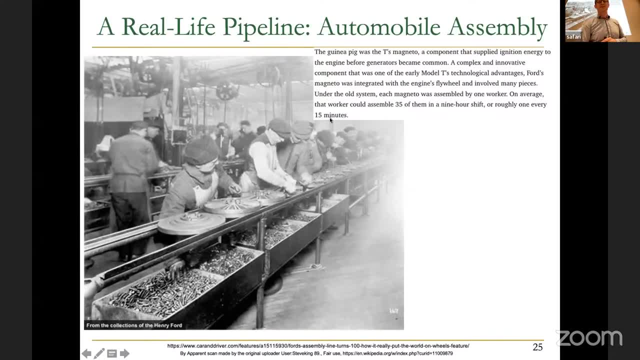 could assemble 35 of them in a time hour shift, or roughly one every 15 minutes, and then for transition to this assembly line processing in 1913, as you can see, and uh, this is the assembly line for the magneto itself and they basically have some results. these are wikipedia. they'll blame wikipedia for. 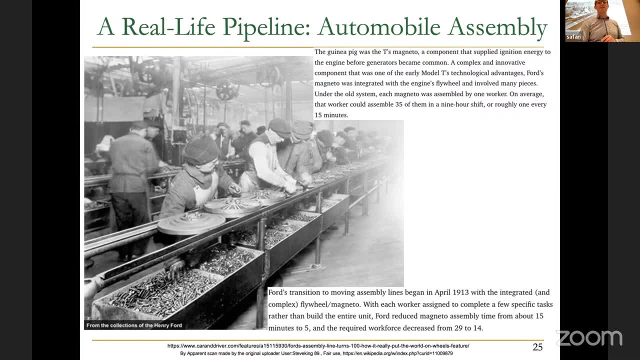 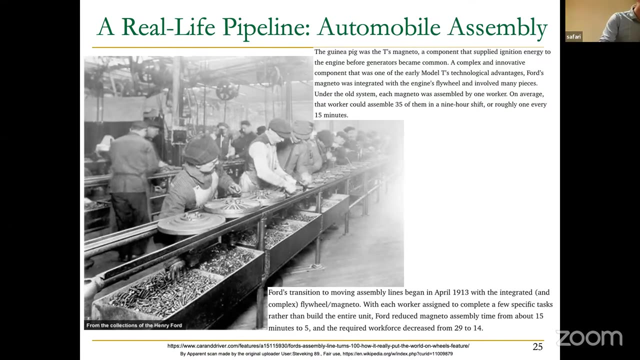 wrong information. if it's wrong information, you can see that they reduce the magneto assembly time significantly. vx, if you will. that's the throughput, basically. i would say: basically, what's going on here? something got removed. how did this happen? oh, okay, it's just this connection, i guess. 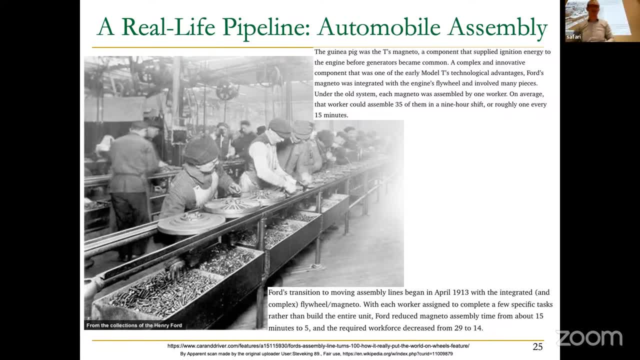 this says low battery, so i need some charger here. it's actually very low battery, otherwise it'll turn off. is the charger not connected? okay, maybe that's. that's. that was the issue. you think it's sold okay? okay, uh, low battery again. okay, basically it's. 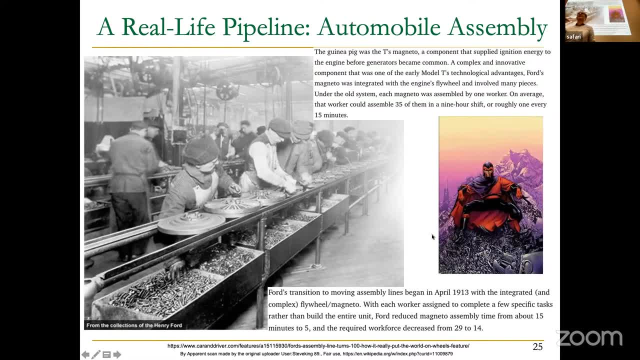 you can see that. uh, yeah, the assembly line improved and this is the magneto. this is the original magneto from the x-men cartoons. you can see the similarity? right? these guys were definitely inspired by ford's magneto over here. okay, so now you know where people get inspired. 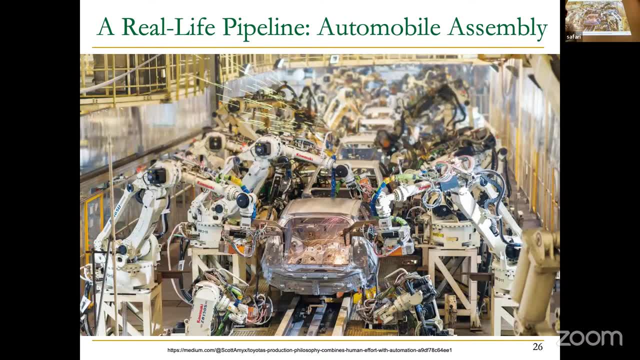 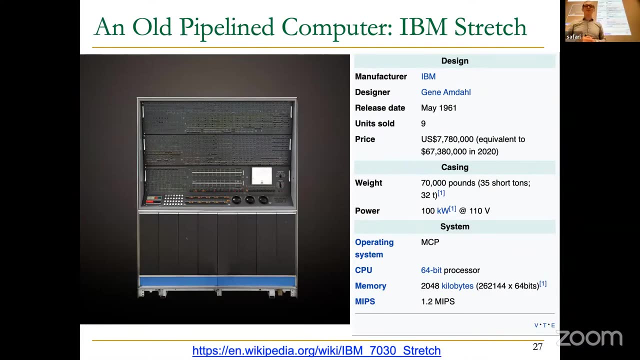 from, and this is a more modern assembly line of robots, uh, assembling cars, so cars go through. similar. this is, uh, yeah, similar, uh, assembly lines, and this is actually one of the first pipeline computers: ibm stretch. you can see that the designer is gene amdahl, in 1960s, and you can also see the price at the time, so you could buy this thing, which is much. 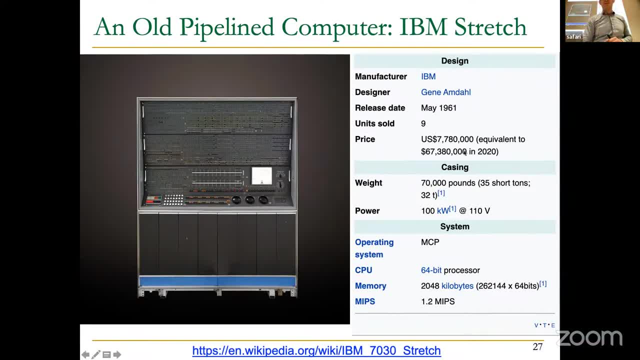 less powerful than what you have in your cell phone for 67 million dollars in 2020.. how many of you are willing to pay that? well, yeah, thank moore's law for not paying that. let's say, okay, but this is fun. of course you can take a look at it, but this is a real. 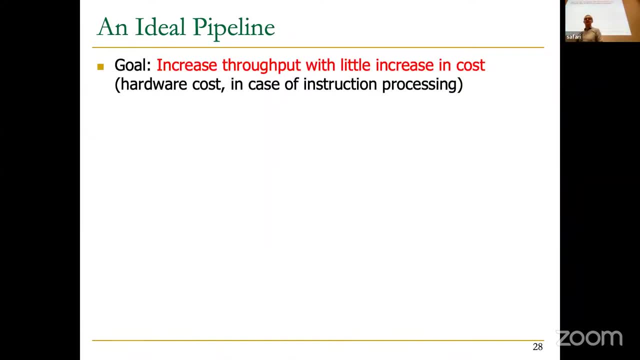 pipeline computer. so the principles of pipelining were developed in 1950s, uh, maybe even earlier. so basically the goal we have in pipelining in an ideal pipeline is to increase throughput with little increasing cost, ideally no cost, right, uh, hardware cost in case of instruction processing. 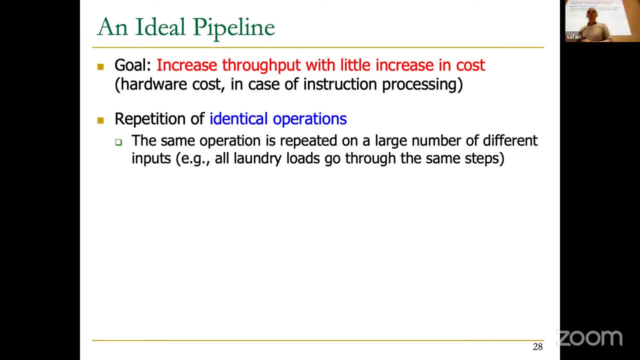 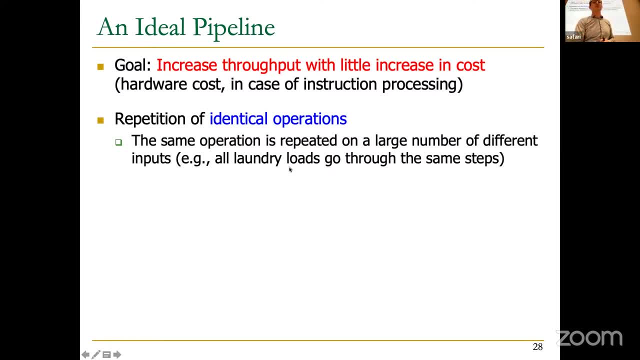 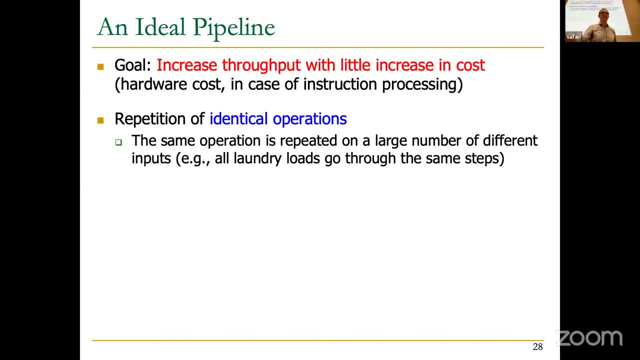 it's going to be a bit different than instructions, because instructions are heterogeneous, they're different from each other and we're going to analyze the instruction processing pipeline, that and you want to repeat independent operations in an ideal pipeline, ideal assembly line, no dependencies between repeated operations. the first load is not. 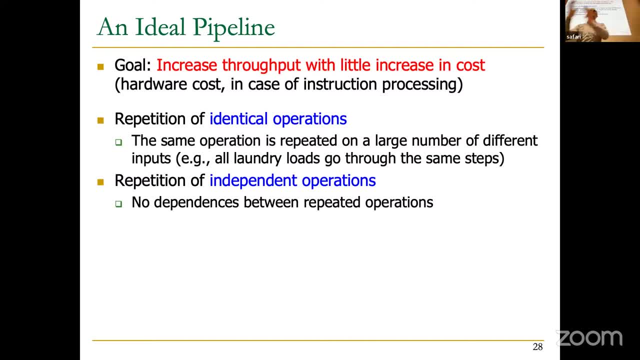 not. the second load is not dependent on the first. the second car is not dependent on the first. that's absolutely true in an assembly line that produces cars or the magneto. there is no dependence right, whereas that's not true in case of instructions, one of the later instructions. 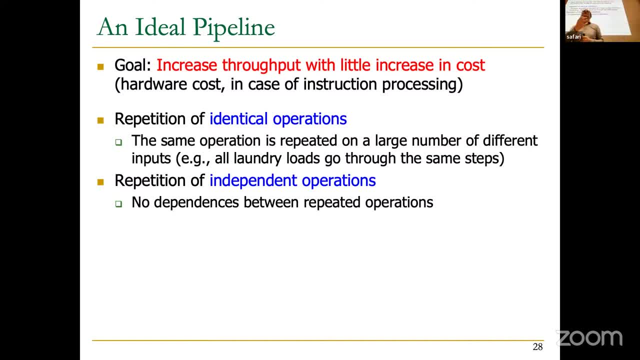 is going to be dependent on the previous instruction because it's going to source a register value that's written by a previous instruction. so it's going to make our lives difficult. and finally, in an ideal pipeline, you want to be able to uniformly partition the sub operations. what does this mean? you want to divide the processing of, let's say, a car. 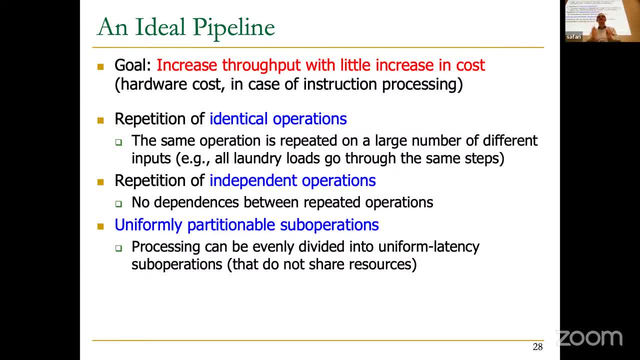 what a car goes through evenly into uniform latency sub operations, such that you have equal length pipeline stages that do not share resources. and you can do that again in a factory, for example. every car goes to the same stage. you basically partition the operations such that each worker consumes the same amount of time and if you actually need 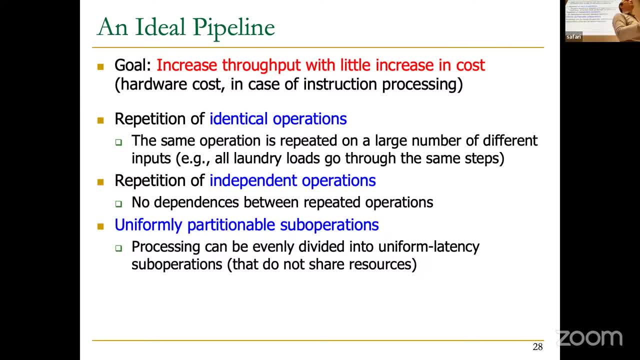 more time, then you divide it. divide the amount of things you need to do or you increase the number of workers, just like we increase the number of dryers. right, if one stage takes longer, you increase the number of workers. so basically, this is going to be harder in case of hardware. 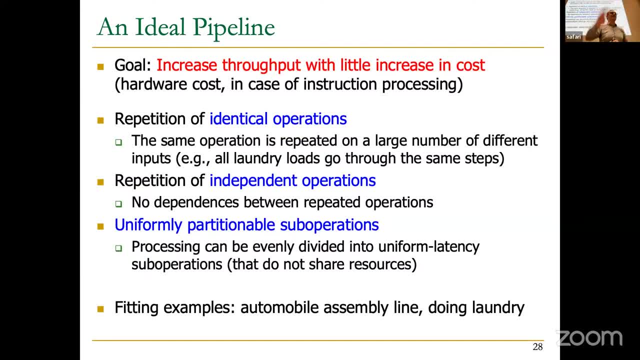 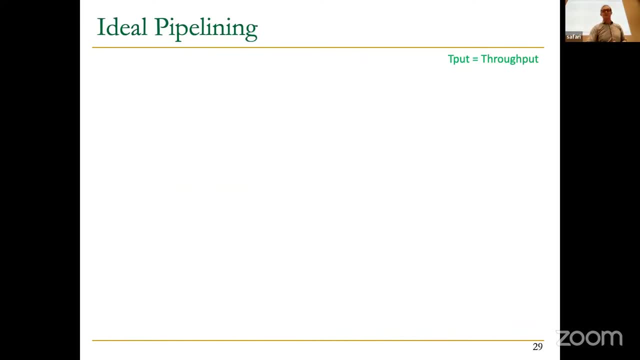 design, as we will see, because of the critical paths and combination logic and sequential logic. so basically, automobile assembly line and doing laundry are perfect examples of ideal pipelines. but instruction processing cycle, as i just said, is not going to be perfectly ideal. so let's take a look at this ideal pipeline. so i'm going to abbreviate throughput with tput, so this is: 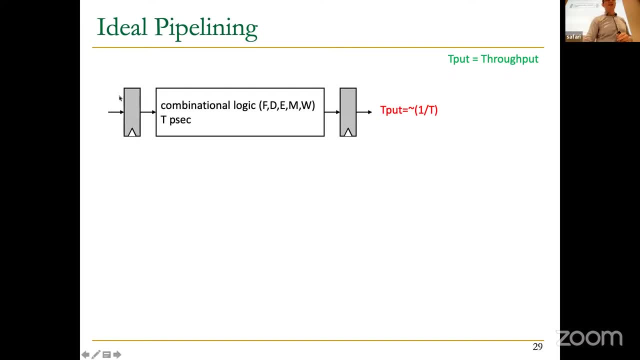 a non-pipeline uh processing engine. let's say you have combination logic that does all of the operations that are needed for an instruction. let's say it takes t, picoseconds and the throughput is approximately one over t because there's some register overheads, a sequential sequencing. 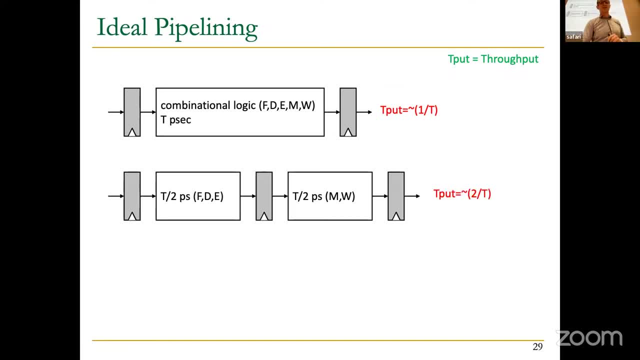 overhead that i'm ignoring over here, clearly. so one over t. let's assume that now, if you divide into two stages, uh, you should really equally divide the two stages. so this should take really two t over two picoseconds and this should take t over two. so your throughput should be: 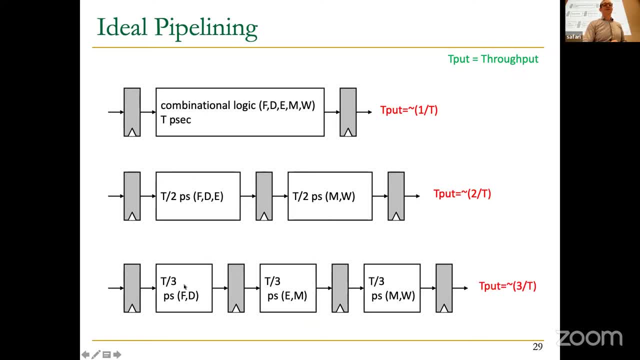 doubled, and then, if you divide into three, you should really divide into equal stages, and then your throughput should be tripled. but again, this may not be easy to do, because how do you ensure that you perfectly divide the work into three different combination, logic, uh, sequences? let's say: 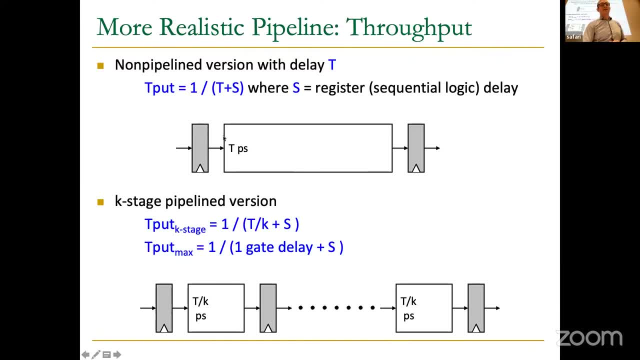 okay. so let's take a look at the more realistic pipeline then. so you have a non-pipeline version with some delay. t throughput is really one divided by t plus s and you have a sequential logic delay over here. and assuming that you can again perfectly divide the 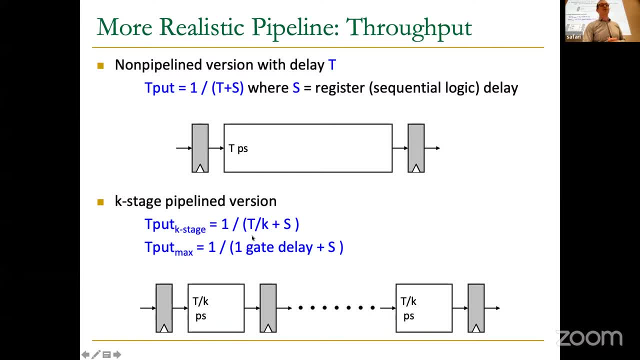 stages. uh, this t picoseconds of work into k stages. the throughput of the k stage pipeline will be one divided by t, divided by k plus s, as you can see, because there is a sequencing overhead and the maximum throughput is basically how, how small can you make this t divided by k? 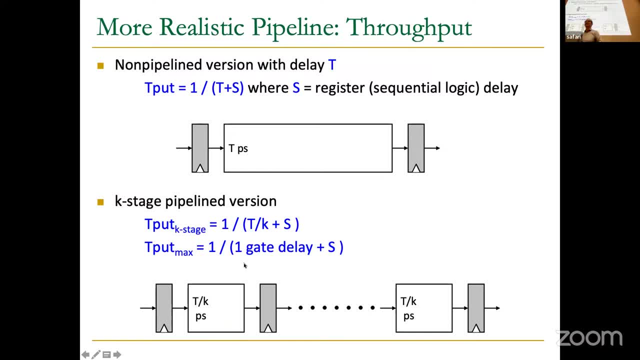 so let's assume that it could be one gate delay, right, yeah, one gate, so you can actually maximize your throughput by minimizing the uh amount of logic that you put in each stage, but your your throughput at that point. maybe this gate delay is small, but this s may be large. 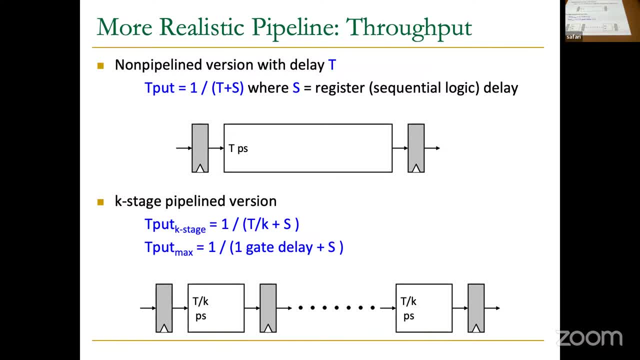 so your sequential logic, delay in the in the in the limit, will dominate, uh, this latency over here. as a result, your throughput will be limited by the sequencing overhead. so it's good to know this. basically, your registers are again your limiting factor over here, okay. so basically, register delay reduces throughput because of the sequencing overhead between stages you pay. 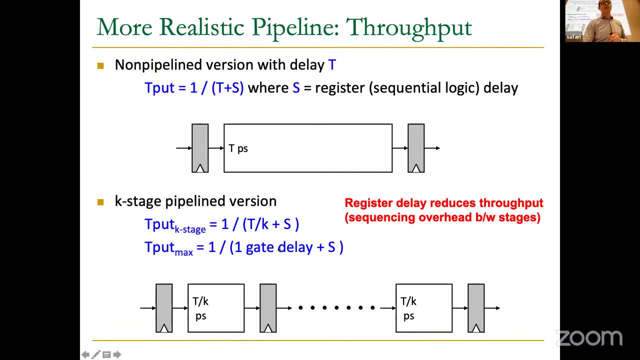 s uh every, at every stage, and that's why your throughput is limited. and again, this picture, as i mentioned, assumes perfect division of work between stages t over k, but that may not be perfect, as we will see in an example very soon. actually it's very difficult to actually perfectly 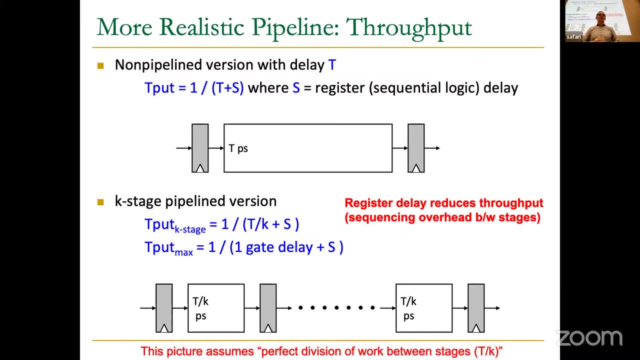 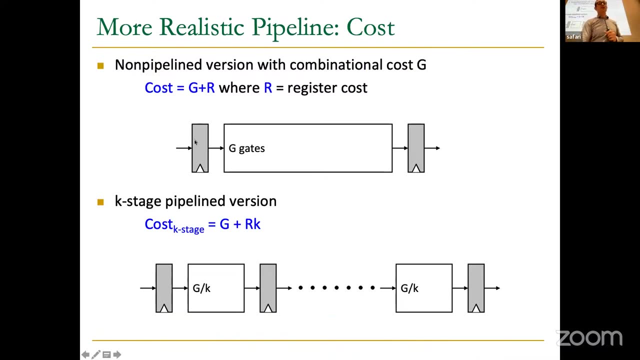 divide this t picoseconds into equal stages. if you don't do equal stages now, the longer stage you remember the dryer determines your clock cycle time as well as your throughput in the end. okay, so let's take a look at the cost. so this was throughput. let's take a look at cost. 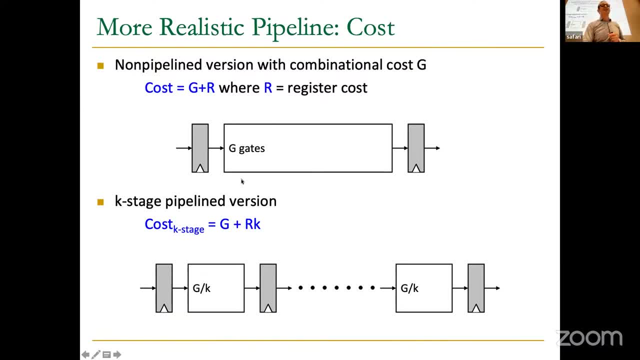 so this is a non-pipeline version with some combinational cost g, g gates, and then there's some register cost r. if you have a k-stage pipeline version, if you perfectly divide the g gates across k stages, this doesn't change. not very realistic. but this is, we're assuming, perfect. but 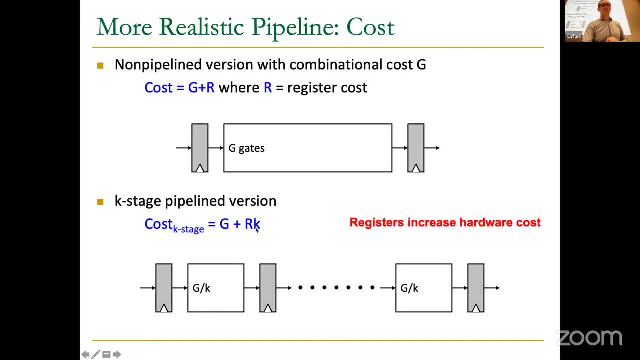 unfortunately, your register overhead multiplies by k, so you can see that registers actually increase hardware cost. that's the trade-off we're going to make again. we're going to increase hardware cost registers even if we perfectly assume that the work can be divided across k stages like this again this: 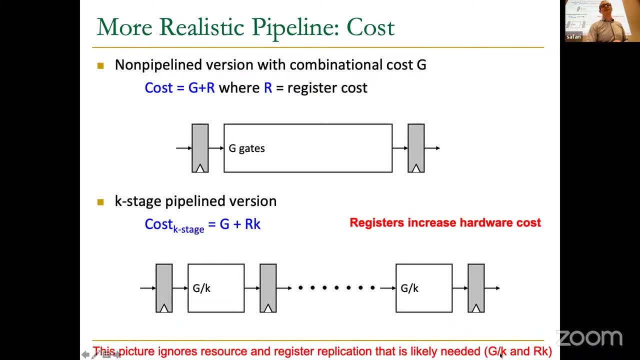 picture also ignores the resource and register application that's likely needed. so basically, we assume that this is g over k, but it may not be actually g over k. it may be g divided by something larger than k. right, because some things you may need to replicate across the stages. 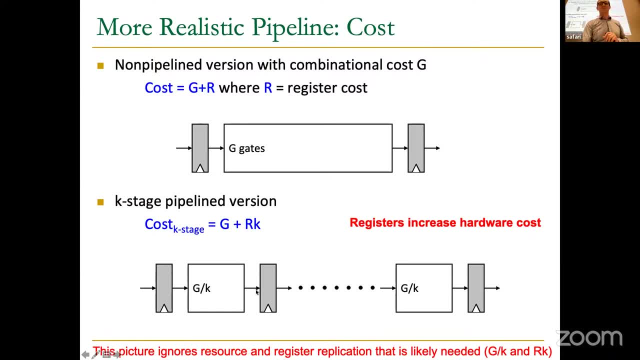 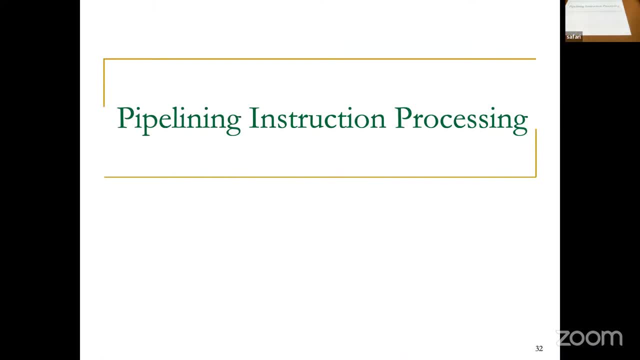 okay, and some registers you may actually need to replicate, as we will see soon. does this make sense, okay? so let's take a look at now, with this, let's say, high level theory, let's take a look at, uh, pipelining, instruction processing. so remember the instruction processing cycle. this is a 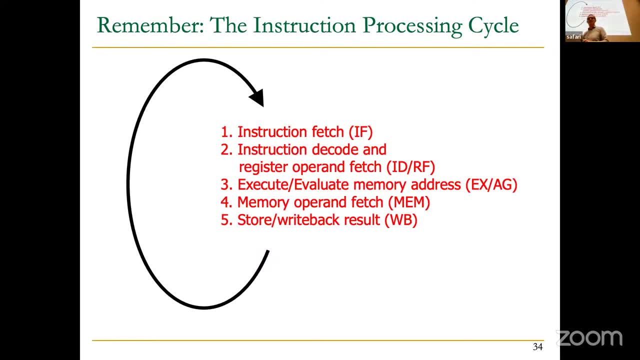 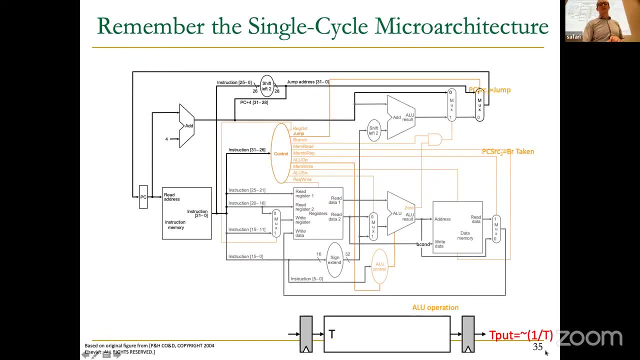 different way of looking at it and this is what we kind of agreed on in the last few lectures. let's look at it in a five stage manner, and this is a single cycle microarchitecture where the throughput is determined by the single cycle microarchitecture where the throughput is determined by the 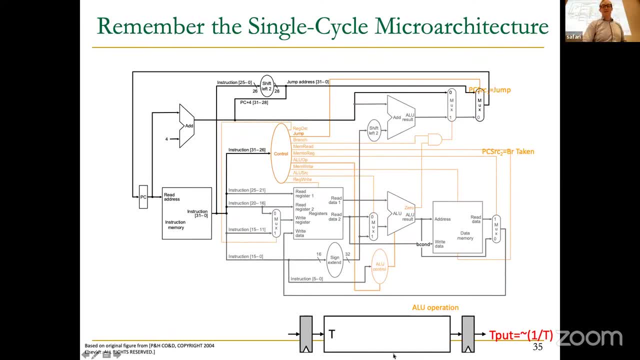 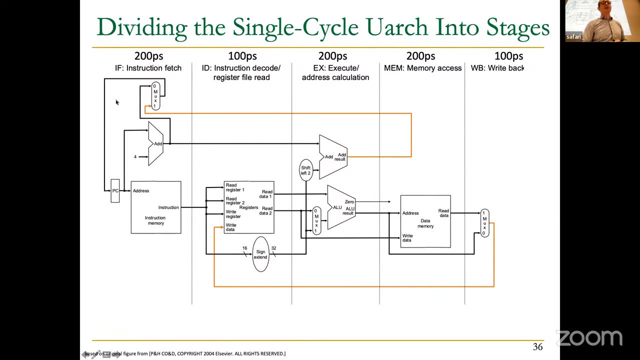 t, which is the longest instruction to process. let's say, let's divide the single cycle microarchitecture into stages of pipeline. let's say instruction fetch is one pipeline stage and instruction decode is another, execution and access calculation another and memory access another, and then write back is another. and i just gave you some numbers over here because, yeah, your book. 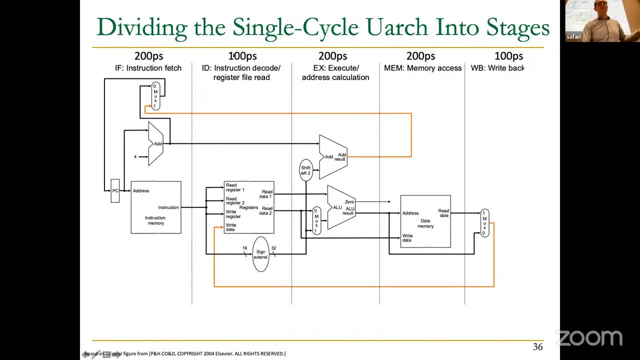 made up these numbers, or i made up these numbers. fine, uh, but i mean it's not unreasonable. this is just to make a point. so basically, if you look at this, there are five stages in the pipeline. i didn't put the pipeline registers. we're going to put them soon- but basically you're here. it's 100 picoseconds. 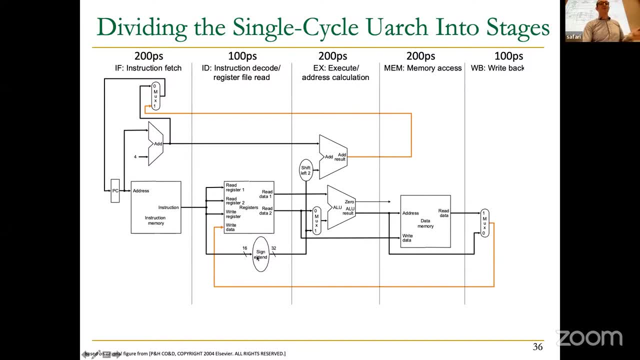 here it's 200 picoseconds, right? you didn't perfectly divide things. why maybe we couldn't right? because the memory may take 200 picoseconds to access and this is the critical path. over here and here you don't have enough in the critical path and if you actually try to, 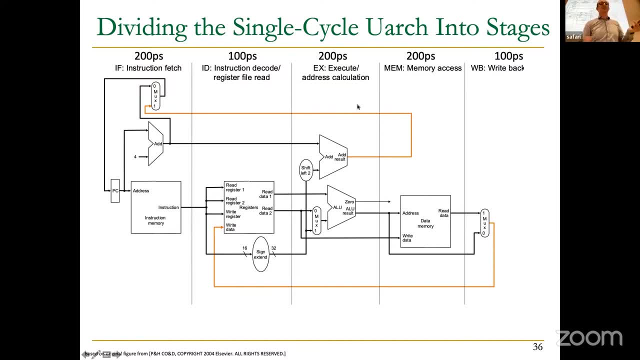 divide it in some other way, this will also become shorter, so maybe balancing this pipeline is not very easy. it's called pipeline balancing- balancing the different stages of pipeline such that they're equal, and essentially it's not easy and it's not a complicated- uh instruction set architecture yet. so let's take a look at what happens over here. so you'll need to. 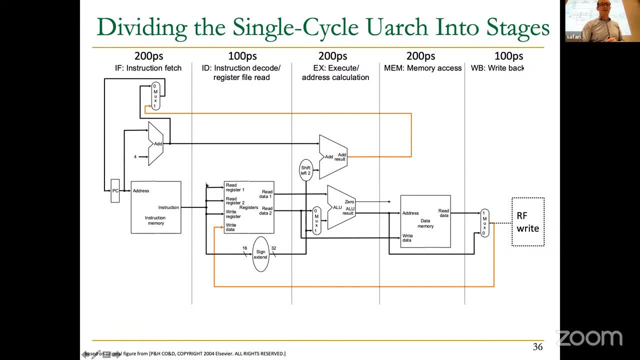 basically enable writing. we're going to talk about that, but there needs to be a way of actually doing that writing. then we're going to ignore some of the back loops, because these are a bit dangerous. how do you handle these things that go from one stage to the resources of another stage? because 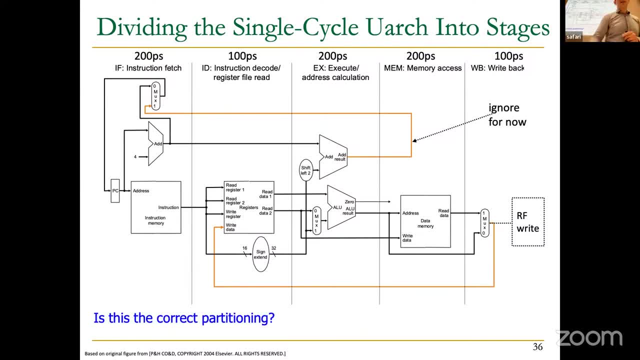 we need to be very careful with how we write these things in order to get the right, of course. so why should if we have too many collections? we have, so we're not able to already look at this a little bit, and there are a lot of, a very few expansions in the pipeline. 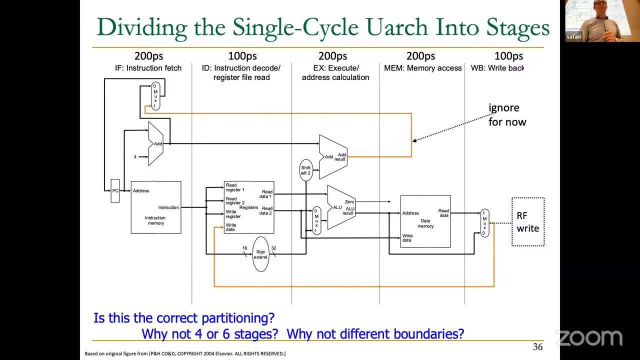 but it's not just the way it should be. it can be threatening and they could cause problems, as we will see. okay, so basically, there are questions to ask over here: is this the correct partitioning? maybe, certainly it's not a perfect partitioning right. can there be a perfect partitioning? it's. 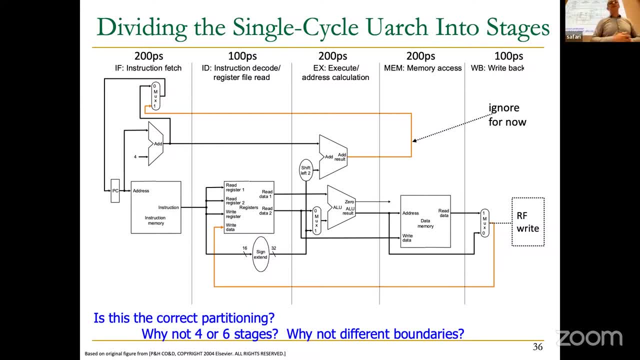 not clear. so why not, for example, four or six stages? why not different boundaries? to run into some other issues, as we will see. okay, so let's take a look at the throughput in this pipeline. even in the simple five stage pipeline, normally, if it's perfect pipelining, we would 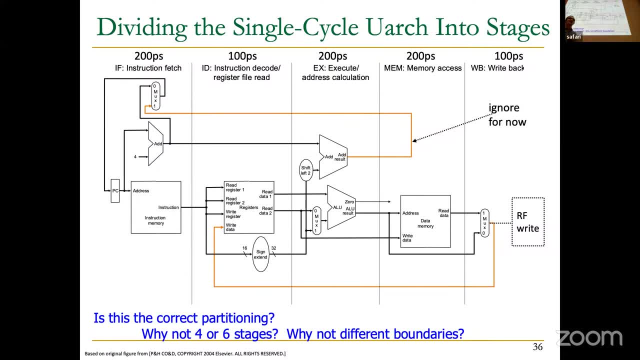 assume throughput to increase by 5x, right, so we should finish before we were finishing. let's say, one instruction, uh, every five, uh clock cycles, uh, now we should finish one instruction every clock cycle, right? so let's take a look at this. so this is the. 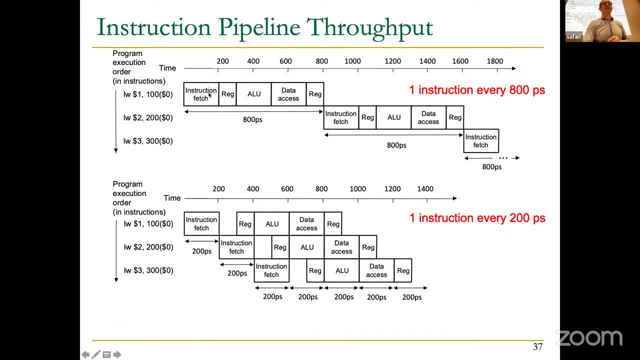 t that i showed you earlier. assume that it's a single cycle machine and it could be multi-cycle also, depending on how you look at it. but basically we're finishing one instruction every 800 picoseconds and we're doing the first load instruction and then the second load instruction, the next load instruction, and they're independent as you can. 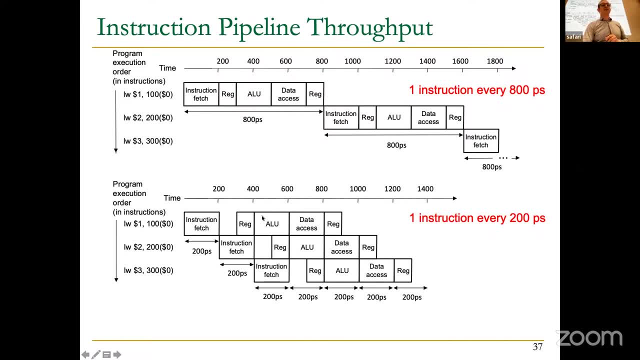 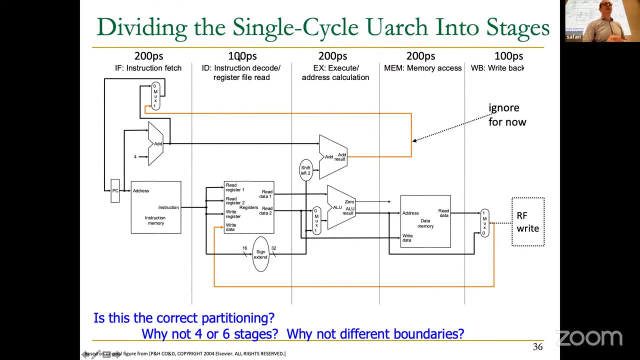 see over here. so one instruction every 800 picoseconds in the pipeline we design in this picture. let's take a look at how many instructions we're finishing per picosecond, so you can see that every stage needs to take 200 picoseconds, even though this is 100 picoseconds. we cannot. we have. 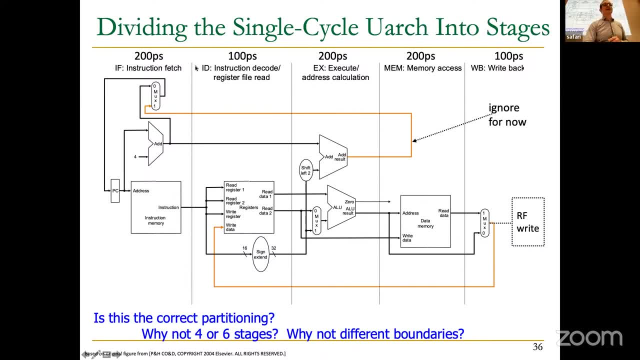 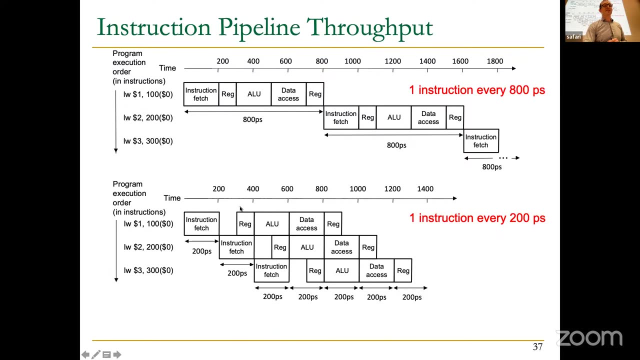 to have a single clock. you cannot uh so that you can synchronize. uh, so this takes 200 picoseconds. this should also take 200 picoseconds. this is taking 200 picoseconds, and the last one should also take 200 picoseconds. basically, patches take in 200 picoseconds. uh, the register read and decode. 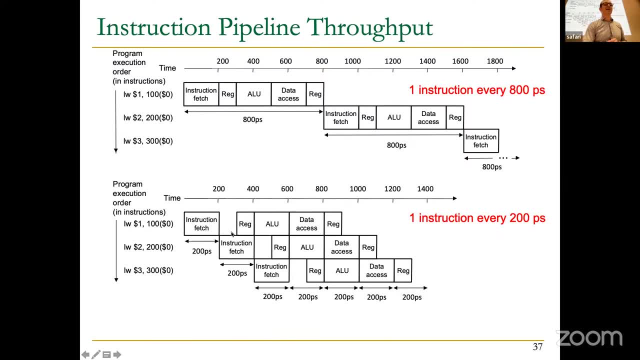 so this is when you can actually respond to the 귓, and then when you see that you push this button one time, it will take 100 picoseconds, but you're going to waste half of that clock cycle because your clock cycle needs to be larger. right, your clock cycle is determined by the worst. 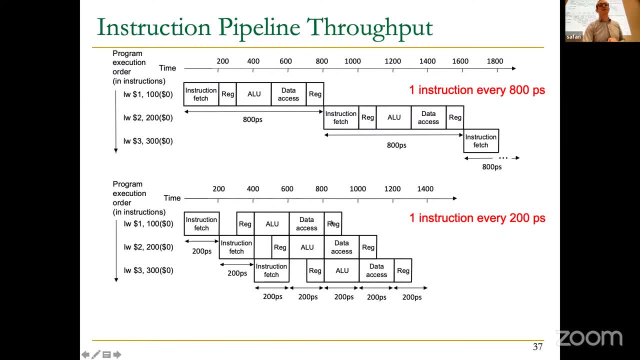 case stage, remember the dryer kind of- and then you can see that the register right is also taking 200 picoseconds. but even though it doesn't need 200 picoseconds make sense. so if you look at the throughput over here, you're really finishing one instruction every 200 picoseconds. 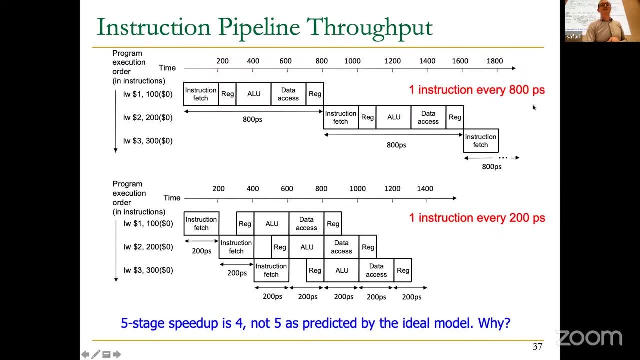 five stages in the pipeline here, But the speedup is 4x. You went from 800 to 200, as opposed to 5x. Why? Because we didn't balance our pipeline well. If you balance your pipeline well, each stage should have taken 160 picoseconds, But, sorry, your memory takes 200 picoseconds. 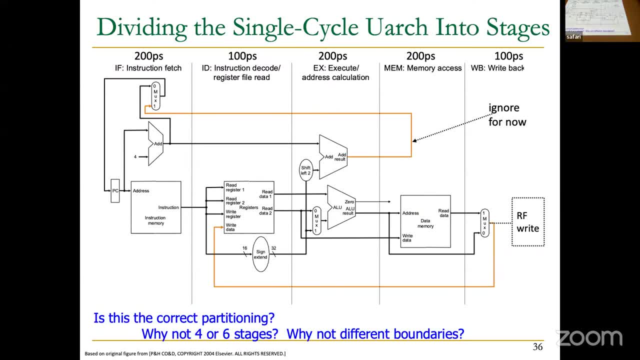 What are you going to do? It's very hard to pipeline internally in the memory. You can actually try to do that, but now you actually need to go inside the memory and add some pipeline registers, as we will see, But it's not going to happen easily. 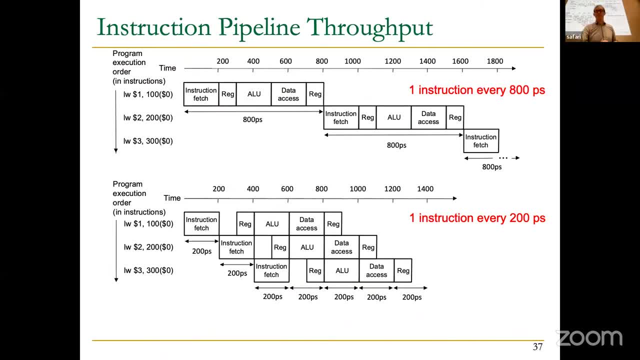 So this is one of the fundamental issues with pipelining: Balancing the pipeline such that you equally divide the work that would otherwise be done without overhead, like 800 picoseconds over here, is difficult. As a result, you lose throughput immediately, And the main reason is: 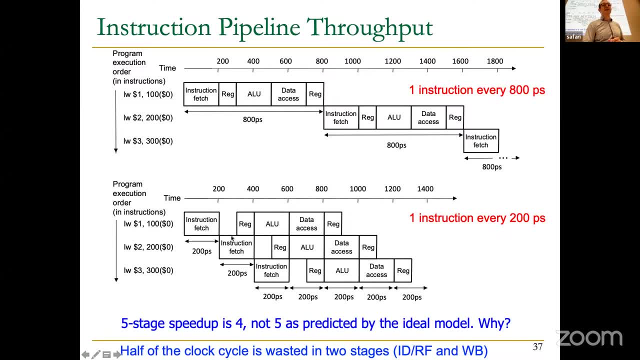 you couldn't divide the work And, as a result, half of the clock cycle is really wasted in two of these stages: This stage and then this stage. Basically, whenever you read registers, you're wasting the clock cycle because that's fast, But your clock cycle is determined by the slowest. 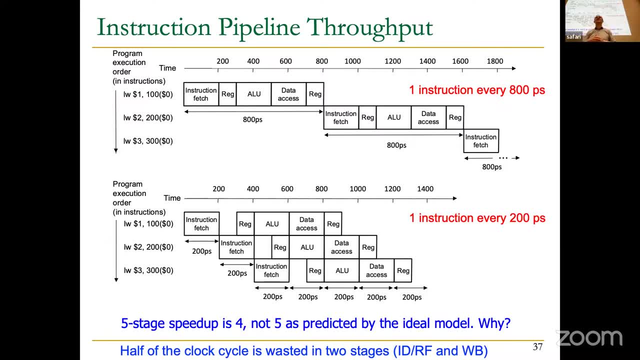 stage in the pipeline. Does this make sense? So a lot of the timing issues we've discussed, now you're actually seeing how they come into play in real life. So reducing the clock cycle time and balancing the stages could be one option to actually restore the throughput. 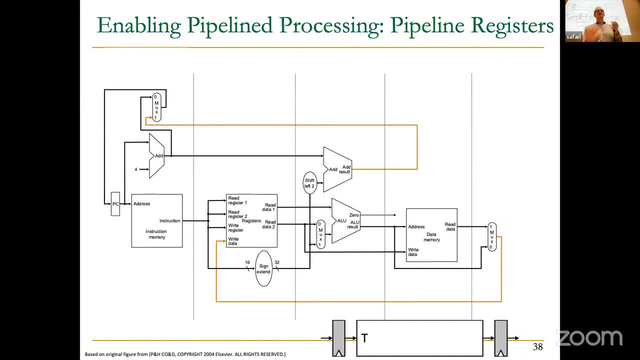 but it's not easy. So, basically, how do we enable pipeline processing? I mentioned these pipeline registers. So this is our single cycle processor, reduced if you will, And you can see that it's only single cycle, as you can see, and we have t amount of work. Basically, we're going to divide. 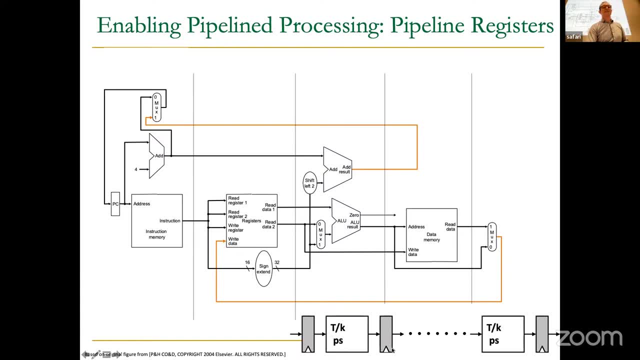 this into some number of k stages, such that hopefully each of the stages will take close to t over k. So to be able to do that, to be able to make sure that the processing that happens in one, one stage, for one instruction, doesn't interfere with the processing that happens in another stage, 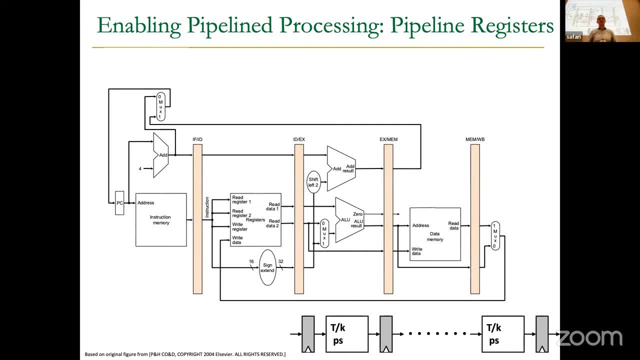 for another instruction. we need to add registers to isolate the different stages, right? This is necessary. Otherwise, if you have only one register to store one instruction, you cannot do much, right? You really need to have multiple different registers to isolate the processing. 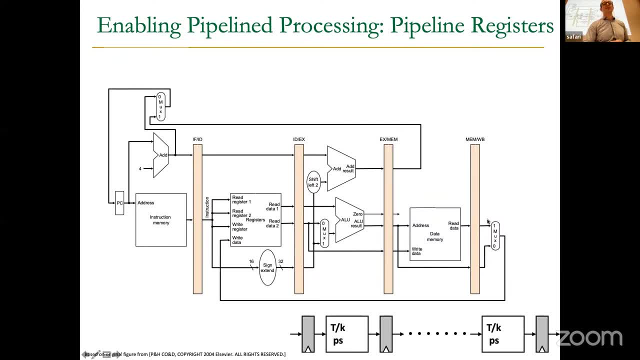 that's happening in this stage, from the processing that's happening in this stage and this stage and this stage and this stage, Now that you have a five-stage pipeline right, There's the fetch and this is an IFID register, The register. these are called pipeline registers. 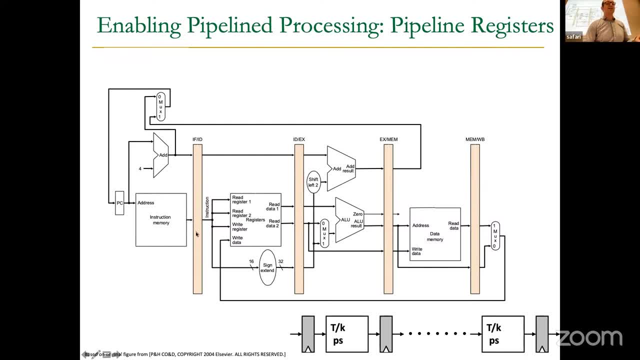 It could, for example, have the instruction that we fetch from memory. It could have PC plus four, as you can see over here. It could have some other control information, as we will see later on. This is the IFID register. register between instruction. 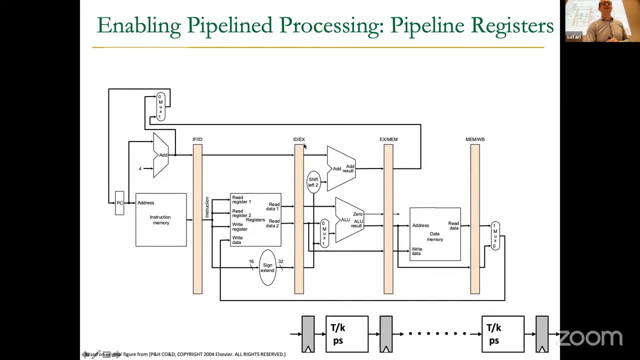 and instruction decode stages. This is IDEX register, pipeline register between instruction, decode and execute stage. This is XMEM, which is instruction or pipeline registration and execution stage. This is IDEX register, pipeline register between instruction, between execute and memory. and then this is a pipeline register between memory and writeback. 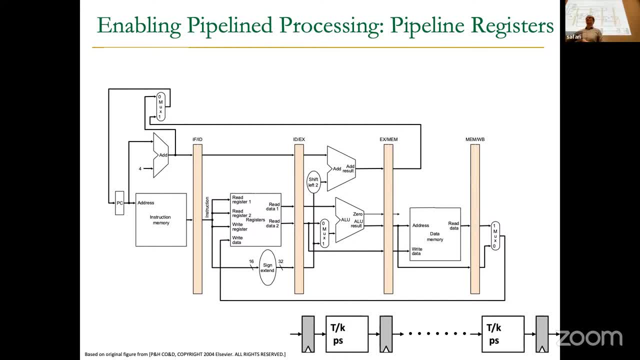 stages Makes sense right. So we'll basically latch the results. Very similar to a multi-cycle machine actually. So this is going to be similar, except we're going to do something different, also because we're going to process multiple instructions concurrently. 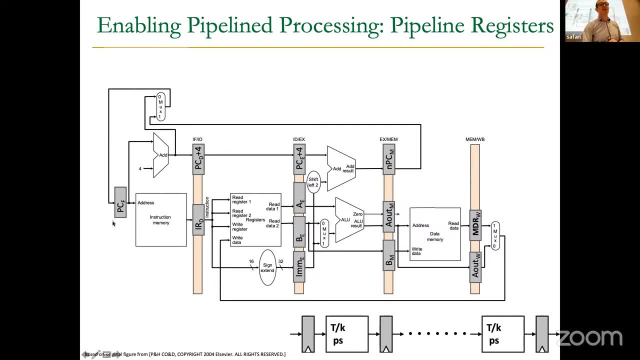 in the different stages. Yeah, these are some examples. So this is program counter. For example, in the first register you have the instruction register, which we used to have, and then in multi-cycle and then PC plus four, And then here we have PC plus four propagated. 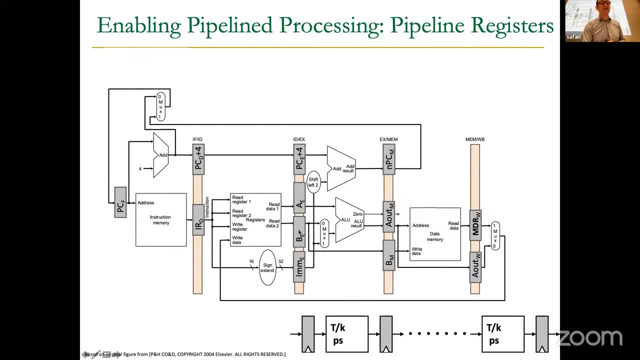 because we're going to need it later. And then the registers that we have read and the sign extend immediate. And then here we have the next PC calculated, in some way latched, and then output of the ALU and some other information, maybe zero, for example, This is for branch condition. 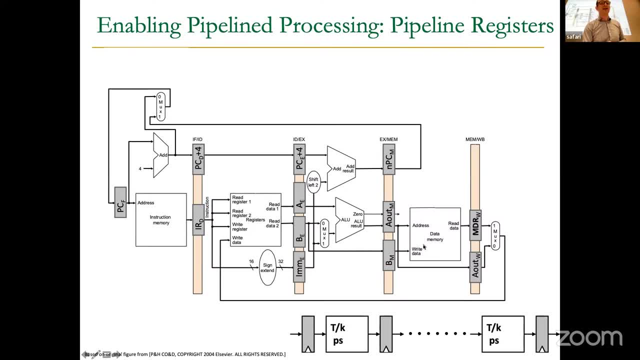 checking And then the other register propagated so that we can write the data in a store And then you have the data read From memory over here and the address- No, sorry, the output of the ALU, so that we can. 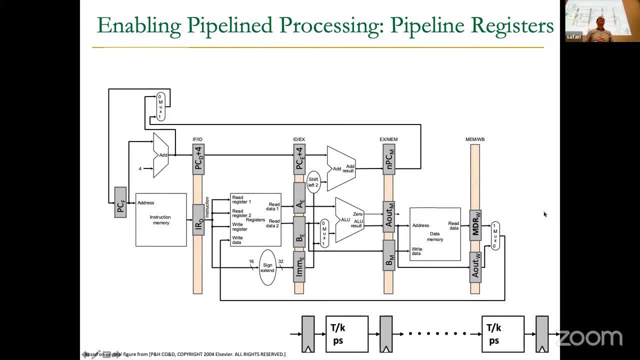 write it to the register at the last stage. Okay, So you need to propagate whatever information you need for the later stages in the pipeline, Because if you don't do that, you won't be able to do the processing as dictated by that particular stage. And this is just data We're 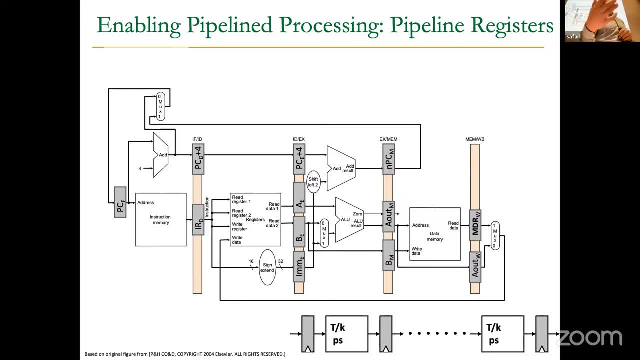 going to also add control information. So pipeline control is going to be very similar to actual single-cycle control, but we're going to propagate the control signals to the next stage And then we're going to add control information. So pipeline control is going to be very similar to actual single-cycle control, but we're going to add control information. So 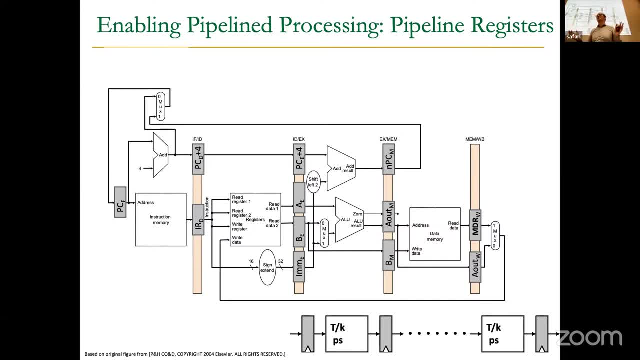 appropriate places when they need to be applied. This makes sense. also, right, You're dividing the instruction processing, so you should really carry the data values that you need to the appropriate place in the pipeline. That's why you need registers. Any questions? Okay, So no resources. 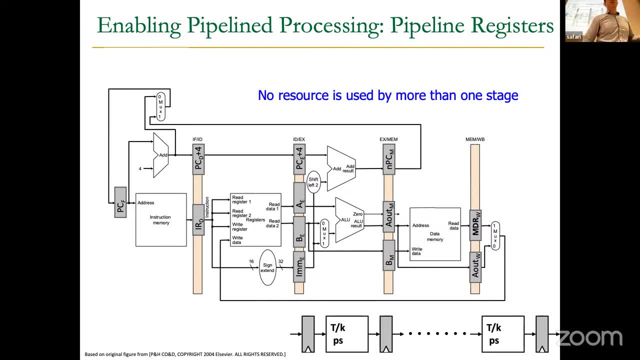 used by more than one stage and you should really ensure that, Otherwise you'll run into conflicts. Okay, So all instruction classes also must follow the same path and timing through the pipeline. So you should really ensure that, Otherwise you'll run into conflicts. Okay, So all. 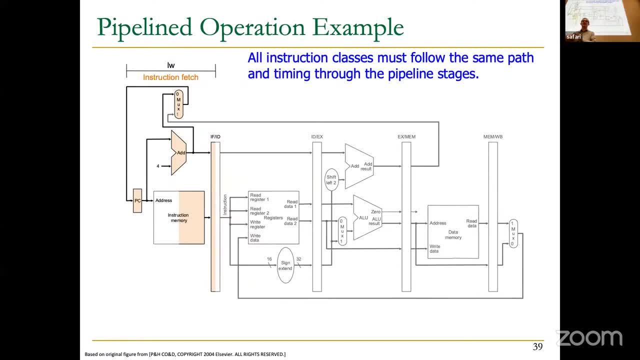 instruction classes also must follow the same path and timing through the pipeline. Okay, So all instruction classes also must follow the same path and timing through the pipeline. Appreciate that, Because this is a pipeline. you feed in instructions and instructions get out. 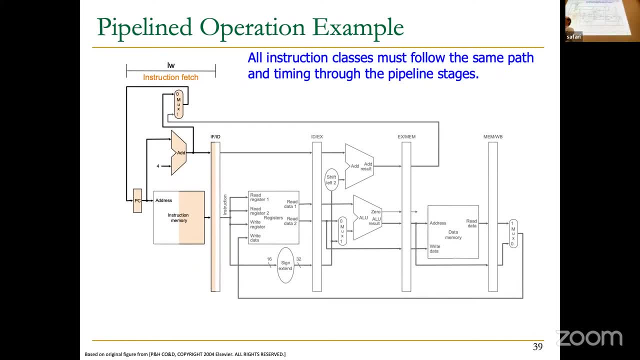 Even though an instruction may not do useful work. remember, in the instruction processing cycle there are some instructions that don't do useful work in some stages. we're going to run into that again over here. But there's no easy way of removing them from the pipeline early. So all 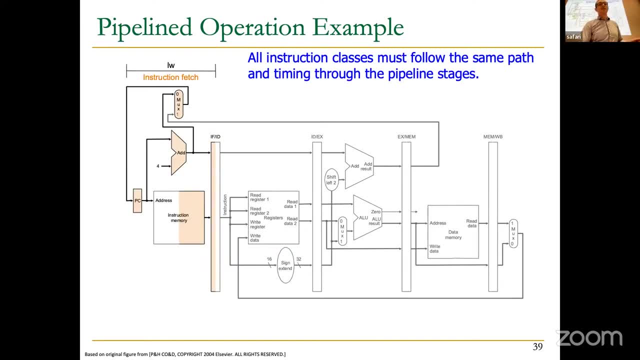 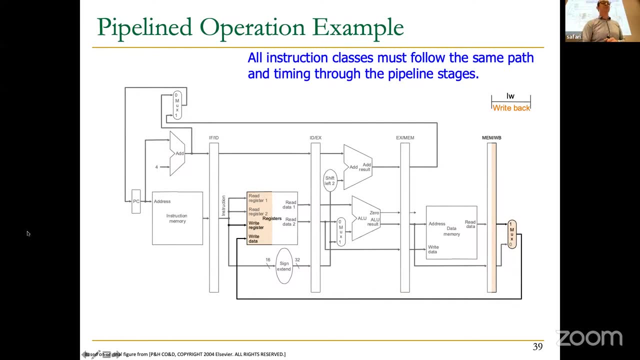 instructions will flow through basically, So they will go through instruction, fetch instruction, decode, execute memory and write back. Load word needs everything, But some other instructions, like jump doesn't need everything, But we need to make sure all of them flow through the pipeline so that we can. 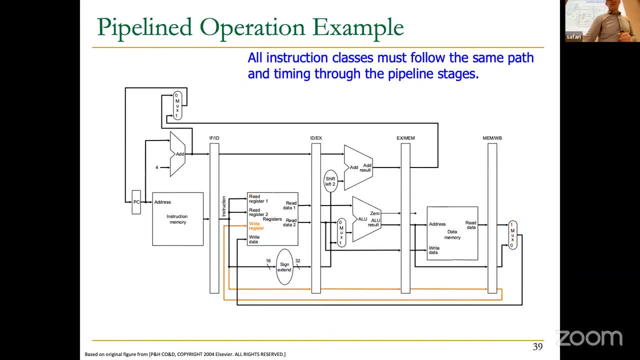 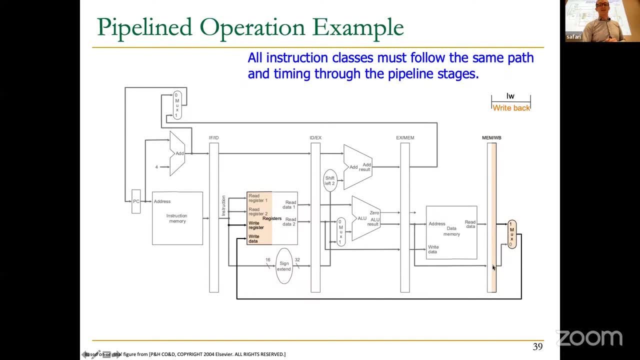 ensure sequential execution. OK, And then this is, if you look at this over here. So if you want to write back to a register, clearly you need to get the data that you loaded from memory over here and write it into the register from here. 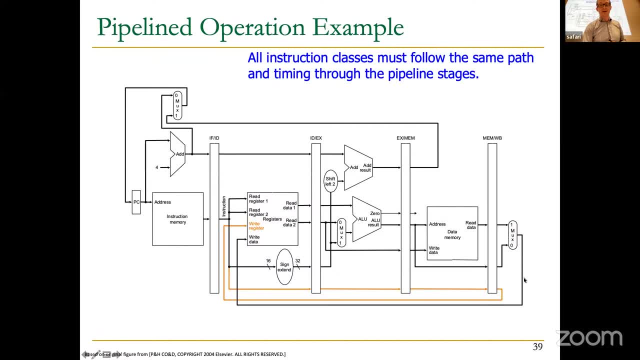 So you actually have the right register signal. So the data is coming from memory over here, if you see. But you also need the ID of the register propagated. So this is one example of what you need to propagate. So the load word is going to write to a register. 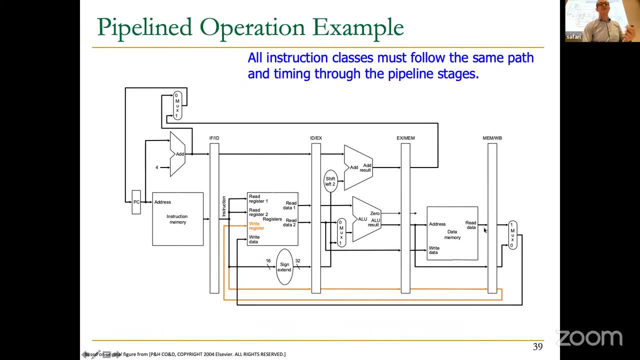 in the write back stage. Before that it will read the data from the memory And then it will latch the data And then the control signals will be assorted appropriately such that the data is communicated from the write back into the write data port in the register file. 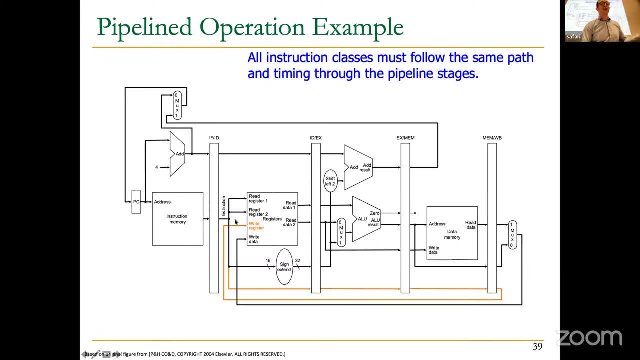 But then you also need the register ID which you generate when you decode the instruction, And that needs to be. When you decode the instruction, you need to propagate the register ID And also the control signal to write to the register. So that's not shown over here. 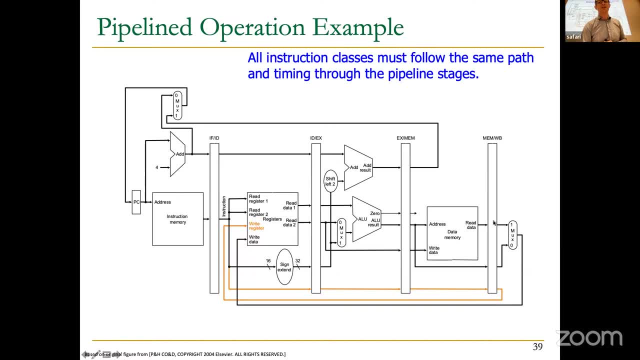 But there is a control signal that says you're going to write to a register That actually needs to be coming from this register over here, Because that's really associated with that instruction in that particular stage. Makes sense, right? OK, So any performance impacts. 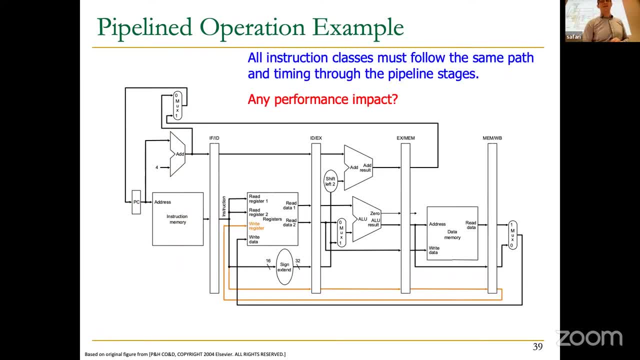 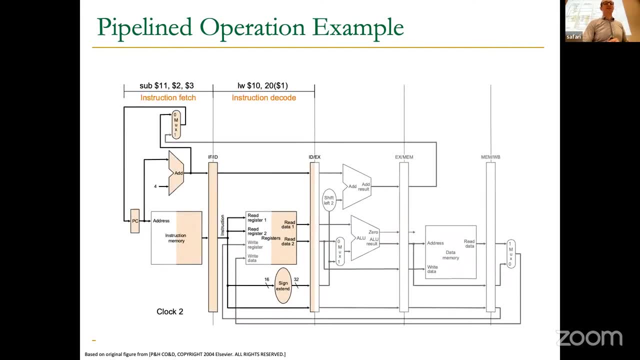 And there will be a lot of performance impact, as we will see. So I'm going to ignore that question right now. OK, OK. so basically, life is beautiful if instructions are not dependent on each other. So this is an example of load word followed by subtracts. 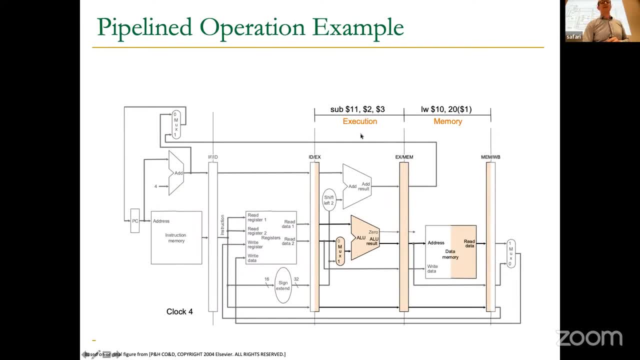 And they can nicely flow in the pipeline because the subtract is not dependent on the load word. But if the subtract actually was sourcing register 10, then you couldn't move the subtract over here. Why? Because this load did not even write to register 10 yet. 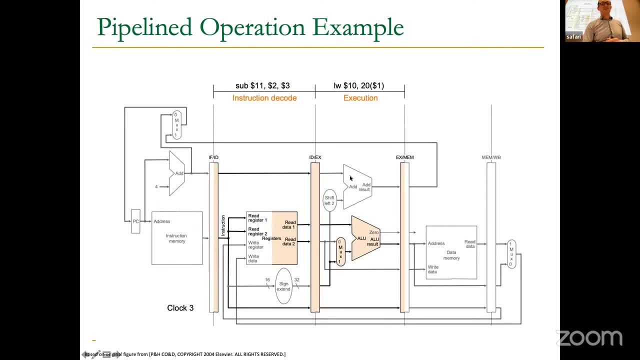 Right, So let's go back. So load is executing over here. It's calculating its address Basically: it's taking register 1, adding 20 to it, plus, yeah, multiplied by 4, as the ISA specifies, right. 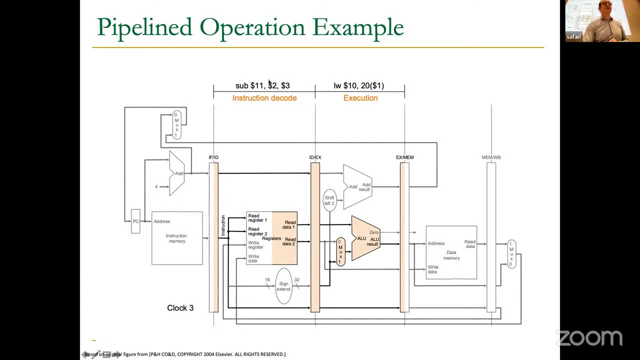 It generated its address. This instruction is being decoded and accessing the register file right now. It's independent. That's good. But if it were dependent, if it were sourcing register 10, it would read the wrong value of register 10 over here. 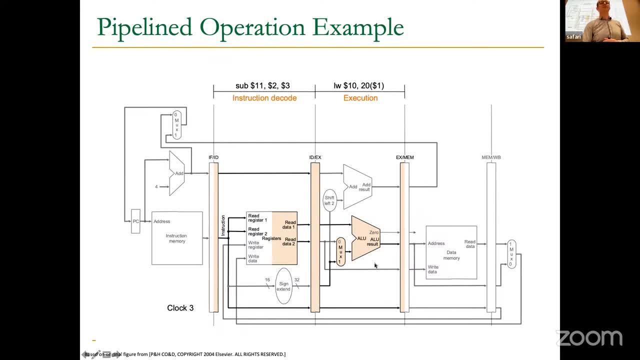 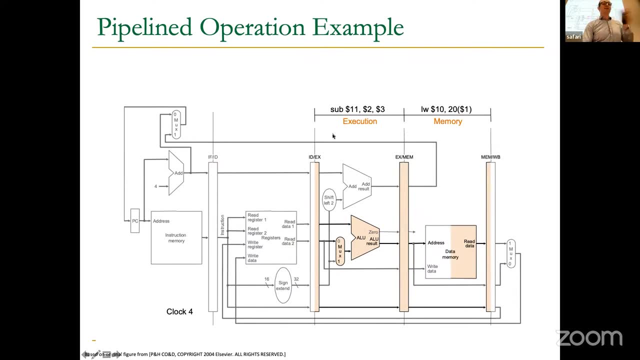 because this load word did not write to register 10 yet Right. So let's assume that we ignore that. This load word moves to memory access And the subtract. if the subtract is independent of the load word, that's fine, no problem, because the subtract doesn't need. 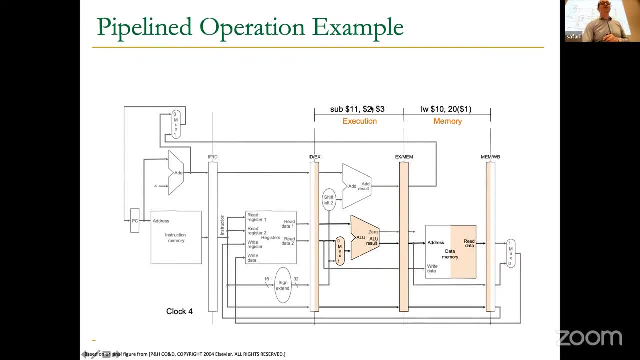 anything from load word at that point. But if the subtract is sourcing register 10, and if it is moved to the stage, it's computing with the wrong value because load word did not write to that register yet, Right? So that's basically the key distinction. 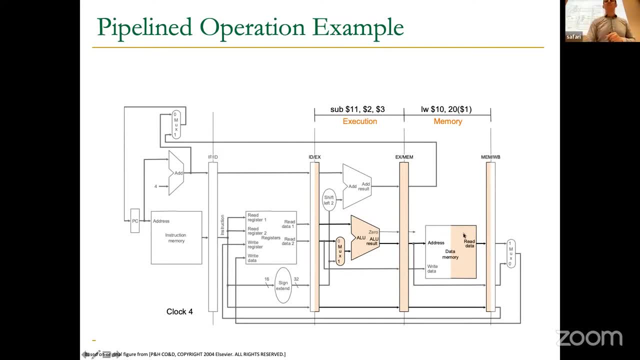 from an ideal pipeline, one of the key distinctions from ideal pipeline and an instruction processing pipeline. These instructions- the second instruction, later instruction- may have a dependence on the first one. As a result, this instruction subtract instruction if it's dependent on load word, which is not the case here. 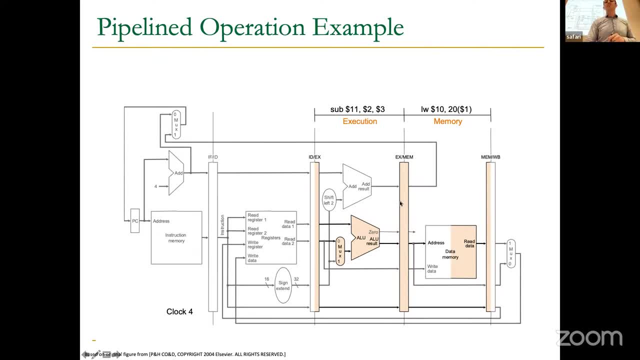 but assume that it's sourcing register 10,, for example. it should not have moved to the stage. It should have waited until it knows it's going to get the correct value, And this is called data dependence handling, And we're going to see methods for doing that later today. 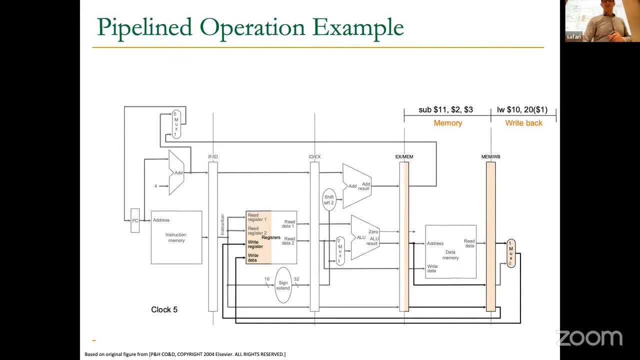 Makes sense, right? OK, So clearly, load word is writing to the register at this stage And if your subtract has moved over here and it was dependent, you've done the wrong thing in your pipeline because subtract got the wrong value. OK. 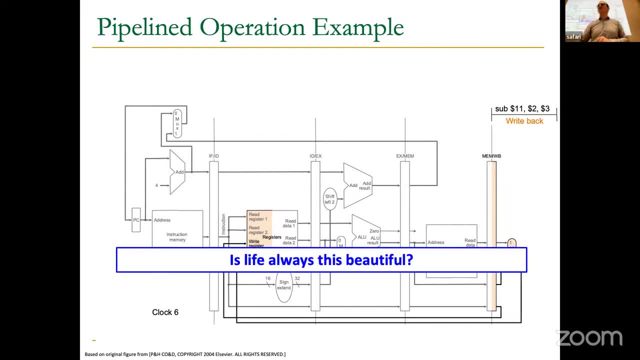 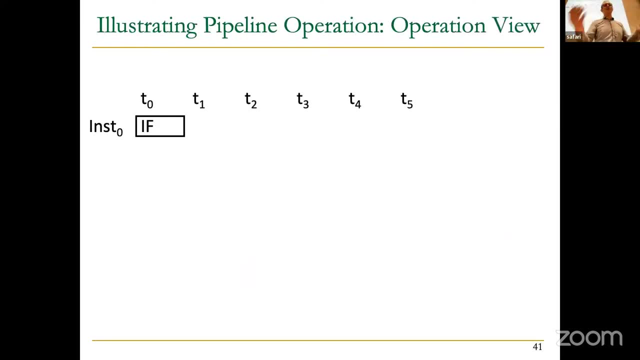 But we're not going to do the wrong thing, as you will see. So his life is not always this beautiful, because this example didn't have any dependency, But I kind of explained it to you with a dependency also. OK, So if there are no dependencies, pipeline operation. 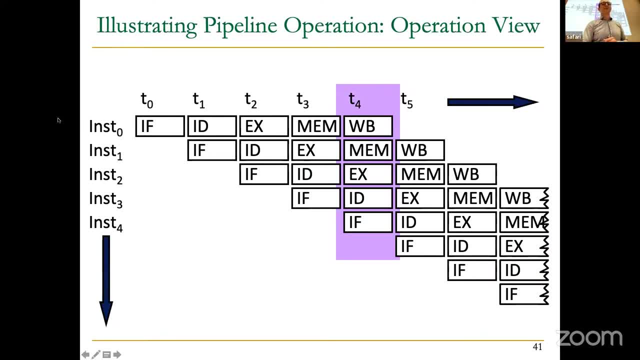 looks like this, basically. I mean, we've kind of seen this in a different way, But you've filled the pipeline at this point And this is the steady state. Your pipeline is full. You have five instructions in a five-stage pipeline. 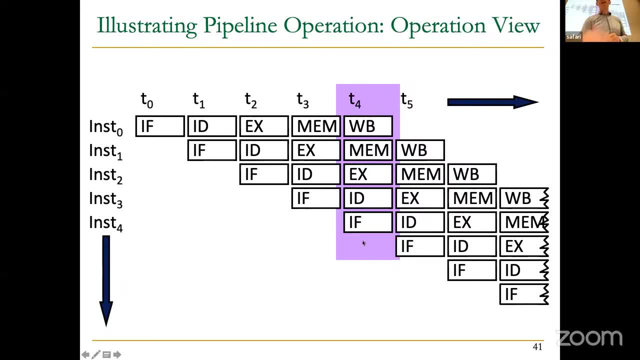 And you're finishing one instruction every clock cycle. That's good. Dependencies are going to hurt us because some instructions need to wait And you cannot move the pipeline. if an instruction needs to wait for an earlier instruction to produce the value, OK, Just to define. this is called a steady state or full pipeline. 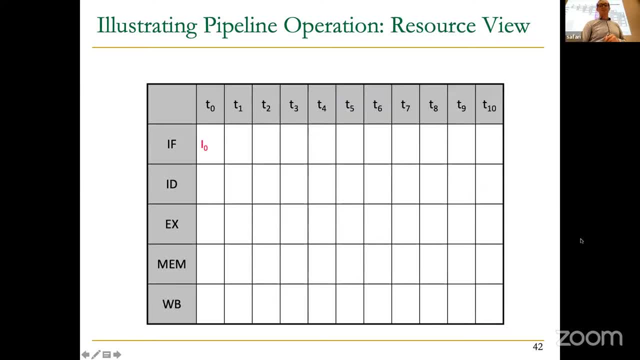 And you can see that the pipeline is full every cycle after this. And this is another view, This is the resource view over here. If you look over here on the x-axis, you have time, different time steps, clocks, clock cycles. 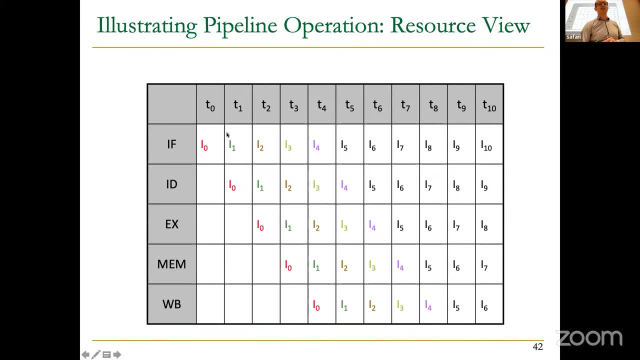 And you have resources And basically you look at which instructions are using which stage. Again, it's beautiful to look at, But when you have dependencies, you will have a lot of bubbles. if you will, We'll introduce the term bubble also. 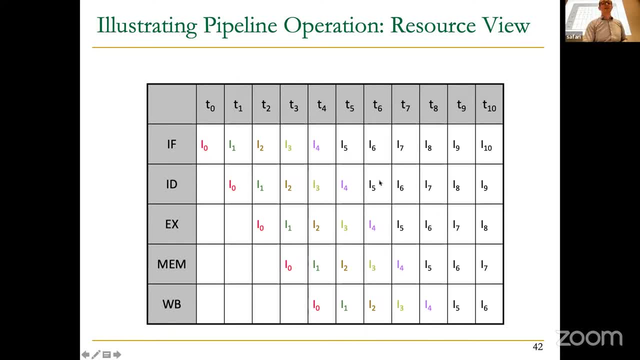 Some part of the pipeline will not be full. So, for example, if instruction four could not have moved because it's waiting for a value from instruction three, this would have been a bubble And, as a result, there would be no instruction over here. 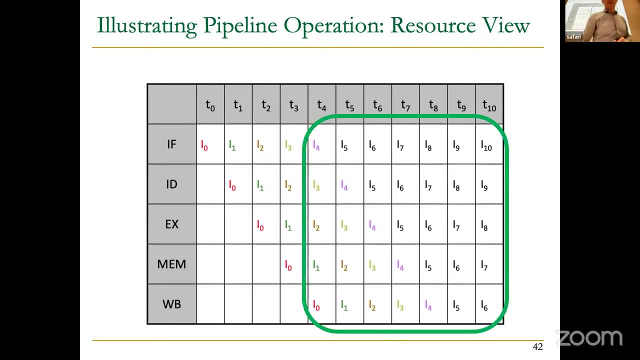 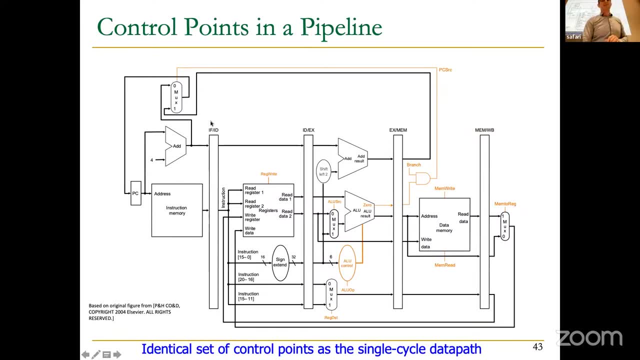 You can think of that as a no operation also. OK, we'll get to that. So that's a steady state. OK, so now let's talk about controlling this pipeline, because we need to control it. We've kind of designed the data path already. 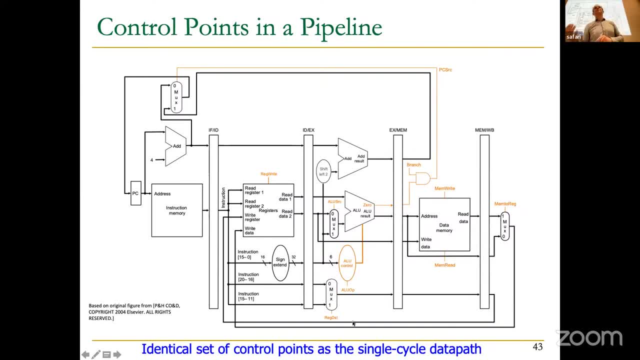 These are the pipeline registers, And controlling the pipeline is actually relatively easy. That's one of the other reasons why we designed the single side cycle processor earlier, because the control points of a pipeline is really identical to the single cycle data path. So if you look at all of these control signals, 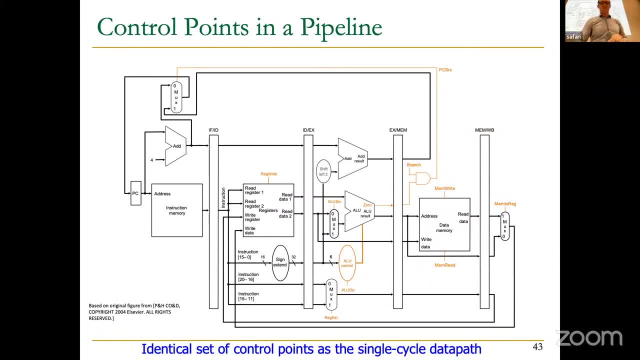 and if you compare them to your single cycle data path, you will see that they're exactly the same, Except different instructions are exercising the different control signals in different stages. That's why you need to propagate the control signals with the instruction and exercise it when it's needed. 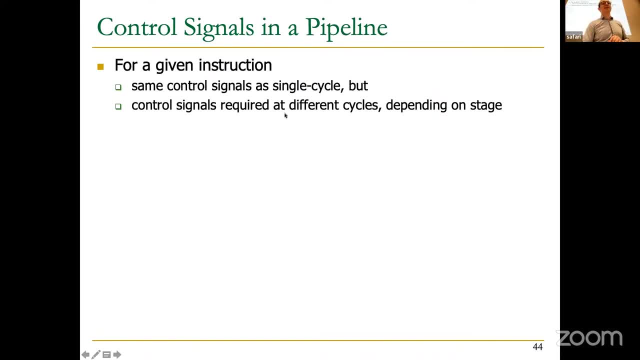 OK. so basically, for a given instruction, you have the same control signals as a single cycle, But control signals are required at different cycles depending on the stage that the instruction is in. So there are multiple options of designing the control logic. I'll give you the first option in more detail. 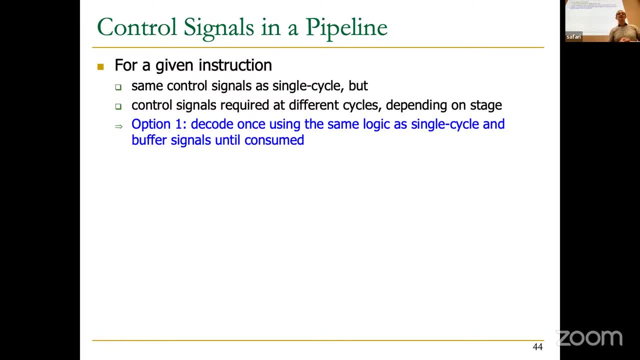 But basically you decode an instruction once in the decode stage using the same logic as single cycle control logic that we have developed two lectures ago, And you remember that that control logic was a combinational function of the instruction, right, If the instruction is this: register write signal. 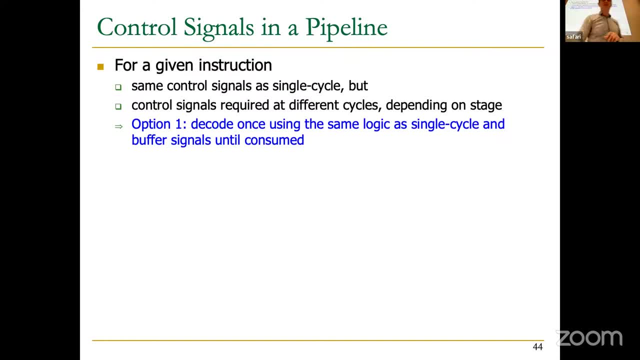 should be set or not set. If you don't remember, go to that lecture two lectures ago. But we buffer the signals until they come to the stage where they need to be consumed. So it looks kind of like this: This is the pipeline again for pipeline registers. 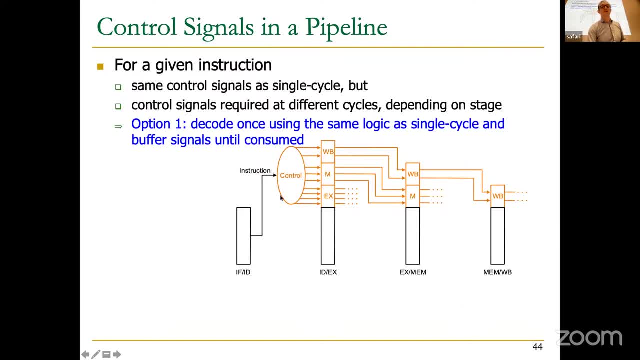 Fetch, decode, execute, memory, write back And control logic is exactly the same as what we discussed two lectures ago. But then you divide the control signals into: oh, these are my control signals that I need in the execute stage. These are my control signals that I need in the memory stage. 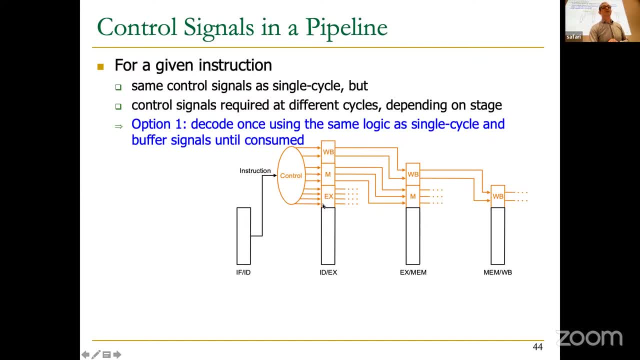 These are my control signals that I need in the write back stage And you put them into a pipeline register over here And then keep propagating them until they're not needed. So, for example, once you move to the stage, you don't need the control signals that are really 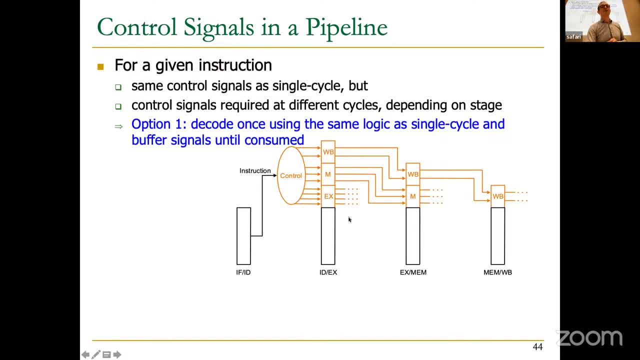 needed in the execute stage, which is the ALU, et cetera. So you drop them. You don't propagate, used unnecessary control signals indefinitely until the end of the pipeline, And then here you use the memory stage control signals to do the processing. 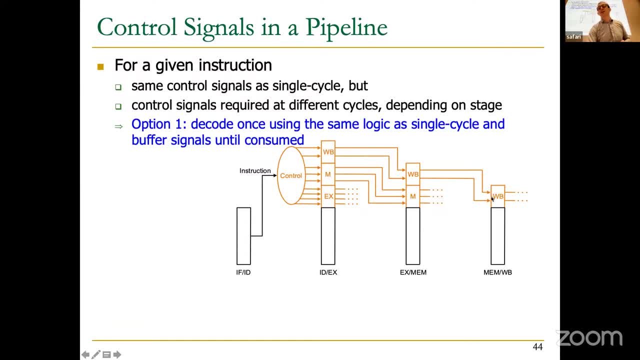 while the instruction is in this stage And then you drop them when the instruction moves to the write back stage, because they're not needed, because you have a separate set of control signals that you designated as write back control signals. Makes sense, right? 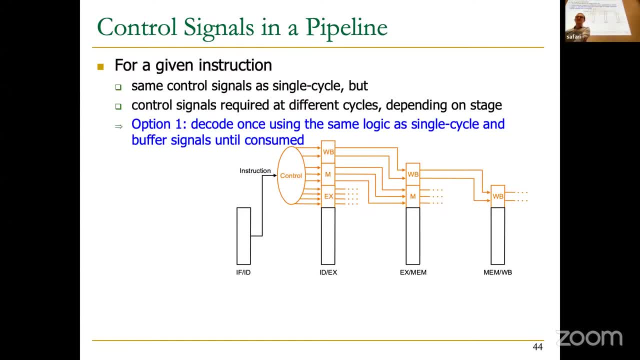 OK, So you can see that this causes some imbalance in the register size. also, right, Unavoidably, the register that comes after decode is a bit bigger because you really need to have all of the control signals that are needed for all of the stages. 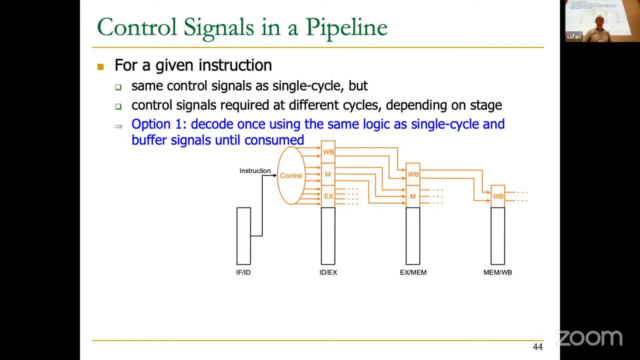 downstream, So in a five-stage pipeline it's not bad, but some of pipelines today are 20, 25 stages, So there could be a huge imbalance between the register sizes basically. So there's another option which is also used actually in some machines. 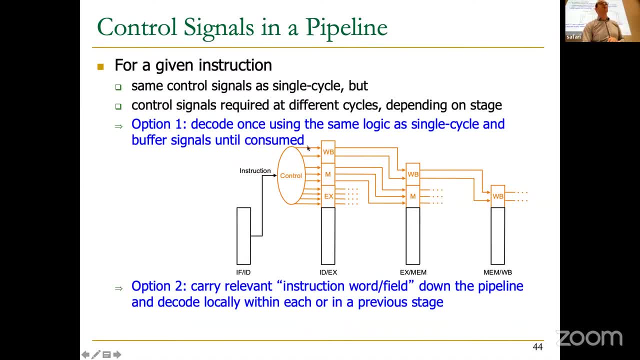 You carry the relevant instruction, word or field. You don't do the complete decoding over here. You basically do decoding incrementally as the instruction moves along. So you distribute the control logic or, yeah, you essentially distribute the decoding. I should say: 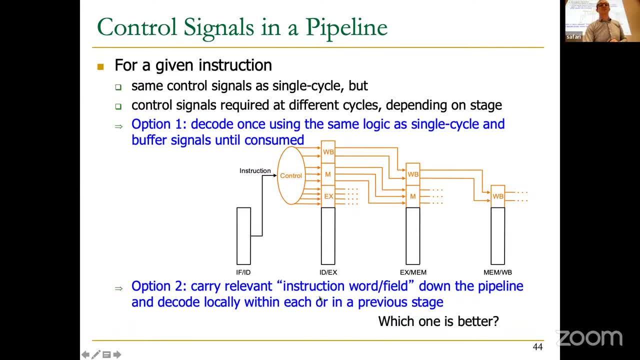 You distribute the decoding across multiple stages Makes sense Here. I don't have a picture that shows that, but basically here you do the decoding that's needed for the execute stage. Here you have another control that decodes and figures out. 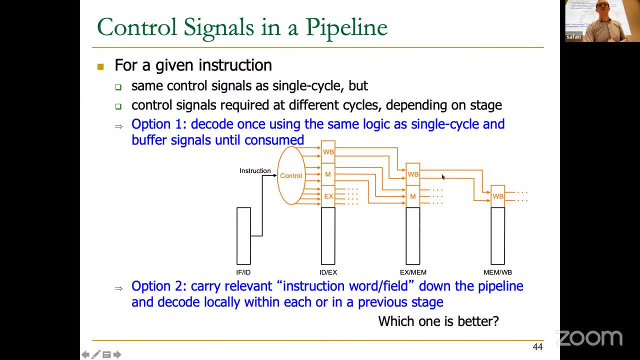 the signal that's needed for the memory stage only, And then here you have another control that figures out the signal that's needed for the write back stage, So it can still overlap control and data processing. You generate the control signals that's needed in the next stage, in the previous stage, basically. 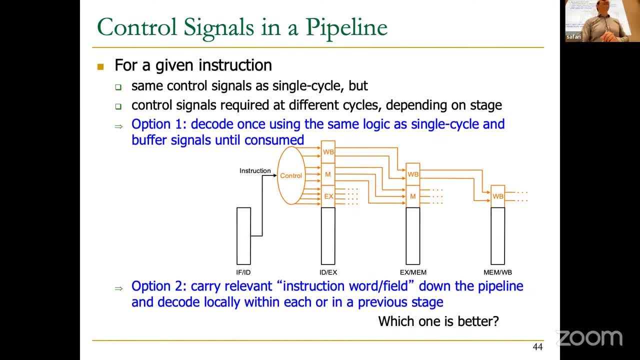 That's the idea. So which one's better? Again, it depends. So it depends is a good answer. The first one does the decoding at one shot in one stage, but then the registers become bigger, So it basically uses unnecessary things. 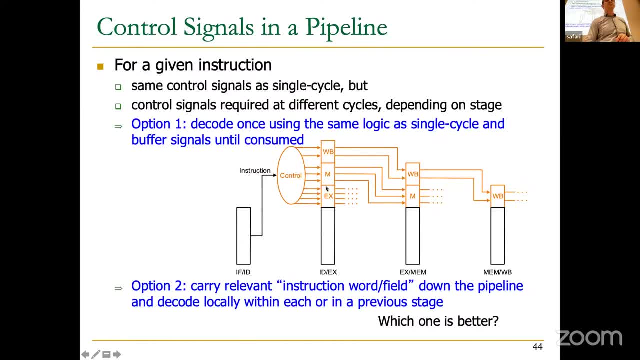 The second one does the decoding more incrementally, So it saves some registers actually Without actually increasing the decoding logic too much. So the second one is more frugal in terms of hardware cost, But the first one is maybe easier to handle. 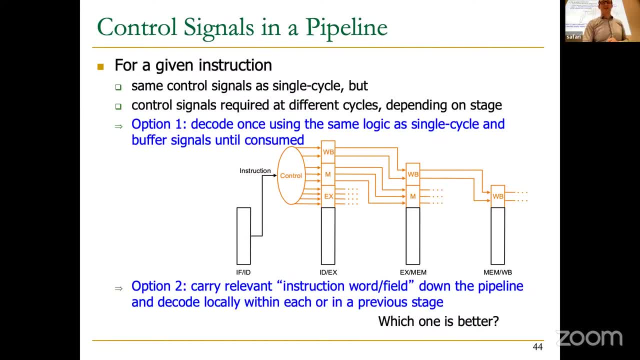 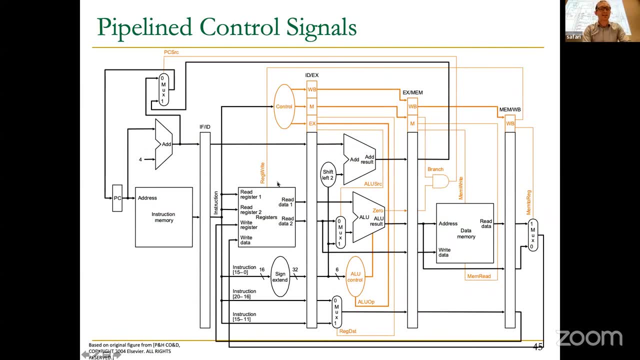 Any questions. There could be other trade-offs, of course, but we're not going to cover them, like energy. OK, so these are the pipeline control signals. This is from this book, but your book is kind of similar. You can see that this book takes the approach of the first option. 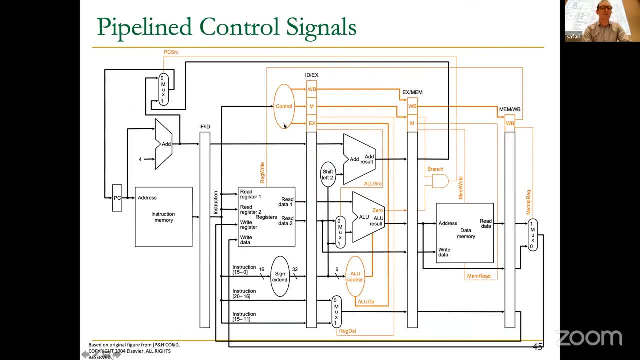 because also it's conceptual, It's easier to explain. You do the control or decoding right away and then you generate the control signals that you need and then you propagate them until they're not needed at some point. But you see that, for example, this execute stage control. 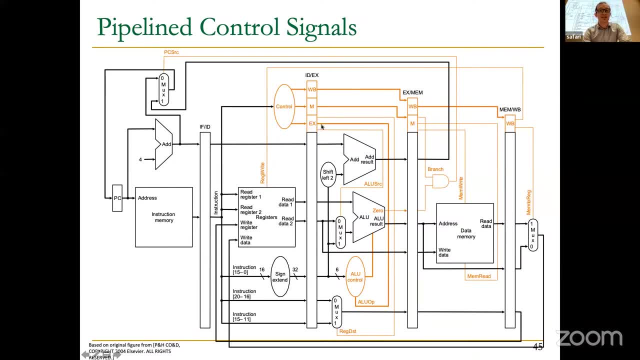 signals after they're generated in the prior decoding stage. they actually control what goes into the ALU, what's done in the ALU, which destination register you actually have and propagate it, et cetera. But the control Control signals. if you study this in a little bit more detail, 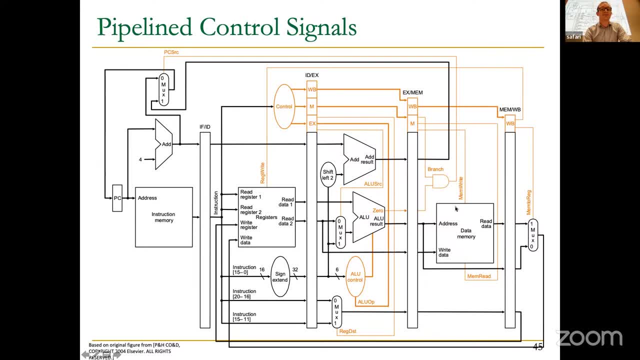 you will see that they're exactly the same as single cycle. If you remember single cycle, we had all these control signals and they're exactly the same. What else should I talk about over here? So one of the issues is going to be making sure 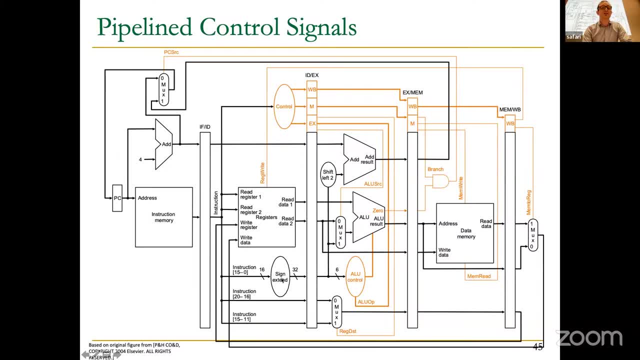 that you get the right value from the right place. So you need to make sure that you propagate the right control signals to the right place and you propagate the right data values to the right place. We're going to look at that later on with an example. 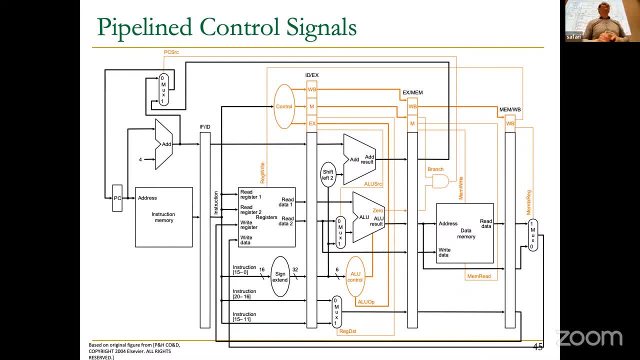 from your book. actually, This is correct. There is no issue over here, OK. OK, So I've already said this, but basically, you propagate the control signals that are needed for writeback. you generate them over here and then propagate them. 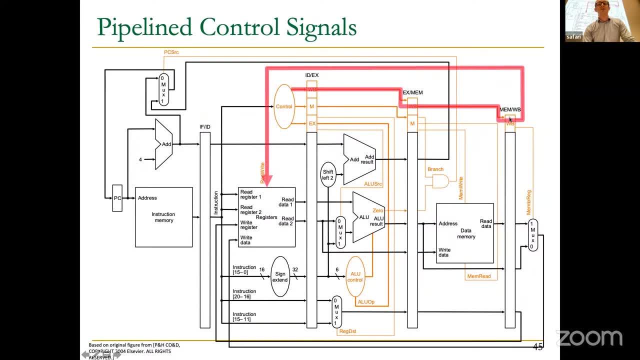 until they're needed. So the register write signal should be used from here, But this signal- register write signal- in the execute stage or memory stage. that doesn't mean that it's not useless. As we will see, it's going to be used for dependency detection. 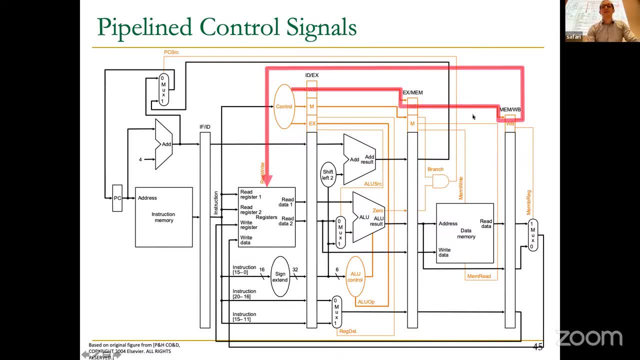 Why? How do you know So, whether an instruction over here is writing to a register? Well, you look at the register write signal that's associated with the instruction in this memory stage over here, basically, So the signal that's buffered over here, that. 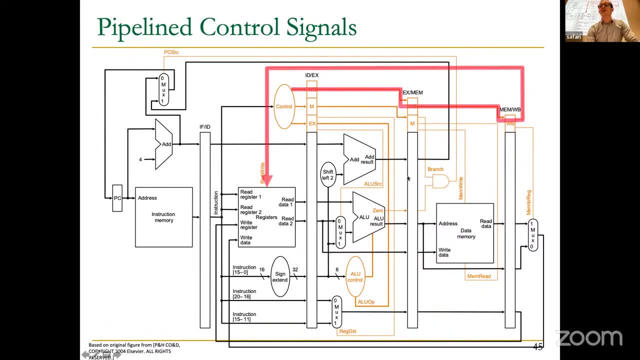 is to be used later on actually to actually write to the register can be used for some other purpose. over here This instruction can say: oh, my control signal over here, register write- is set. So some other instruction that's coming later. that depends on me. 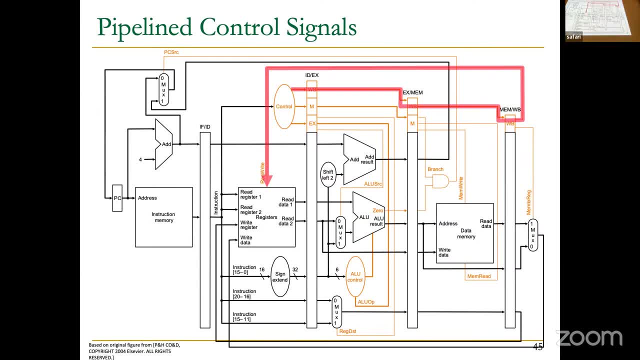 should wait, OK, OK, So there will be some other logic that we will add to stop the instructions that are going to be dependent on instructions that are in the later parts of the pipeline. Does that make sense? So these control signals are going. 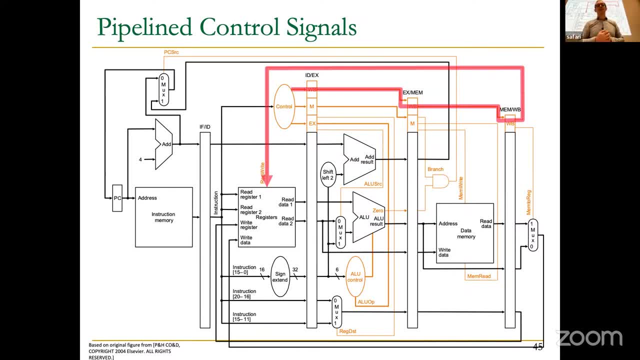 to be used for multiple purposes, now for dependency detection mainly, and for some other purposes later, as we will see. So we're going to complicate this pipeline. This is, right now, not handling dependencies well, Or it's assuming something about dependencies, I should say. 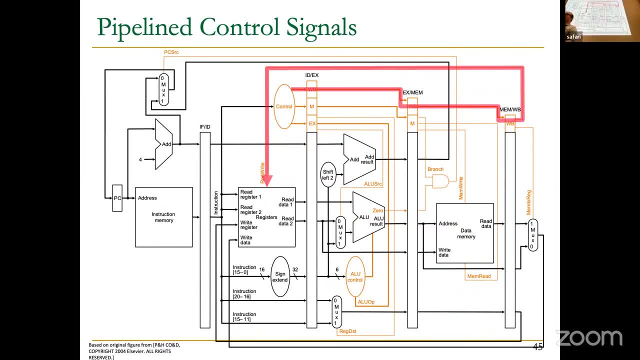 Because there are ways of handling the dependencies in the compiler. as we will see, Compiler Figures out which instructions are dependent on each other and separates the instructions enough in the instruction stream, such that you never need to check for dependencies in the hardware. 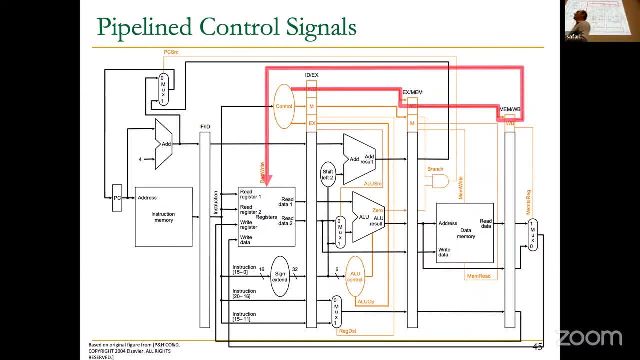 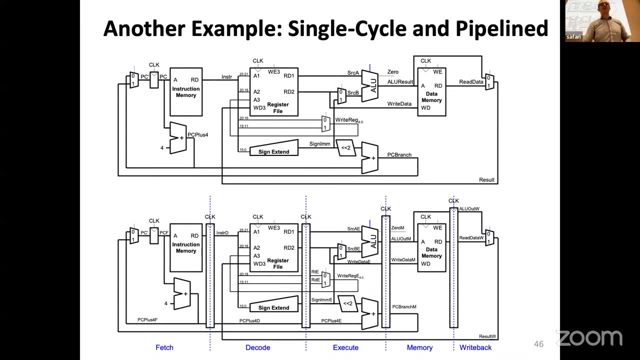 Does that sound good? It's called software-based dependency detection, or interlocking, And whenever you can do it, it could be good, But we will see some issues related to that as well. OK, So this is another example from your book. 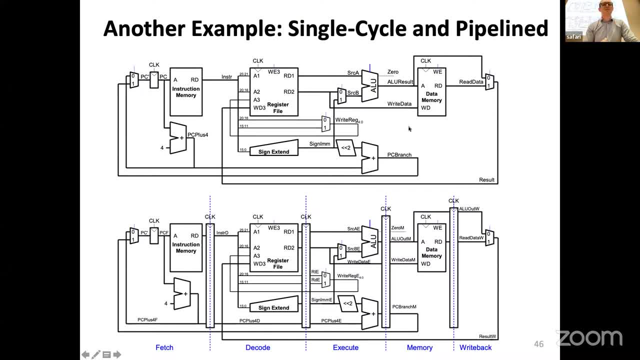 So you can read your book. similarly, And as you by now figured out, I believe, different processors are very similar, And these are also MIFS processors. That's one of the reasons they're very similar. So this is a single-cycle microarchitecture. 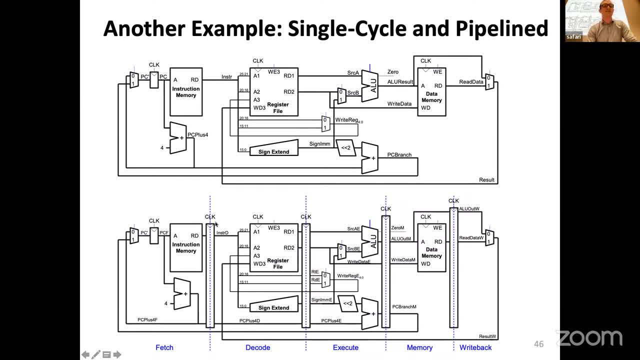 that we have seen from your book And this is the pipeline microarchitecture that your book develops. As you can see there, the pipeline registers. It's a very similar stage also And the structure of the pipeline is very similar, And your book also shows that your control signals are. 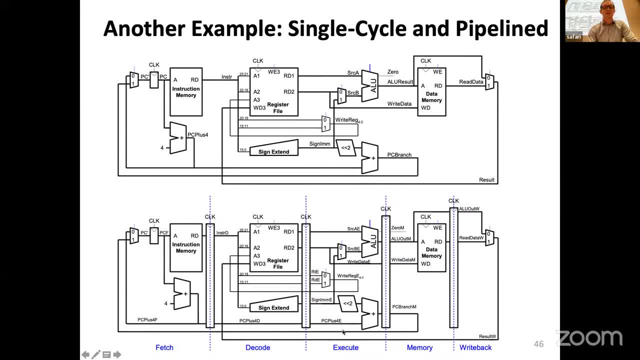 exactly the same in the single-cycle machine as well as the pipeline machine. Now, your book also illustrates some things like this. This should not be happening. Basically, there's a writeback stage where you should be writing to the register, But someone designed the pipeline such that the register 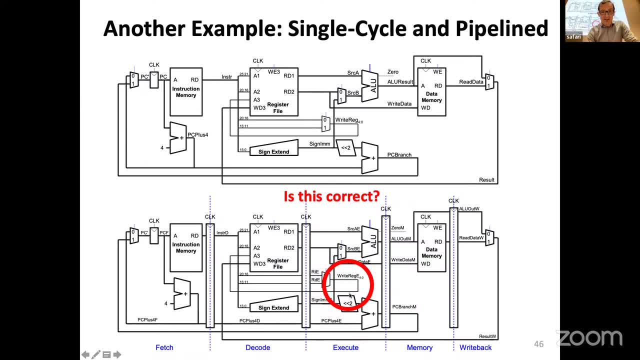 ID that you're writing to is coming from here, So you need to be careful. Basically, the whole point of this example is you need to be careful with these signals that are crossing stages, And this is the register ID that you're writing to. 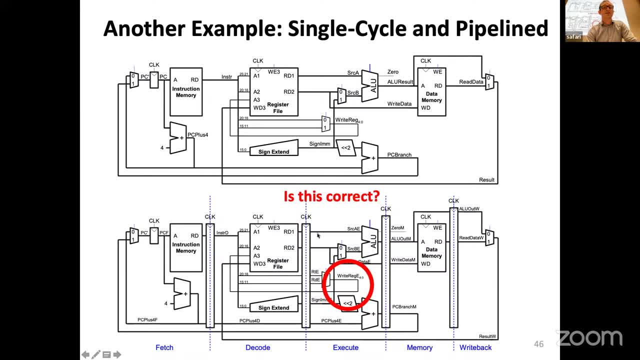 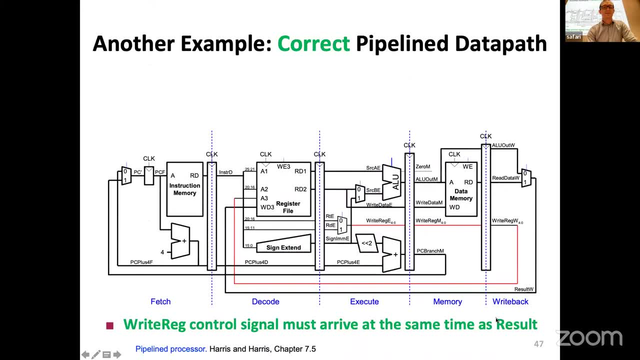 It should not go over here, because the instruction over here should not write to a register at this point. It should buffer its result And it should write to a register at this point. It should write to a register at the end. OK. 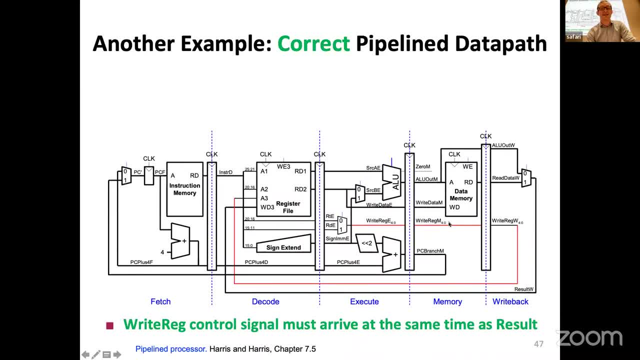 So basically, this is the corrected signal. Corrected signal actually needs to be propagated. That's the register ID And it needs to be used over here to be supplied to the register file. Make sense? That's how we divided the tasks. 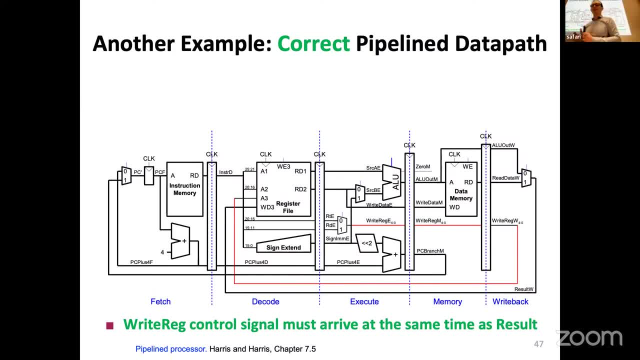 You could have chosen a different division, then You should do something else. But if you divide it this way and if you make sure registers are written at the end of the pipeline, this is what you should do, And we're going to see the real reason why we write. 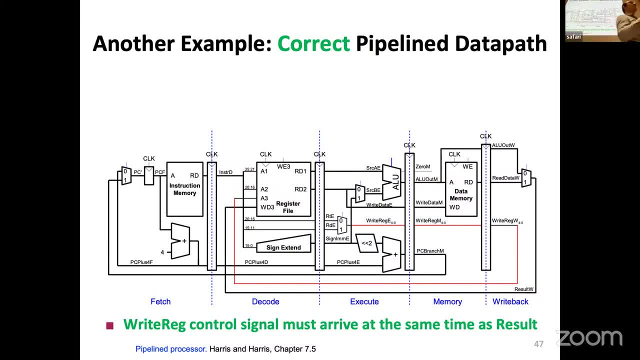 at the end of the pipeline next week or the week after. So hold off on that You could have questions. Why are we writing registers at the end of the pipeline earlier? There are dependencies that will complicate things, for sure. But there's another real reason, which. 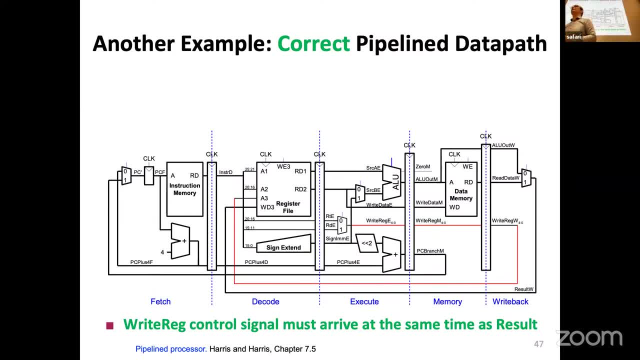 is making sure the semantics of the Neumann model is obeyed, But hold off on that for now. Basically, the takeaway is you should really use the control signals as well as the data signals from the right stage when you're crossing the boundaries of stages like this. 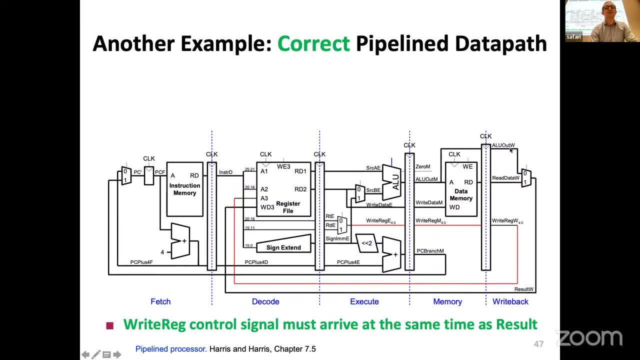 I mean, logically, you're not crossing the boundaries. Logically, what you're doing is belonging to the instruction in this stage, But physically, in terms of the resource, you're kind of crossing the boundaries of it. So, logically, this instruction is the instruction over here. 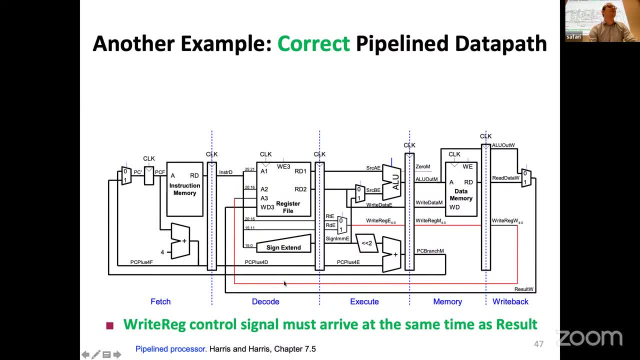 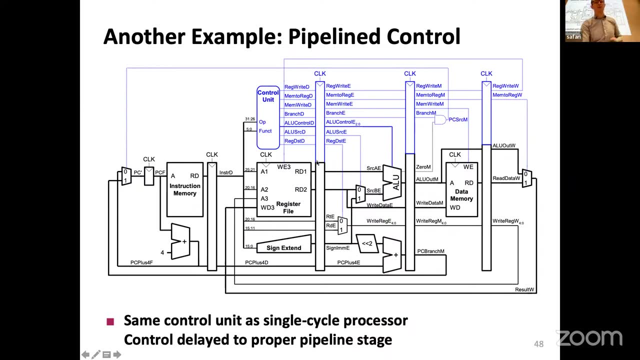 should be writing to the register file Physically. you need to ensure that also. So what I just said- propagating the signals- is physically ensuring what should be logically happening. OK, OK. So this is another example from your book. now, Now you can see the pipeline control from your book. 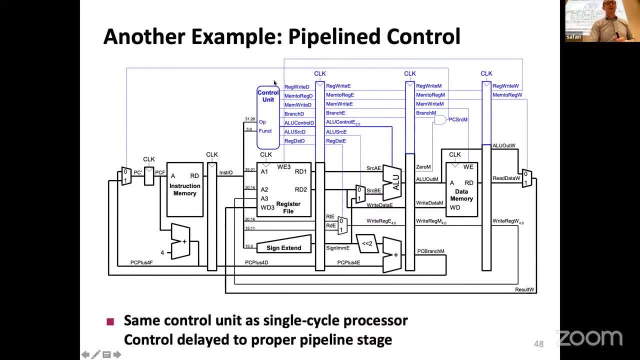 is also taking a very similar approach that I showed to what I showed. You have a single decoder or control unit that's generating all the control signals, And these control signals are buffered in this pipeline register and used whenever they really truly need to be used. 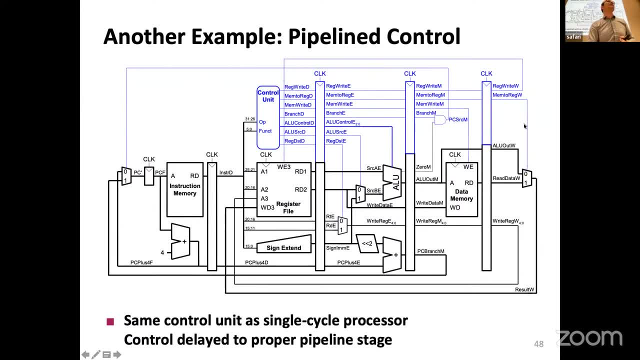 You can see that the register is getting skinnier, if you will, or shorter. OK, As the control, because the control signals that are needed at the end of the pipeline are a subset of the control signals that are produced over here. 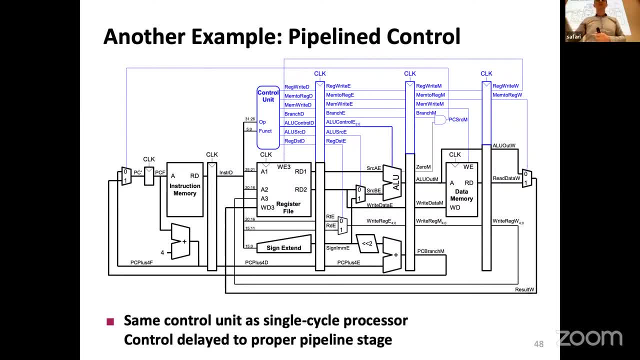 Makes sense right, And you've already seen this If you're not in your reading. actually it's going to be very easy, also because it's the same set of control signals as a single cycle processor. You just delay the control to the proper pipeline stage. 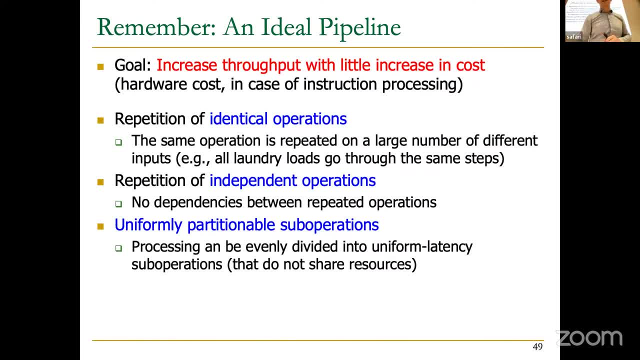 OK, So let's examine this ideal pipeline. So this was our ideal pipeline, And this is exactly the same slide that I showed you earlier. We repeat the identical operations, identical instructions. We repeat independent operations, independent instructions completely, And we uniformly partition the sub-operations. 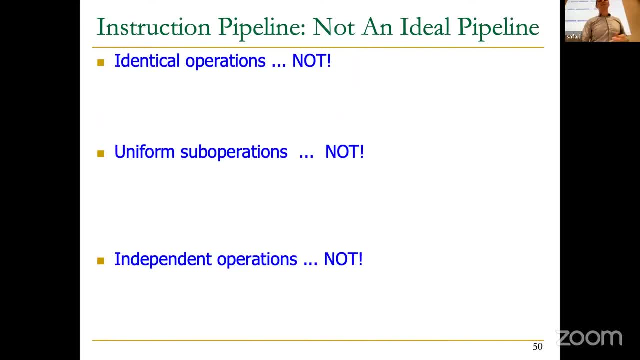 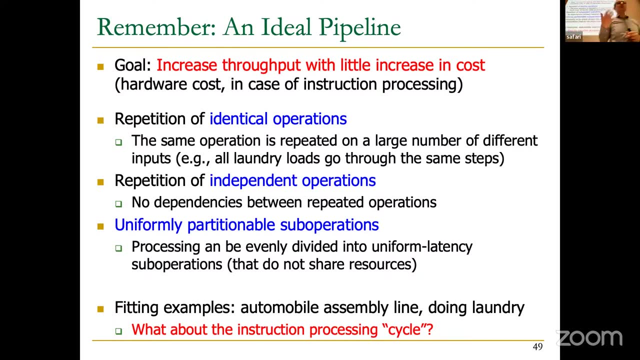 such that each pipeline stays uniform latency. Now let's examine, Let's evaluate. This is again our framework. You can think of this as a principled framework to evaluate the ideal pipeline And if you come up with another property of an ideal pipeline, 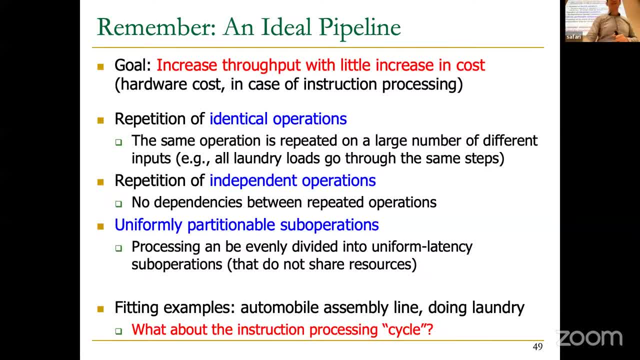 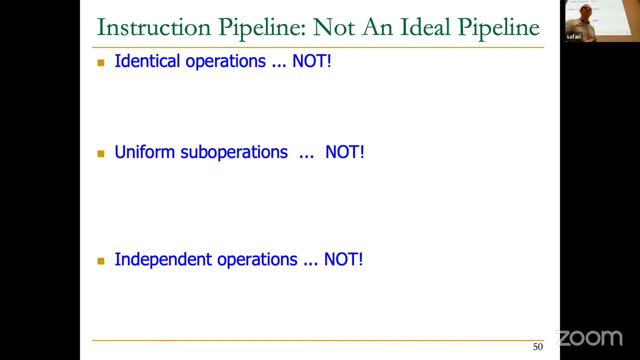 we should have added it, But these are the three major properties of an ideal pipeline that we have come up with. Let's take a look at whether the instruction pipeline satisfies these properties of an ideal pipeline, And it actually breaks all of them. let's say: 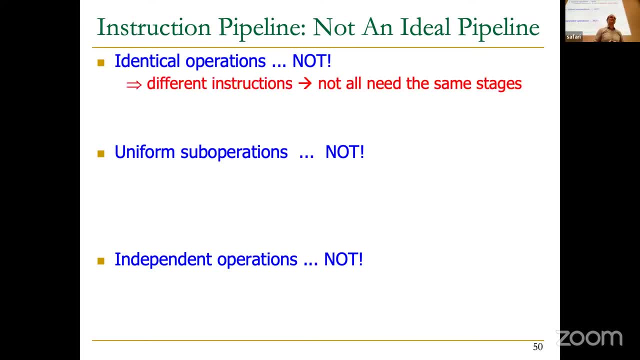 It's identical operations, No Different instructions. Not all of them need the same stages. Basically, we've introduced immediately some inefficiency to our pipeline because it's a pipeline but you feed everything through the pipeline, Basically forcing different instructions. 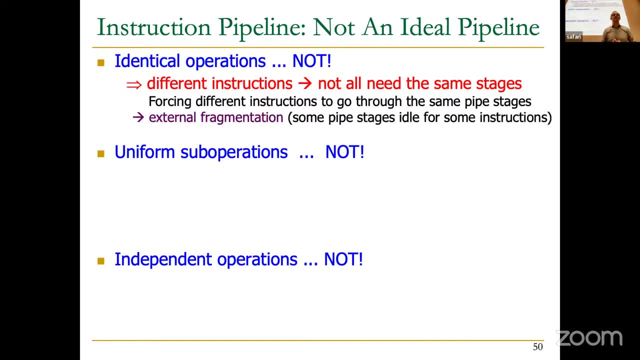 to go through the same pipeline stages leads to external fragmentation, meaning some pipeline stages are idle or useless, So you need to add a lot of complexity to your pipeline for some instructions. As I said, this is difficult to fix unless you add a lot of complexity to your pipeline. 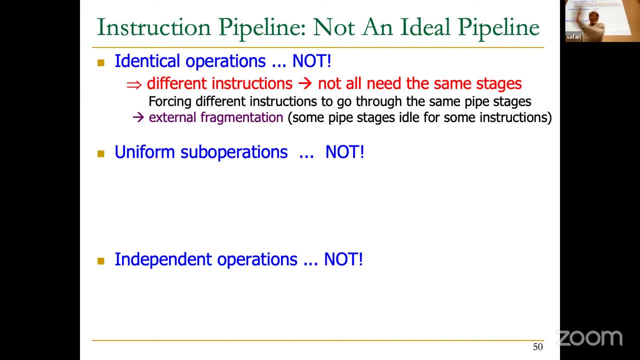 And after that point your pipeline is not a pipeline anymore. almost The beauty of the pipeline is everybody goes through the same assembly line. If you try to fix this external fragmentation you could do it at very high complexity, but it's not a nice looking pipeline anymore. 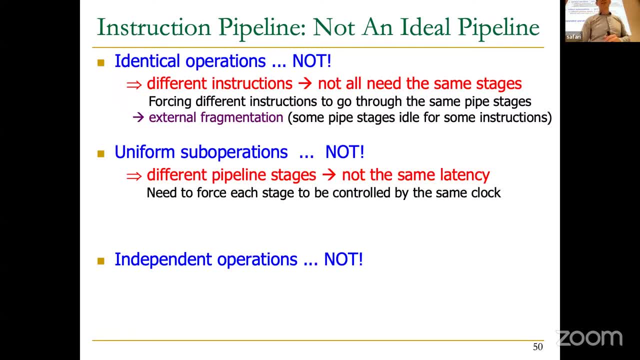 It's not as beautiful. OK, Uniform suboperations, different pipeline stages- they're not to force each stage to be controlled by the same clock because we're assuming synchronous sequential design. As a result, now you get internal fragmentation, meaning inside a single pipeline stage. some work is wasted. 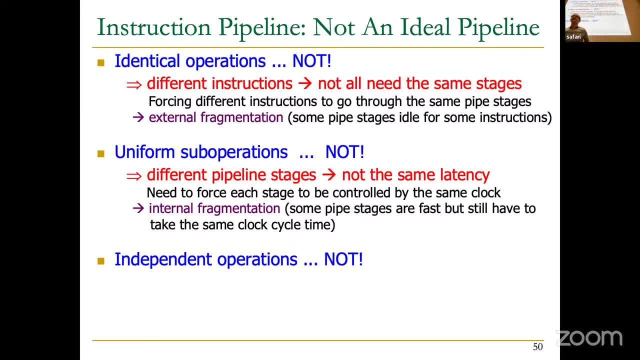 Some stages are much faster, but it needs to take the same amount of time that the worst possible stage takes. OK, And then independent operations. we've kind of said this: Instructions are not independent of each other. You need to detect and resolve inter-instruction dependences. 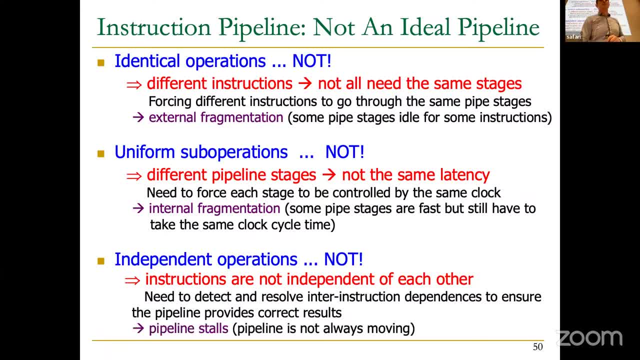 to ensure the pipeline provides the correct results, and this leads to pipeline stalls. Pipeline is not always moving. because you need to stop some instructions, because they're dependent on a value that's going to be produced by an earlier instruction but has not been produced yet. 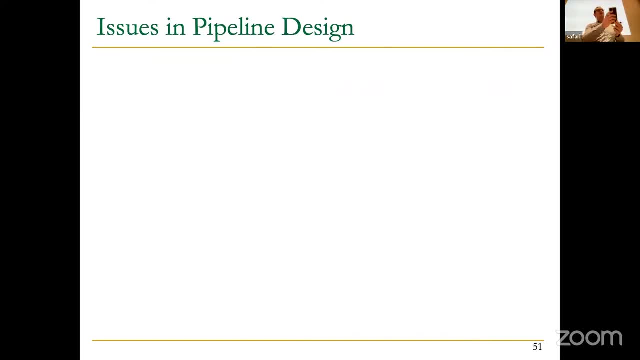 OK, so this brings us to issues in pipeline design. We should have shouted because I didn't realize where we were, But this is a great place to actually take a natural break. Let's be back at 25 past and then we're. 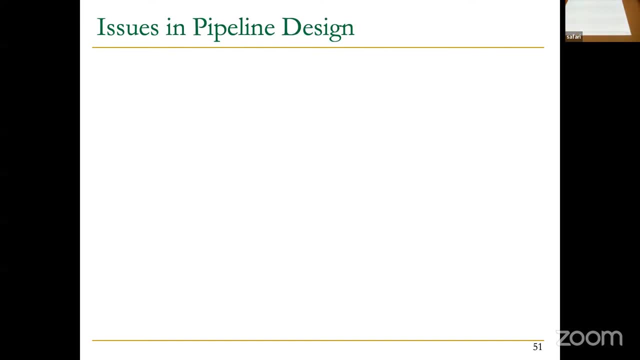 going to delve into some of these really interesting issues. So, in terms of the performance of the pipeline, I'm going to ask you to take a moment to think about the issues that you're going to be discussing, And then I'm going to ask the participants. 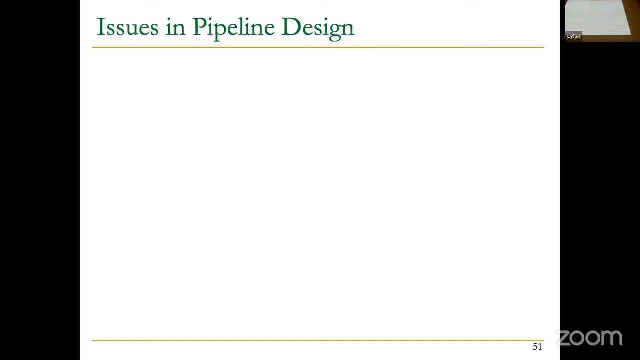 to think about the challenges they have to take on, the challenges that they're facing in their work. And then I'm going to ask you to think about the challenges that you're going to be facing in your work. So I think it's important to think about the challenges. 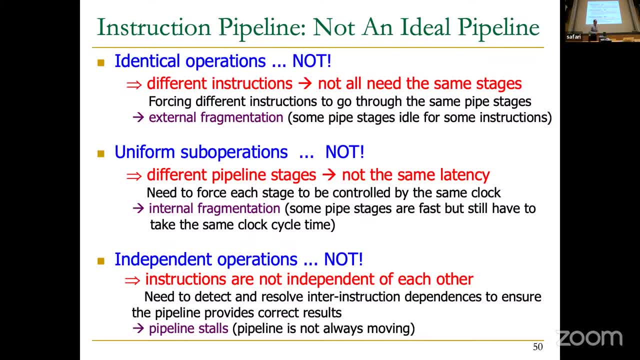 That's good. Okay, so we're going to continue building this pipeline And now, as I said, we're going to go deeper because, as we just figured out, or we have kind of developed over the last part of the lecture, an instruction pipeline is not an ideal pipeline. 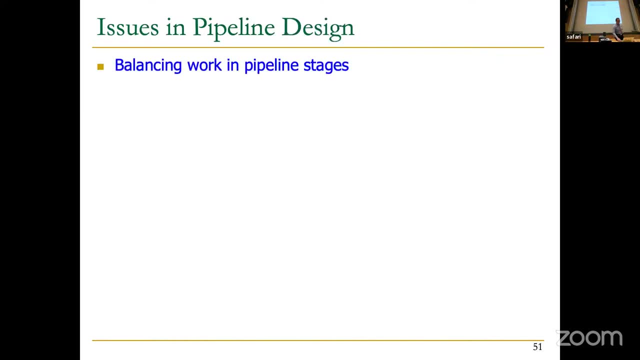 So this brings up a bunch of issues in pipeline design: Balancing the work in pipeline stages, as I mentioned, such that as much as possible, each state does equal amount. we're not going to discuss that. It's not easy. How many stages are there? 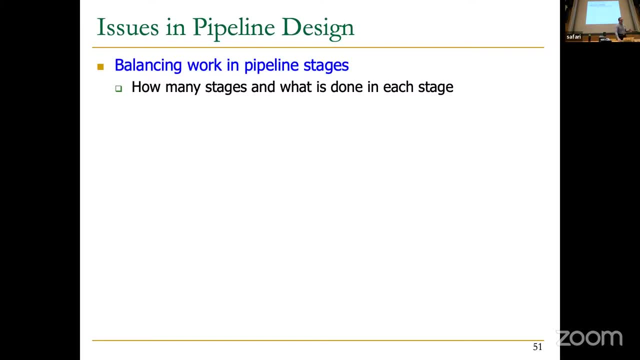 What is done in each stage, That we can discuss more, but we're going to assume some pipeline design to begin with. But in real life you need to do that. You need to balance the work as much as possible so that you don't waste time in a pipeline. 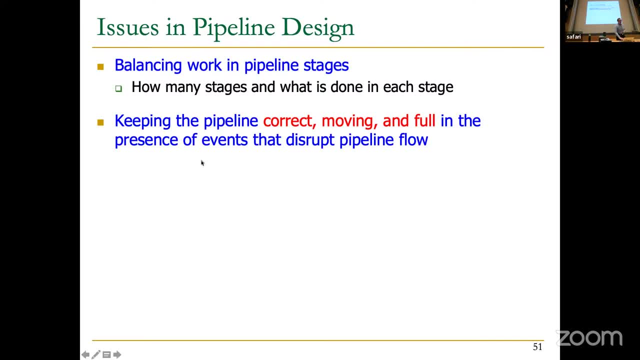 and you don't waste throughput like we have seen. The second part we're going to discuss a lot in today, next week and even when we cover out-of-order execution, because out-of-order execution is going to enable keeping the pipeline full as well. 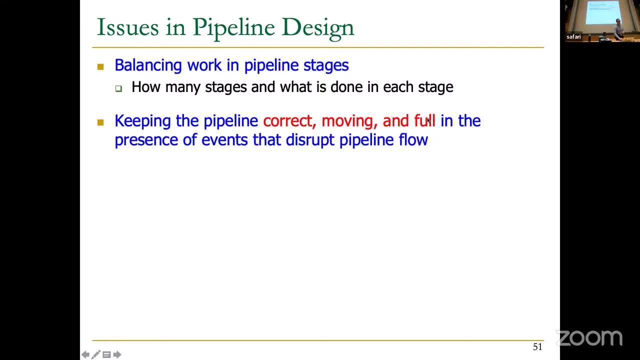 Basically, we want to keep the pipeline correct, moving and full in the presence of events that disrupt the pipeline flow, And correctness is very important, of course, And keeping it correct is really important for a correct execution. You satisfy the semantics of the dependencies between instructions. 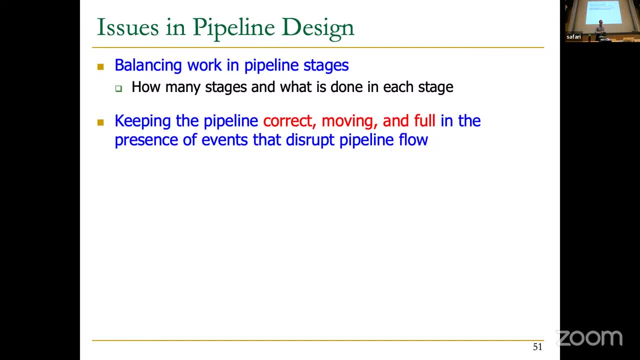 but keeping it moving and full is important for performance, as we will see, Because if you're going to keep the pipeline full, you may have only one instruction finishing every five cycles. again back to square one, basically Even worse, potentially, actually. 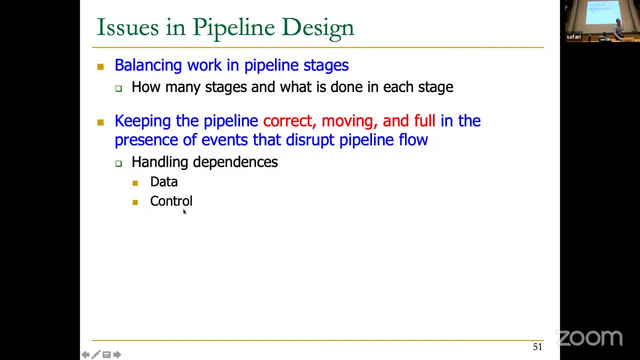 So this requires us to handle dependencies, data and control dependencies, and we're going to actually spend a lot of time discussing these. Decades of work has gone into how to handle these better and better. It also requires us to handle resource contention. 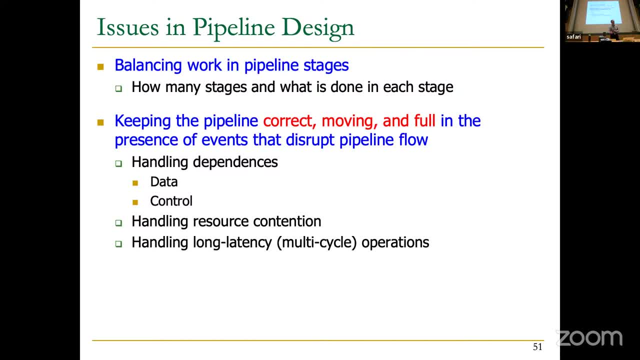 That's going to be important to discuss as well, And especially handling long-latency, multi-cycle operations like memory access, but also multiply instructions, for example. And then we're going to talk about handling exceptional situations. These are called exceptions and interrupts. 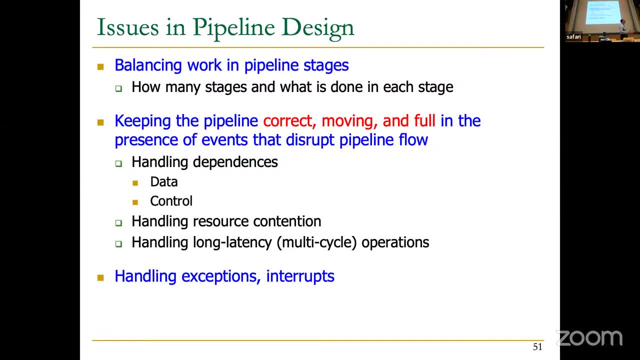 For example, what if your instruction is doing divide by zero? What happens at that point Or while your instruction is executing? what if you get an error in some other part of the machine? That's an interrupt? What if your program gets interrupted for some reason and you need to handle that? 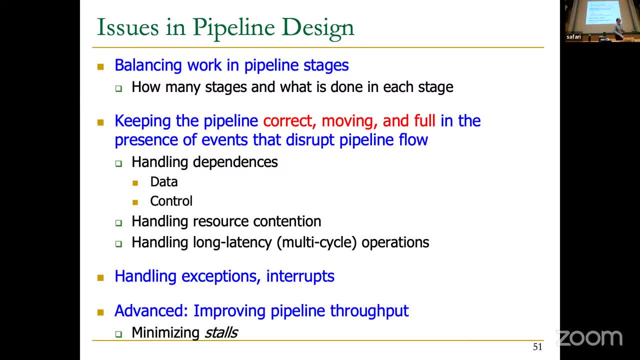 That's going to be the subject of next, next lecture, probably maybe the next lecture, depending on how we finish today. Basically, some of these are related to improving pipeline throughput- How do you minimize the stall that you need to do- And this is a bit more advanced and we're going to talk about that also. 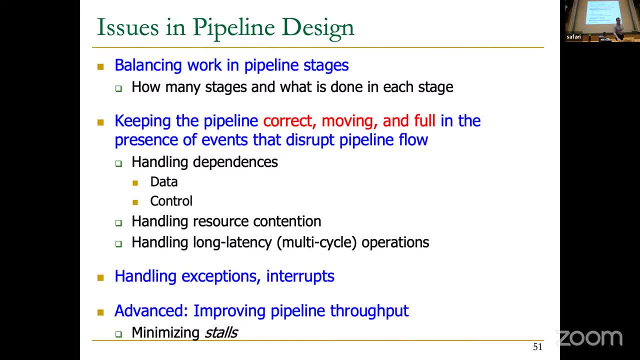 Out-of-order executions. the whole point is going to be improving pipeline throughput as well as overall performance, as we will see. But now let's start with these pipeline stalls. Why would the pipeline stall, And what is a stall? first of all, 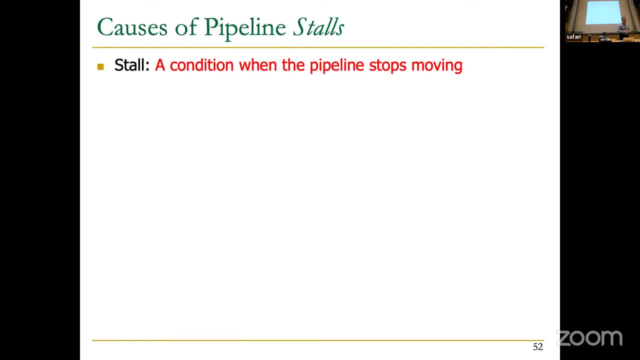 A stall is a condition under which the pipeline stops moving. It could happen due to three major reasons. One is resource contention. One pipeline stage needs a resource the other pipeline stage is using And for some reason you didn't replicate the resource, because it was too expensive or whatever right. 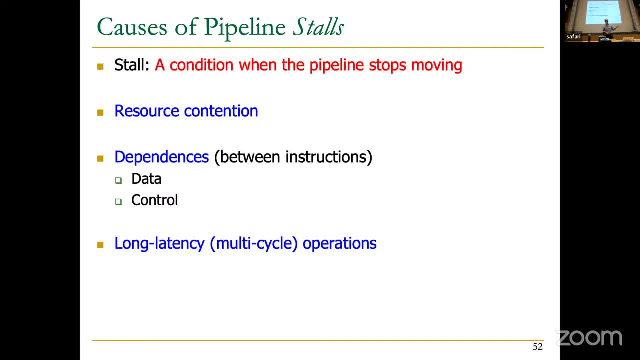 There could be multiple reasons. As a result, one of the pipeline stages needs to wait, And that's a stall right. Dependences can cause this, as we discussed Data and control. dependence between instructions can cause this. One instruction is in the pipeline. 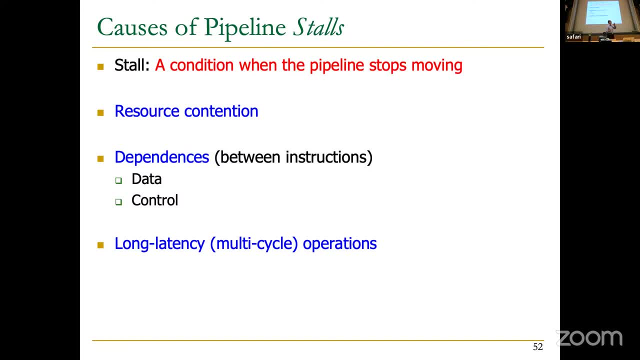 It's producing the value the other instruction needs. So this instruction cannot proceed in the pipeline because it needs to wait until the value is available to it. Control is basically: you have a branch instruction that changes the program counter. What do you fetch next into the pipeline? 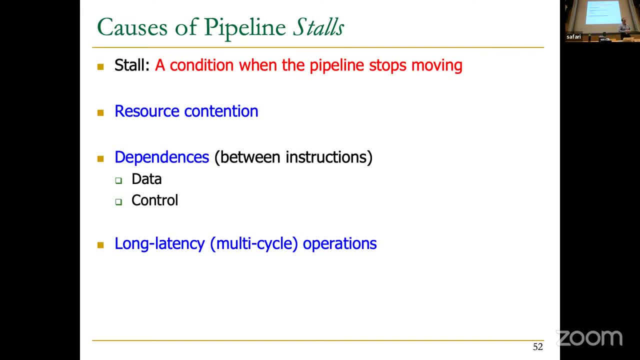 How do you know what program counter to fetch next into the pipeline? So immediately we have a problem in the pipeline actually with control, And long-latency multi-cycle operations are examples of these dependencies. But even when you don't have a dependence, a long-latency memory access stops the pipeline. 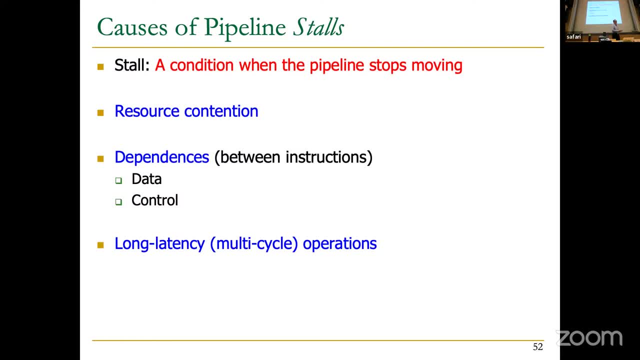 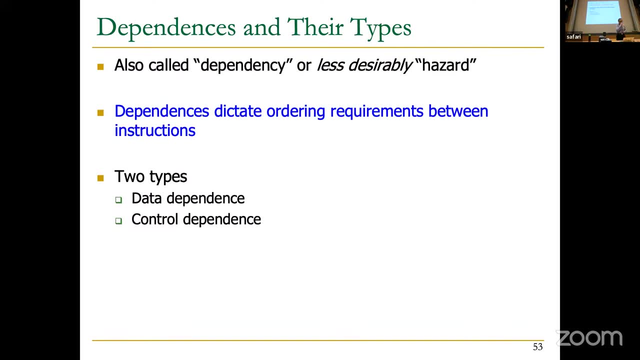 from moving, right, You wait for memory 1,000 cycles, then your pipeline is not moving anymore, right? Okay, So we're going to talk about that. So let's talk about dependencies. Dependences are called dependencies also. 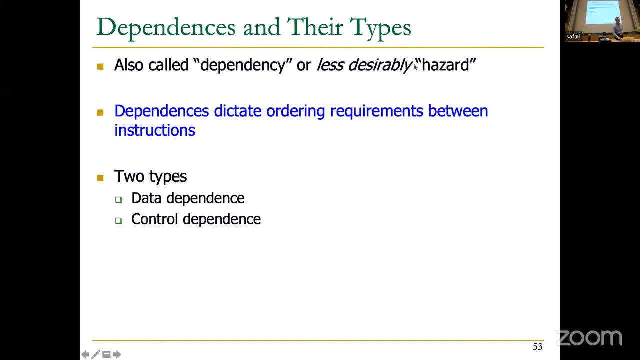 I'll use the word dependencies. Sometimes it's called hazards also. I don't like this terminology, because hazard is a situation that you didn't control, right, But this is something that you know about dependence basically. So dependencies dictate ordering requirements between instructions. 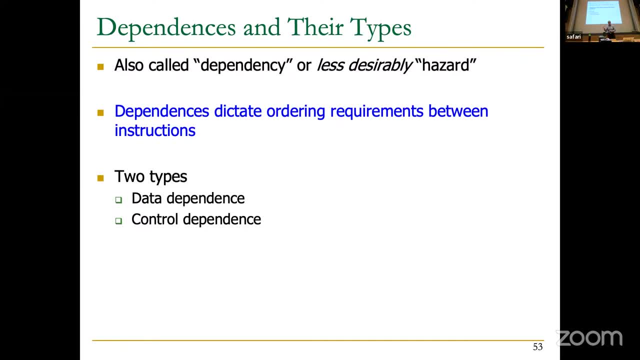 If you don't handle the dependence correctly, it may cause a hazard, That's true. It may cause a problem where you get the wrong value. But dependencies dictate ordering requirements between instructions and there are two types of them: data dependence and control dependence. 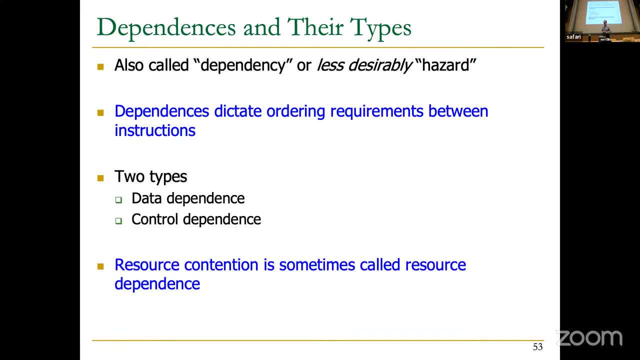 We're going to look at both of them. Some of the books talk about resource contention as a dependence, resource dependence, which is somewhat true, but it's really not the same as a semantic dependence. Basically, it's not fundamental to the program. 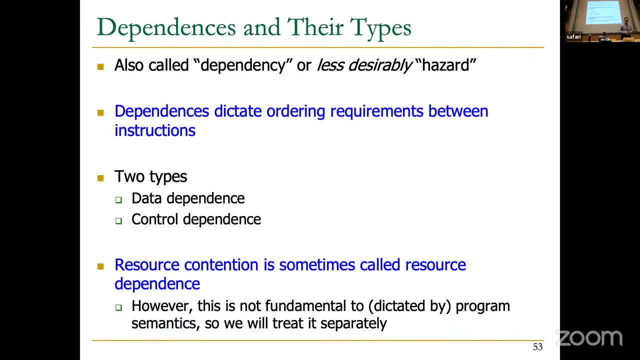 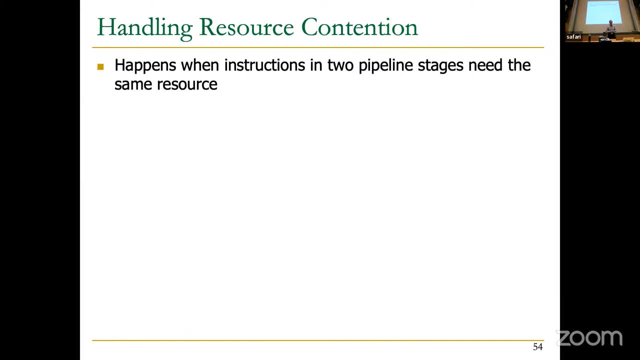 It's not dictated by the semantics of the program. So we treat resource dependence, We treat resource contention separately or resource contention separately. So let's talk about that actually first. Basically, resource contention happens when instructions in two pipeline stages need the same resource. 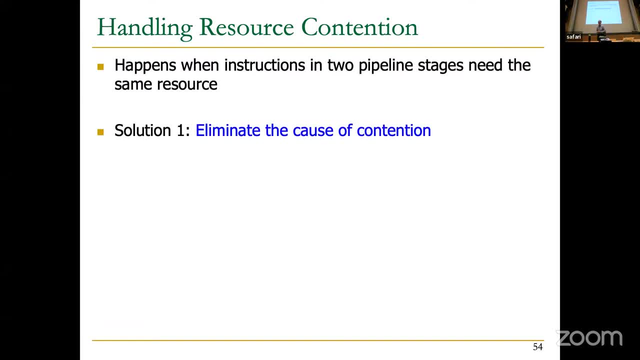 So there are multiple solutions to this. Eliminate the cause of contention right. Replicate the resource, Duplicate the resource or increase its throughput. We kind of did that right. I didn't say that explicitly, but we actually had two memories right. 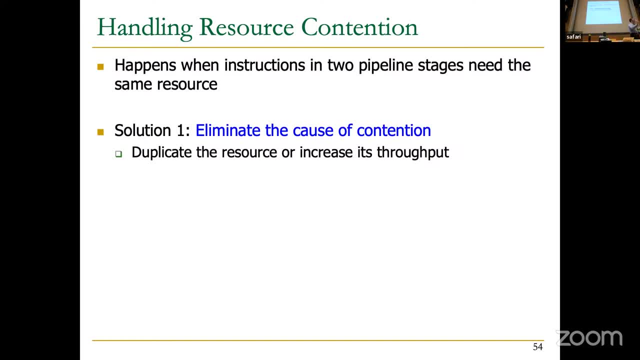 Instruction memory and data memory, like the single cycle. In multi-cycle we merged them together, But in pipeline we actually We separated them again. Yeah, So that's the reason, That's the fundamental reason why we did that actually. 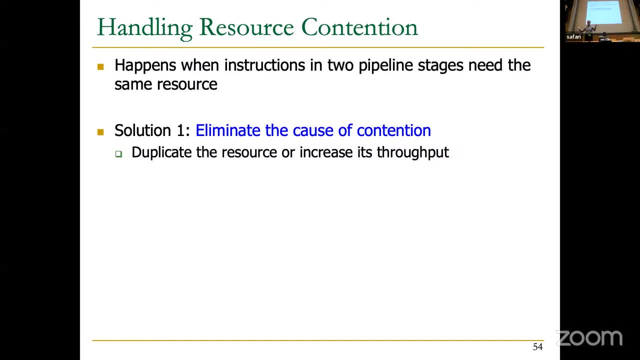 Because the resource is needed by two different stages. So separating them is good. Again, you could have multi-porting. You could have multi-ported them, So you really didn't need to separate them, but it made it easier to explain things to separate them. 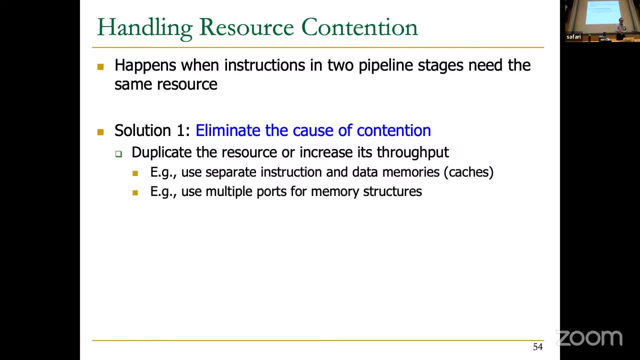 as we discussed last time or one of the last times. So yeah, I just said one of them, Or memory structure is used multiple ports. Basically, multiple ports is different ports dedicated to different stages. It's also eliminated. It's eliminating that resource contention. 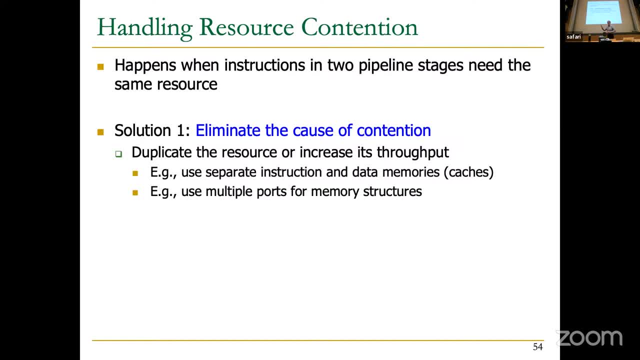 AL use could be another thing, right, If you need the adder, for example, to increment the program counter in fetch stage of the pipeline, and if you also need the adder to execute the instruction in the execute stage, you have to provide two adders now. 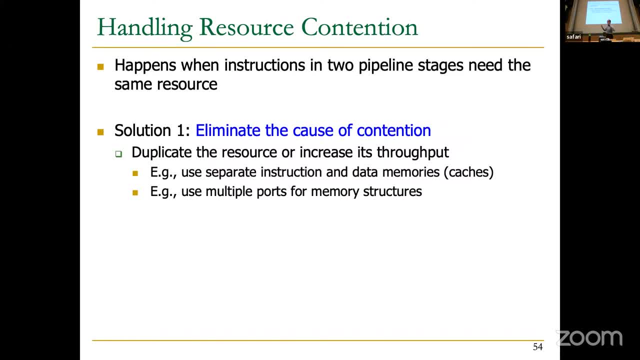 It's very similar to the single cycle design from that perspective. Multi-cycle design could have merged these adders into one, because you're not really actually doing things concurrently, right? In single cycle design it's perfectly concurrent, except you're using all the 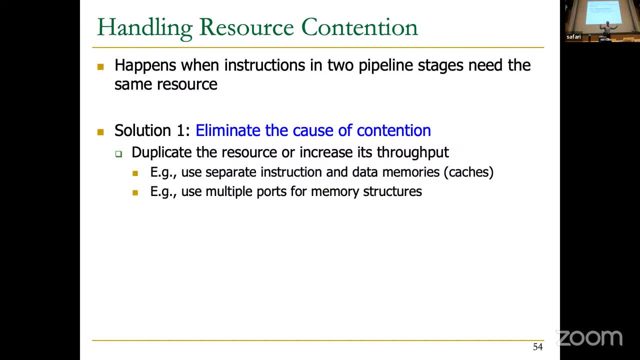 You're using all the different resources for a single instruction. Here again we have lots of concurrency, except we're using the different resources for different instructions. That's why single cycle design and pipeline design are very, very similar to each other. 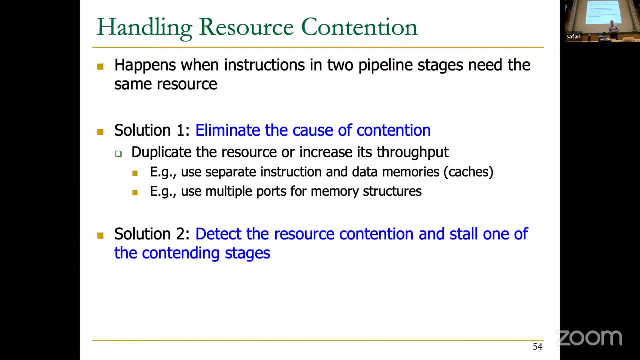 Okay. so we could keep going, but let's move on. The second solution is basically: okay, too expensive to replicate. If it's too expensive to replicate a resource, you put in mechanisms and hardware to detect the resource contention and stall one of the contending stages. 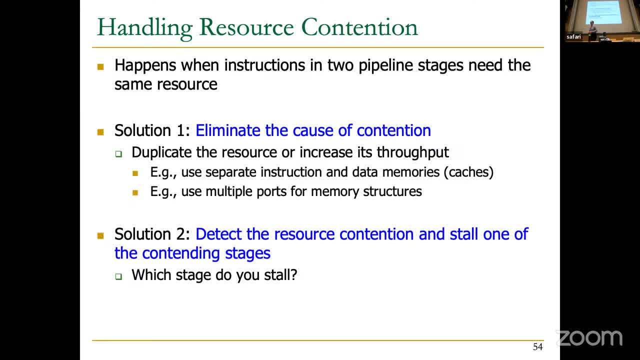 And then the question becomes, of course, which stage do you stall? Well, it makes sense to stall the earlier stage in the pipeline. So, for example, if you had a single read and write port to the register file, don't stall the instruction that's going to write to the register file. 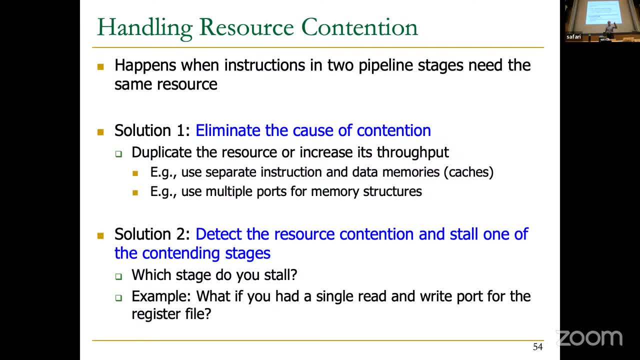 and move out of the pipeline, Stall the instruction that's reading from the pipeline, because they both need the same port. Don't design a pipeline this way. basically, This is a cooked up example, but you may have a single port to the register file. 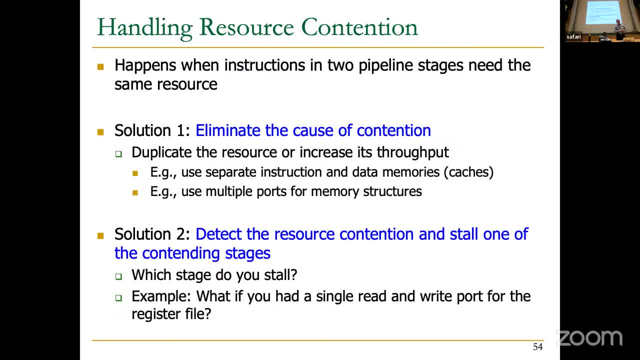 because it's costly for you, whatever reason. So basically, keep the pipeline moving as much as possible and your stall decisions should be based on that. If you stall the one that's reading, it doesn't kind of make sense, right? 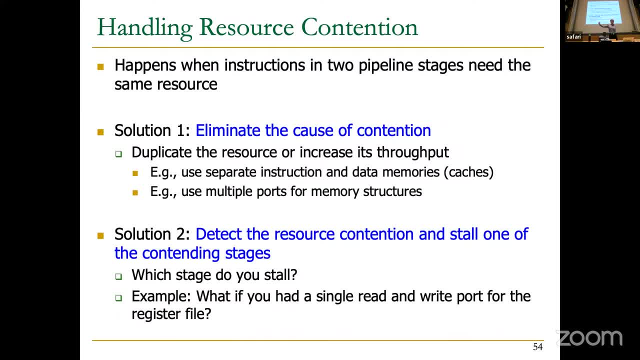 Because you cannot potentially move it to the next stage because the pipeline needs to be moving. So keep the pipeline moving is the principle here in terms of determining which stage you stall in the pipeline. Okay, so that's resource contention. Let's take a look at an example. 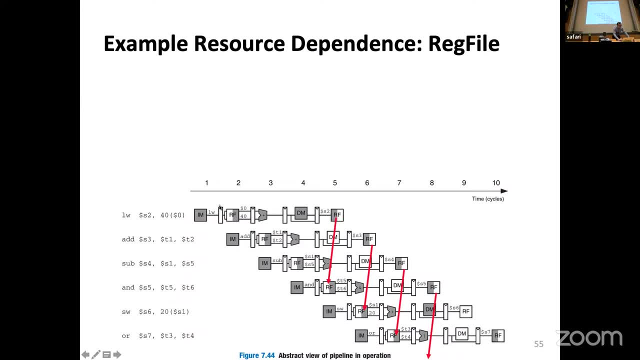 This is an example of resource dependence on the register file. So this is an example of resource dependence on the register file. So this is an example of resource dependence on the register file. This is also from your book, but basically, let's see. 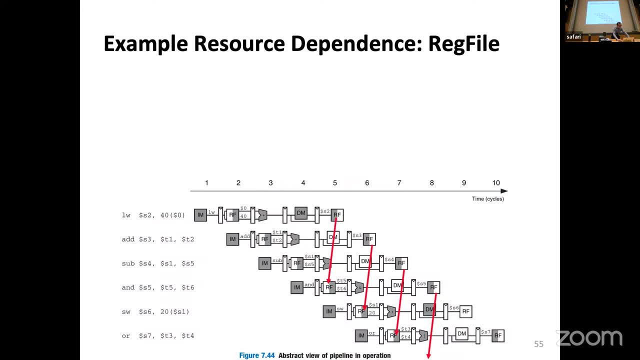 These should be all independent instructions, by the way, or maybe there's some dependence, I don't know. Basically, the register file. No, no, there's some dependence, sorry. So, basically, this instruction is writing to the register file. 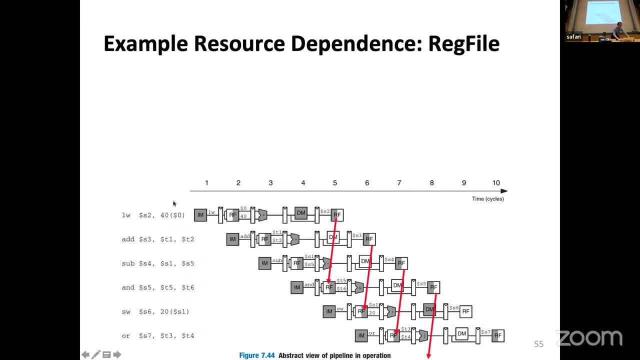 and this instruction is reading from the register file. Actually, there is no dependence between these two instructions, but there may be dependence between other instructions. Don't worry about them for now. How do you handle this? Register file is needed for writing over here and register files read it for reading over here. 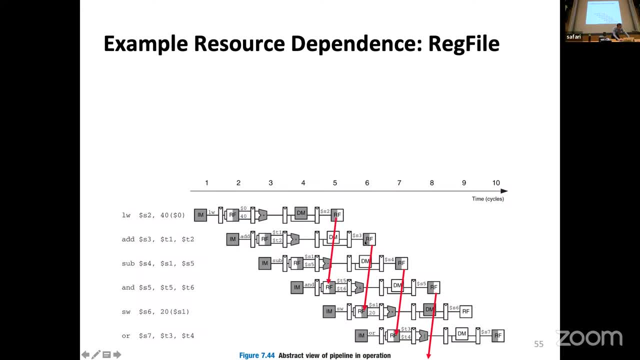 Similarly over here. this instruction is writing to register S3.. This instruction is reading from register S1.. And that keeps happening. as you can see right, This is concurrent, same cycle: Cycle 5,, cycle 6,, cycle 7,, cycle 8.. 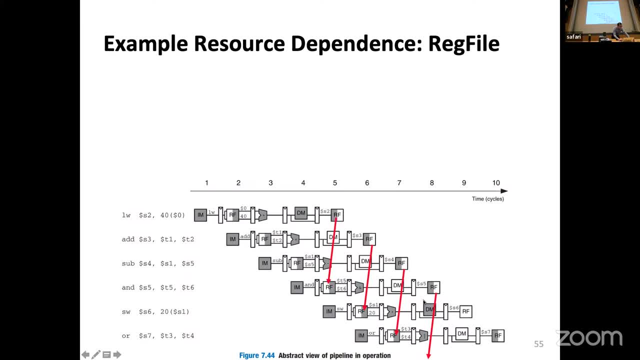 It keeps happening, even though the instruction that's reading at cycle 8 is not shown. So basically, the register file can be read and written in the same cycle. Providing multiple ports help this, But there's also some optimizations that you can do in the register file that we're going to assume. 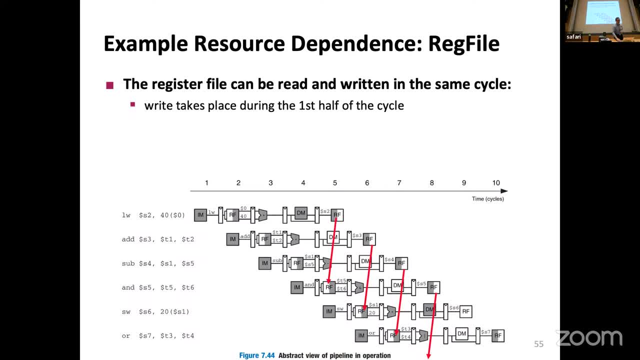 that's going to be useful for data forwarding and making the pipeline moving faster. We're going to assume that write operation takes place during the first half of the cycle, So write finishes in the first half and read happens in the second half. So even if there is a single port in this particular case, 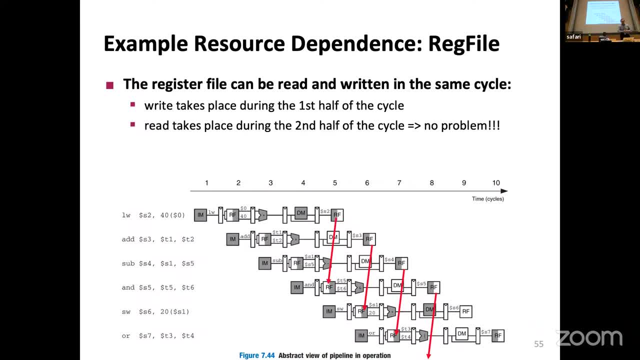 there's no problem. basically, This is one way of solving the problem. This also helps If the first instruction over here is writing to the same register. this instruction is reading right If you design your register file such that this is correct and this is true. 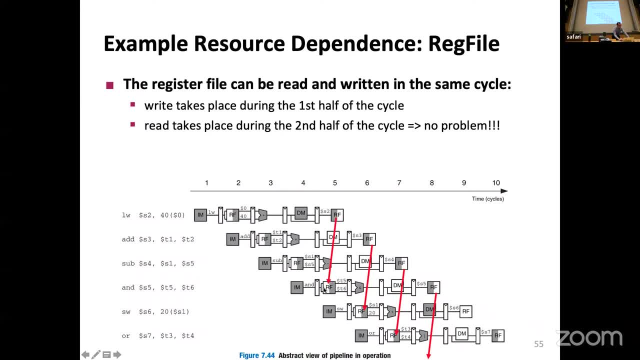 then this instruction can write to register X in the first half of the clock cycle And this instruction that's here that needs that register X can read it in the second half of the clock cycle because it's assumed to be written by the end of the half of the clock cycle. 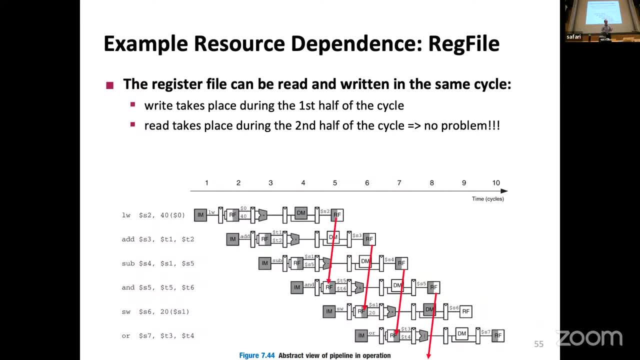 So this is going to help us communicate data values, And this is a form of forwarding, as we will introduce later on- I'm going to get back to this- So this can achieve multiple purposes. basically, This achieves getting rid of some ports from the register file. 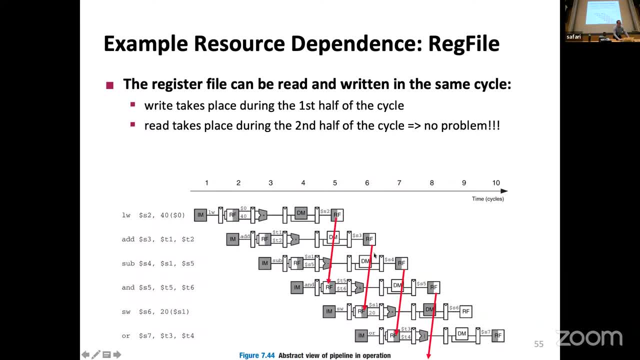 as well as communicating data between instructions that are in the write back stage and that are in the register file, or instruction decode and register file read stage. Does that make sense? This is what we're going to assume in the pipeline design. You don't need to assume this. then you'll need to do something else. 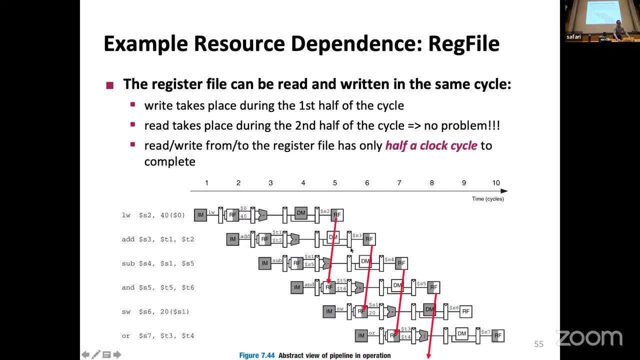 whenever either there's a resource dependence or data dependence. So basically read or write from or to the register file has only half a clock cycle to complete, And we will see this later on again. Okay, now let's talk about data dependencies. 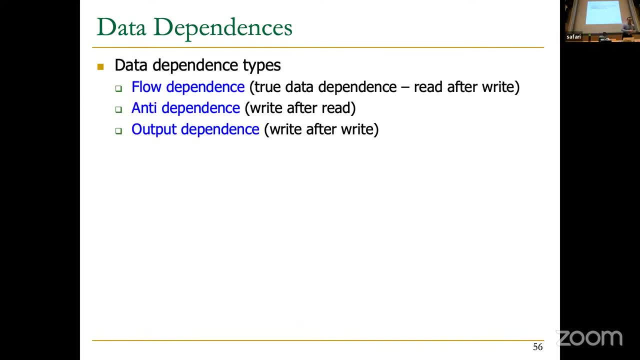 So data dependencies are fundamental to the program- At least well, one of these is fundamental to the program actually, And there are three types. One is flow dependence. It's also called data flow dependence or true data dependence. It's basically when an instruction reads a value that's written by a prior 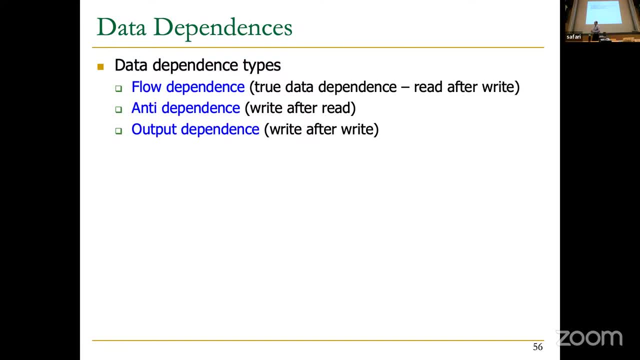 So this is a true dependence, clearly right A prior instruction is the producer of the value that this consumer instruction is reading And you need to make sure this is correctly handled. The other two dependencies are not exactly true dependencies. They're anti-dependences and output dependencies. 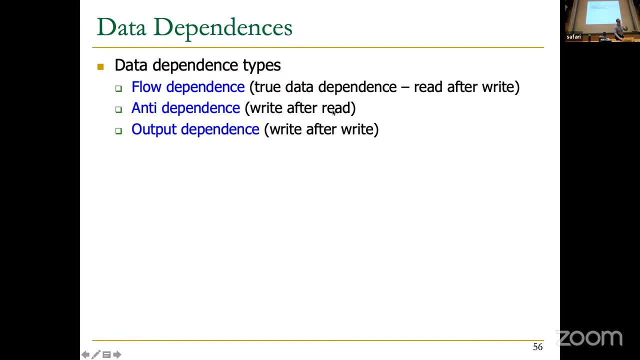 Basically, an instruction writes to a register after a prior instruction reads from the same register. Clearly they're not communicating values. as you will see, An output dependence is an instruction writes to a register that reads what a prior instruction also writes to. 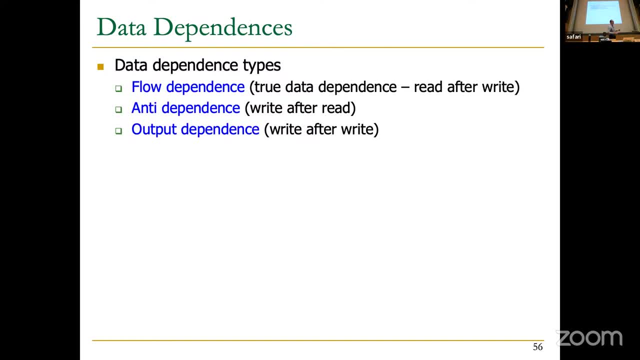 Again, there's no value communication between the instructions here. They just happen to write to the same register. Why would that happen? Because you don't have enough register IDs in your ISAs. right, If you had infinite number of register IDs, you could have not done that. 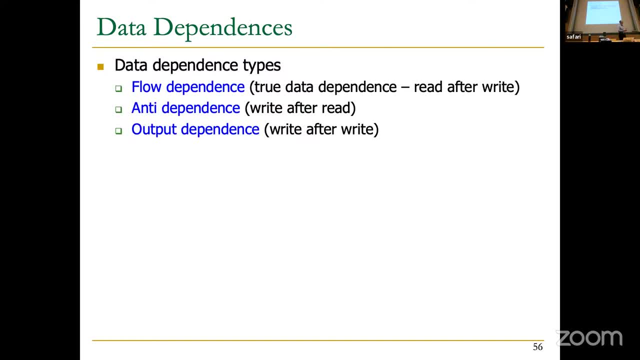 But we're limited by the encodings of the instruction in terms of how many registers we have. So that's why these two dependencies are actually also called false dependencies, but they do affect the pipeline. Okay, which ones cause stalls in a pipeline? 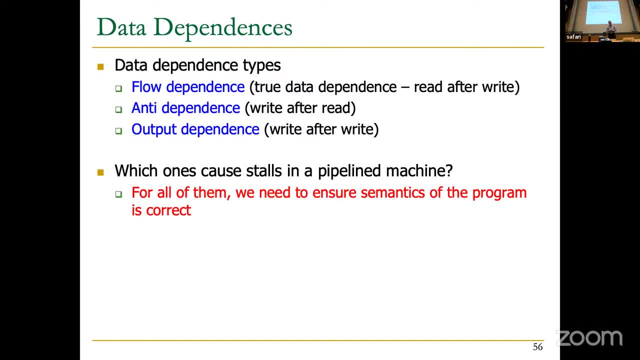 Let me show you. Actually, all of them can cause stalls. You need to ensure the semantics of the program is correct for all of these. So flow dependencies always need to be obeyed, because they constitute true dependence on a value. They're really producer-consumer communication. 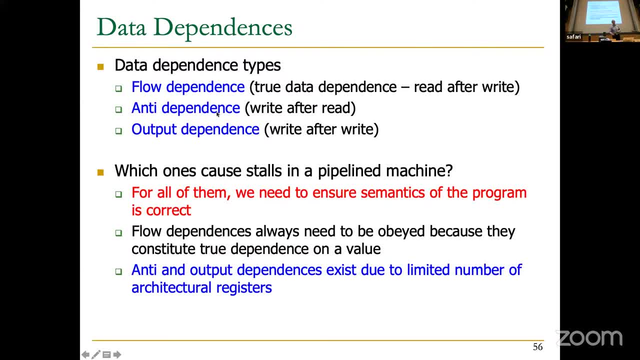 But anti- and output dependencies exist due to limited number of architectural registers. If you had infinite number of registers, you could eliminate all of the anti- and output dependencies, because there's really naming right And we will see that also. Actually, I'll use a picture. 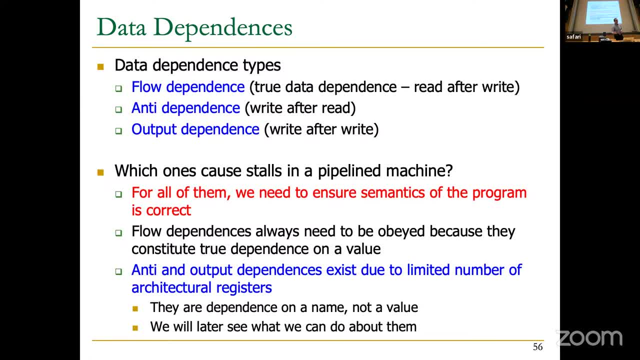 There are dependents on a name, not a value, And we will see later what we can do about them. Out-of-order execution is going to be in part about renaming these registers to some other namespace such that you don't have dependence issues with anti- and output dependencies. 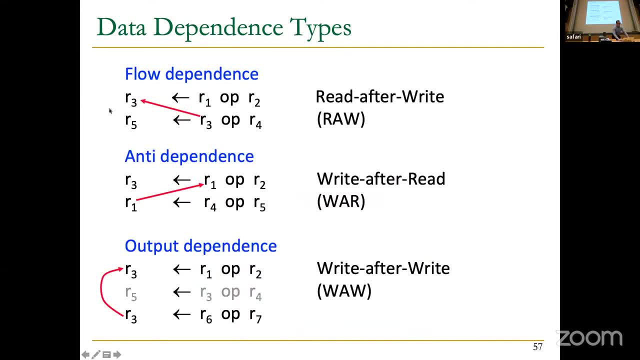 Okay, so let's take a look at this pictorially. This is a high-level operational description. You have this instruction that operates on R1 and R2, writes the results into R3, and you have another instruction that operates on R3 and R4,. 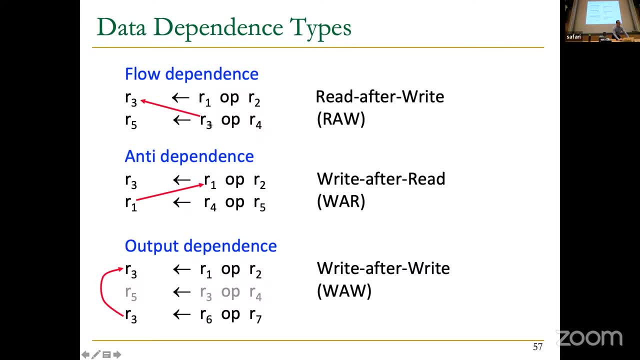 that writes the results into R5.. You can see that the second instruction that comes later in sequence is reading a register that the first instruction is writing. So this is the read-after-write dependence. as you can see, You do a read after a prior instruction writes. 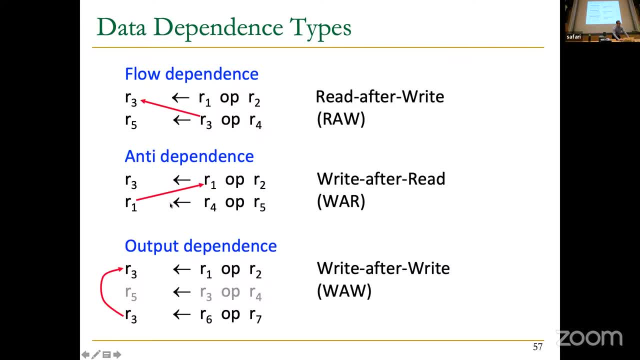 Anti-dependence is exactly the opposite. The later instruction is writing to a register that the prior instruction is reading from, So this is right after read and clearly there's no communication of value Here. this R3 needs to be communicated to this instruction so that it can correctly execute. 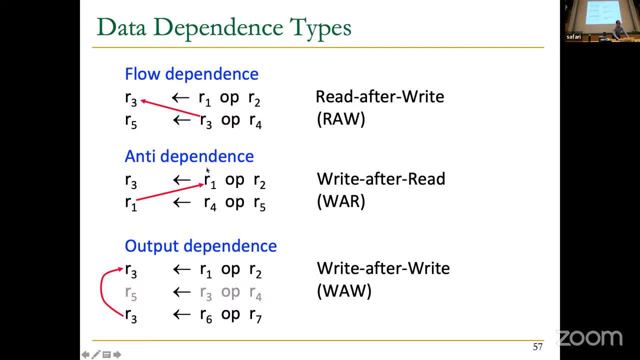 Here. this instruction really doesn't care what the value of R1 was, It's just rewriting that value, right? There's some storage that it's rewriting. You're reusing that storage for some other purpose And you can see that these instructions are completely independent actually. 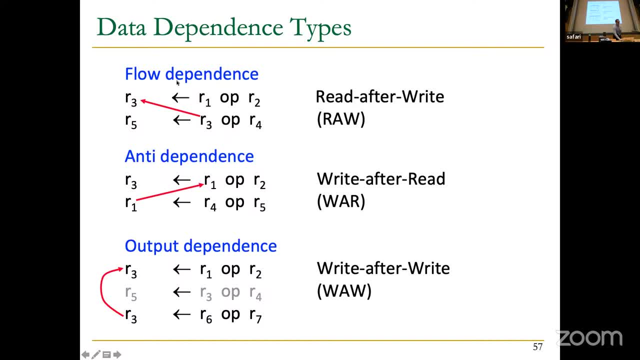 So this is not a true dependence. That's why this is called a true dependence, Whereas output dependence. if you look over here, this instruction is writing to R3.. And this instruction is also writing to R3. And this is called write after write. 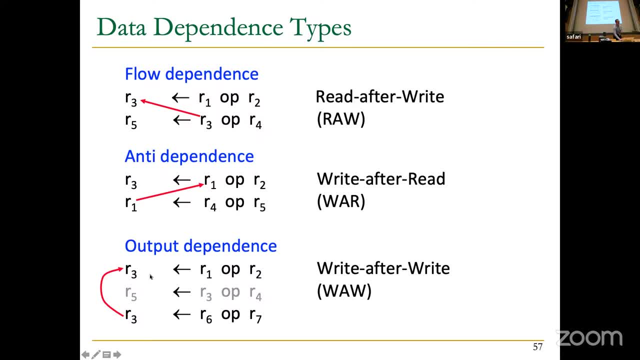 It's also called output dependence And again, there's no data flow over here. This R3 is different from this R3. You're really redefining what R3 contains from a semantic perspective, So the only semantically relevant dependence is really this one. 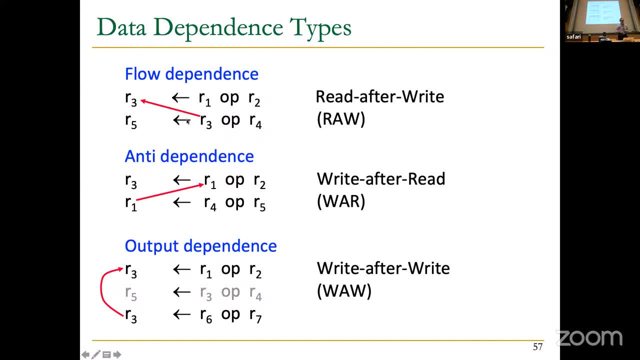 Because it's the producer-consumer between different operations. It basically specifies a producer-consumer or value communication between different operations, Whereas these are. for example, if you had infinite number of registers, you could have easily said: this is R1000.. 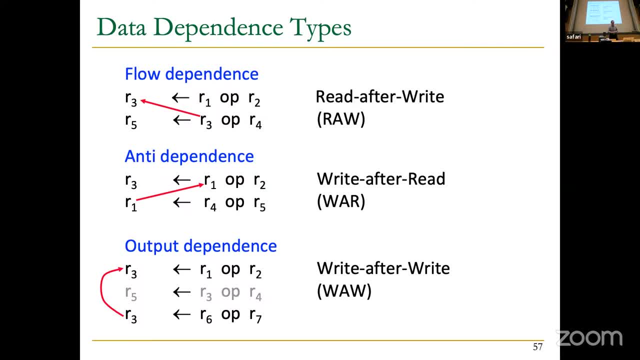 And nothing. everything would work in your program. semantically, Here again you could have said this: R3 is R10000, right Makes sense, right. The reason anti and output dependence exists is because you don't have enough register IDs, register names. 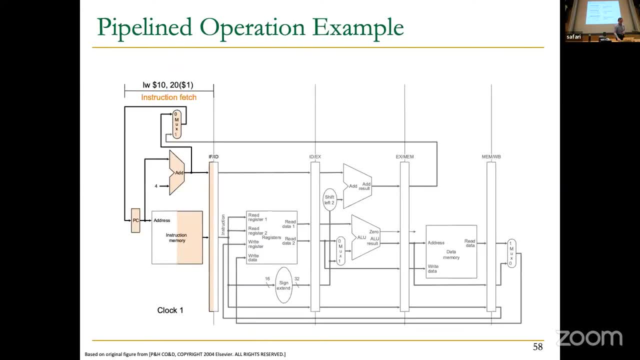 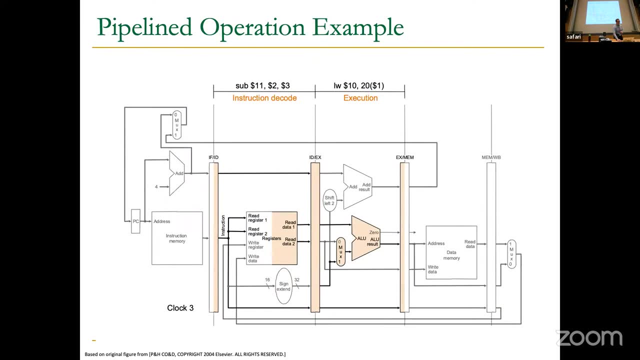 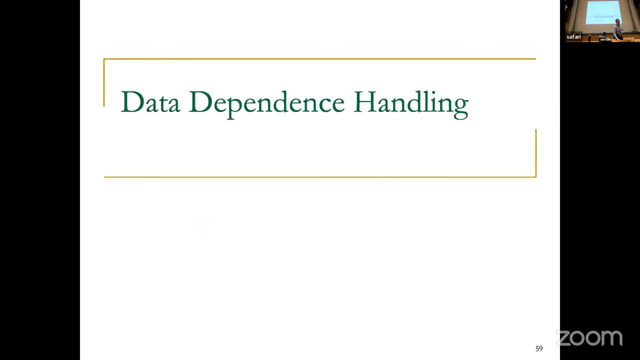 Okay, Okay. so keep that in mind, because we're going to get back to that multiple times. So this is the pipeline operation example we kind of looked at earlier, where load word and subtract were independent of each other. But what if the subtract were dependent on load word? 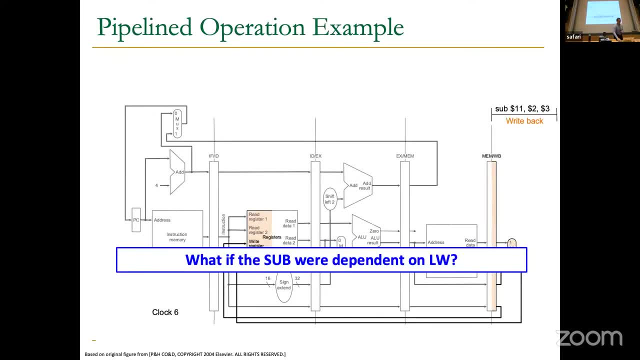 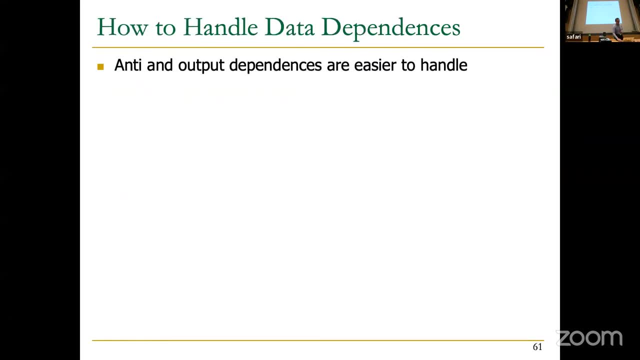 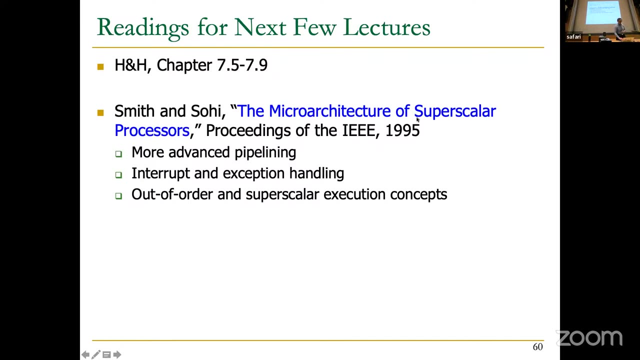 So that brings us to data dependence handling. What if an instruction was dependent on a prior instruction? So this is actually covered in your lecture. Well, not lectures book, a little bit Lectures also, it will be covered soon. But this: the microarchitecture of superscalar processors. 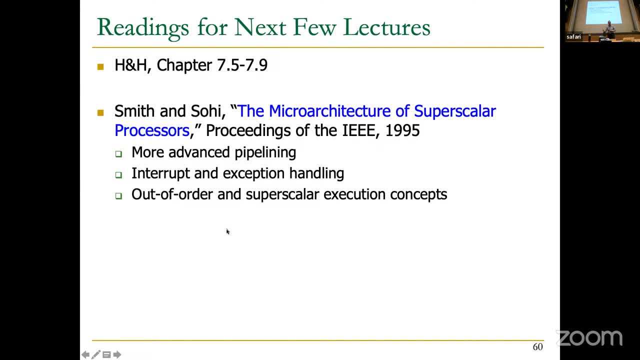 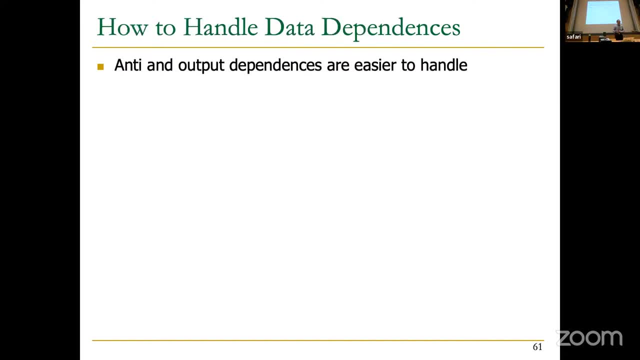 the survey paper that describes how superscalar processors work covers it also nicely. That's why I assigned it Okay. so how do you handle data dependencies? I'm going to focus on true dependencies at this point, because anti and output dependence are easier to handle, as we will see later on. 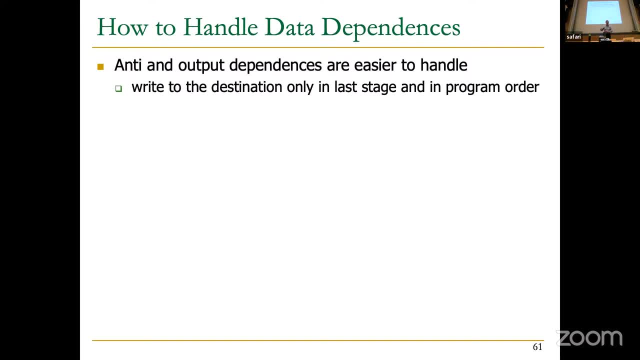 Basically in the pipeline. you write to the destination only in the last stage and in program order. This handles anti and output dependencies, except for dependence detection logic that we will discuss one of them, But we will dismiss that a little bit. So basically, if you actually write to the destination register, 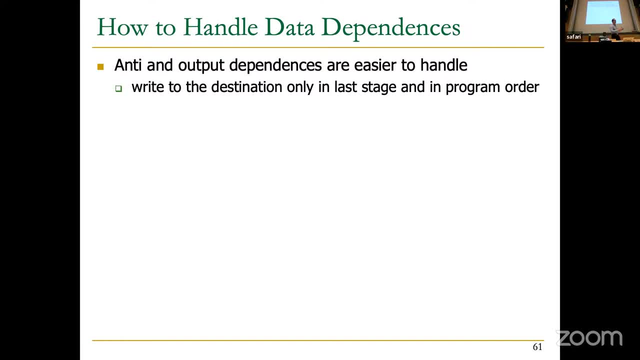 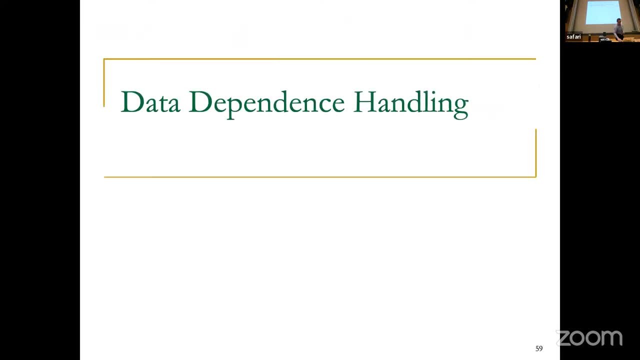 only in the last stage of the pipeline and in program order. you should not have any issues with anti and output dependencies. Basically, don't mess up with the ordering of the writes, Because what really matters with anti and output dependencies is the ordering of the writes. 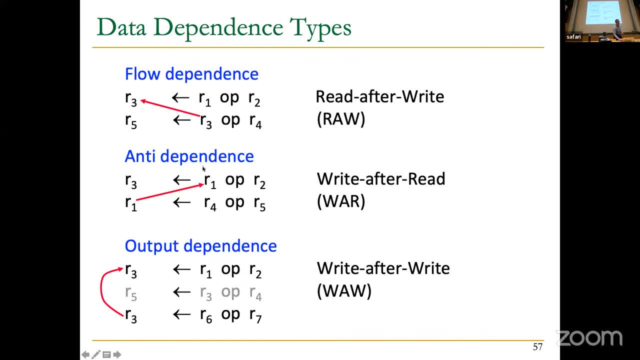 So, for example, this instruction that's earlier, this instruction that's later should not write to register 1, and this instruction that comes earlier semantically or in sequential execution model, should not read the value produced by this register 1.. So that's obvious, hopefully. 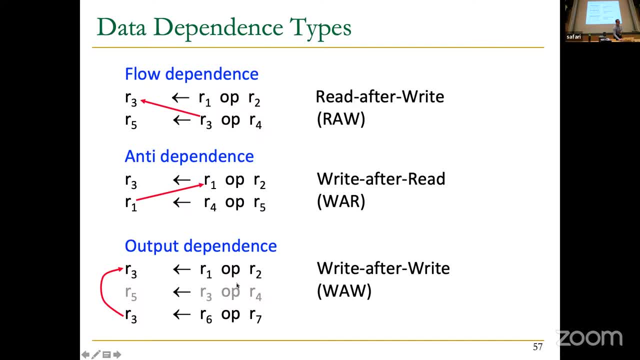 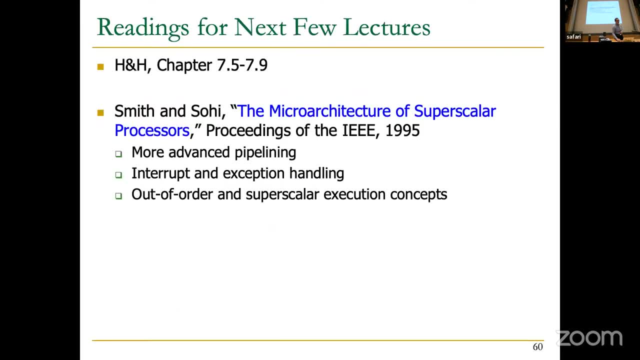 This instruction should not write to register 3 before this instruction, otherwise this instruction will get the wrong value potentially. Basically, don't reorder the writes. and a very simple way of handling, that is, write to the register at the end of the pipeline. 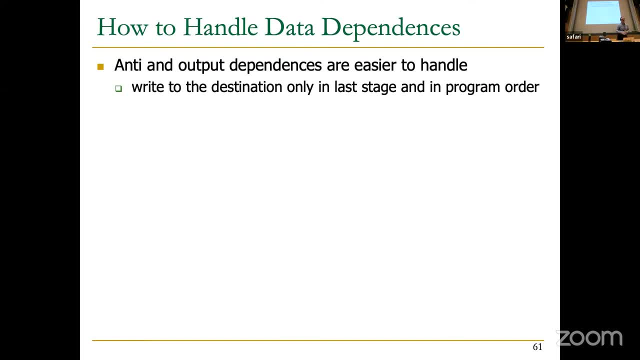 That's why the writeback stage is the last stage. We're going to see more on this when we talk about precise exceptions, because that's where you really need some more care. Okay, so flow dependencies, or these true dependencies, are actually much more interesting and much more challenging also. 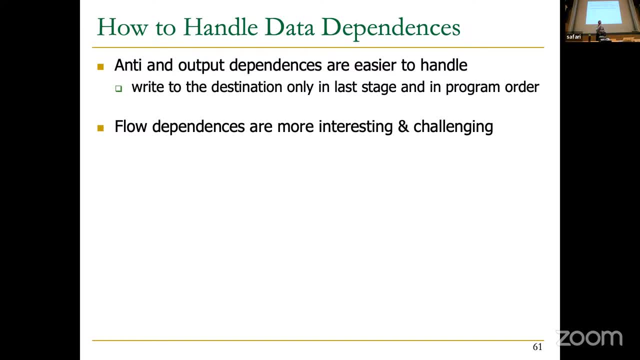 because you cannot eliminate them by renaming the registers, for example, and you cannot eliminate them easily Because they're really there for a reason which is the semantics of the program, And we're going to see six fundamental ways of handling these flow dependencies. 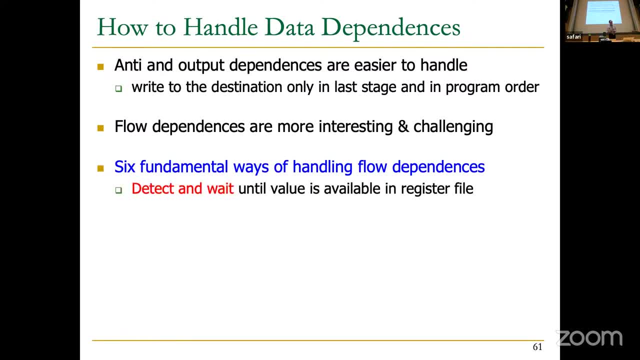 The first four require detection. So basically one is detect the dependence and wait or stall the instruction that needs the value until the correct value is available in the register file. This is the most conservative way of handling them. The second one is detect the dependence and forward or bypass the data. 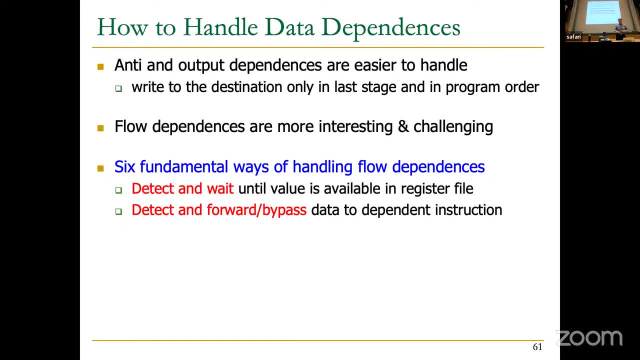 to the dependent instruction before the value is written into the register file. So you have the correct value that's produced maybe in the ALU output. forward that data value to the instruction that needs it once you detect the dependence. Don't wait until the value actually is written into the register file at the end of the pipeline. 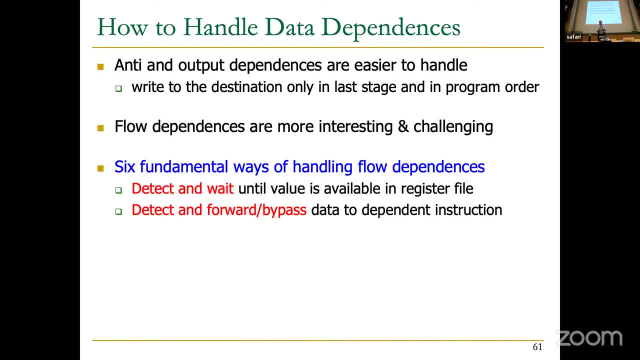 So that's going to improve performance because it's going to reduce stalling of instructions and stalling of the pipeline. Does that make sense? So we're going to see how this is done. So keep this in mind and we're going to be more and more, let's say, sophisticated. 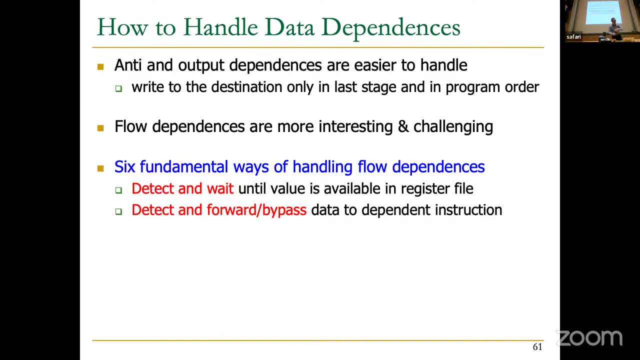 So the only difference between the first and second one is the second one does not wait until the value is written into the register file or register is written into the register file. The third one, which we're also going to see, is detect and eliminate the dependence at the software level. 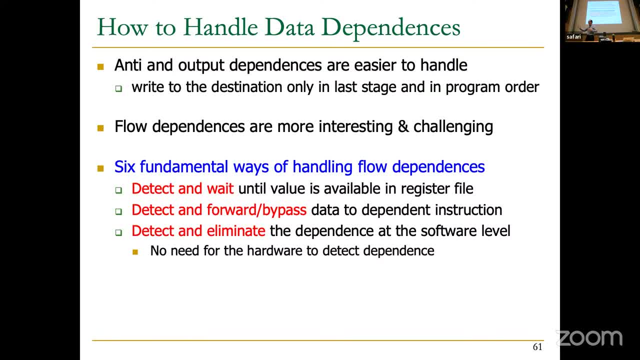 Basically, the software figures out which instructions are dependent. It also has knowledge of the pipeline structure. It also knows what's happening in the pipeline. So now the software is very tied to the microarchitecture. It could be the programmer, It could be the compiler who's doing this. 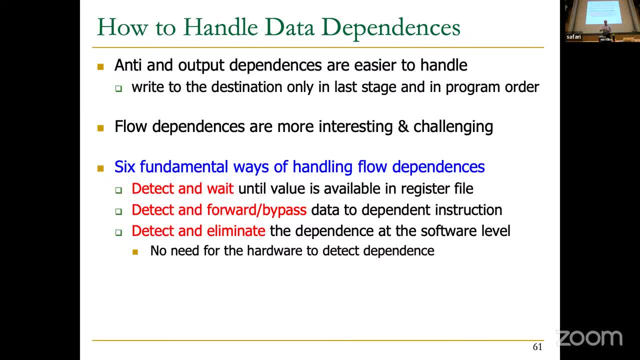 It basically says: I'm going to insert some instructions such that you will never get the wrong instruction, You will never get the wrong value, Or I'm going to reorder the instructions such that no instruction will get the wrong value. Semantics will be obeyed correctly and we're going to see that. 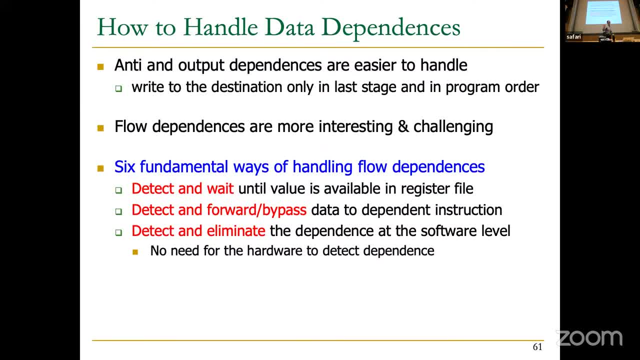 The easiest way to do this is inserting no instructions, no operations, such that the instructions are separated from each other enough. We're going to see this in out-of-order execution. You detect the dependence and if an instruction is dependent on another instruction, 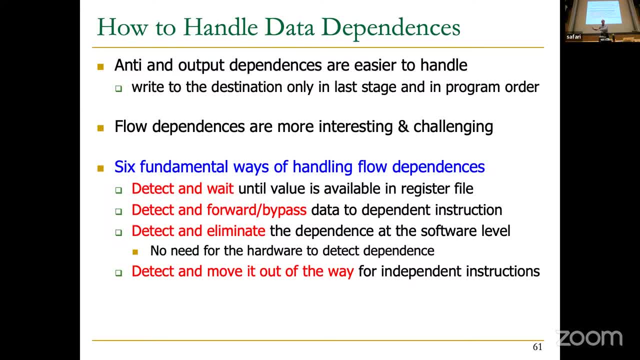 you move it aside such that it doesn't stall the pipeline. That's going to be more advanced and this is out-of-order execution And you can do more sophisticated things like: okay, the value is not available yet, Why don't I just predict it? 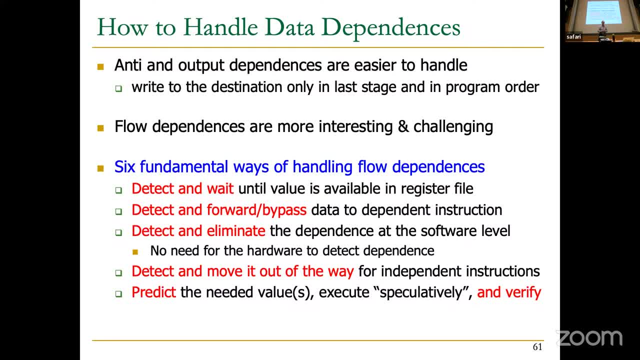 I just predict that this register will be zero And use that prediction, Execute dependent instructions speculatively and verify whether you did the correct thing. Now, if you did not do the correct thing, you'll need to handle it so that no instruction gets the wrong value. 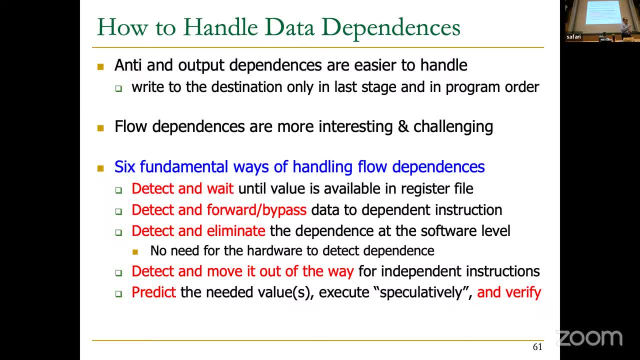 So we're not going to talk a lot about this, but I just wanted you to know that this is an approach. We may talk a little bit more. This is more sophisticated, as you can see, And finally, we're going to see do something else. 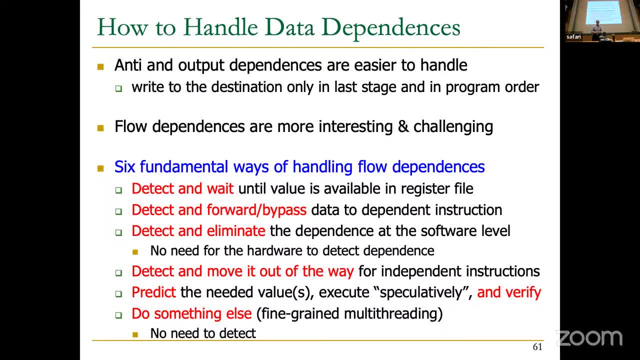 Basically, is there a dependence? Well, make sure there's no dependence between the two instructions that are Well, between any of the instructions that are in the pipeline. One way of making sure of that is making sure that the instructions belong to different programs. 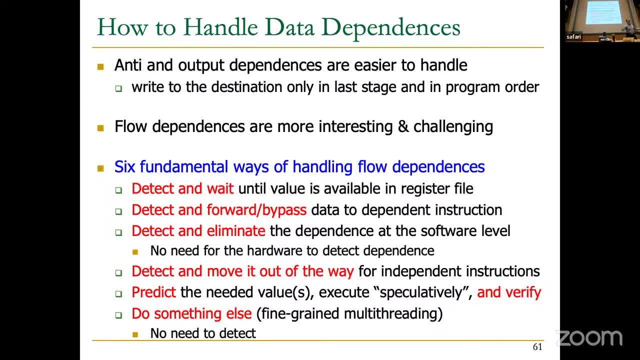 that have nothing to do with each other. So use the pipeline such that you execute an instruction from a different program in each stage of the pipeline, And this is called fine-grain modeling. This is called fine-grain multi-threading, and GPUs are great at doing this today. 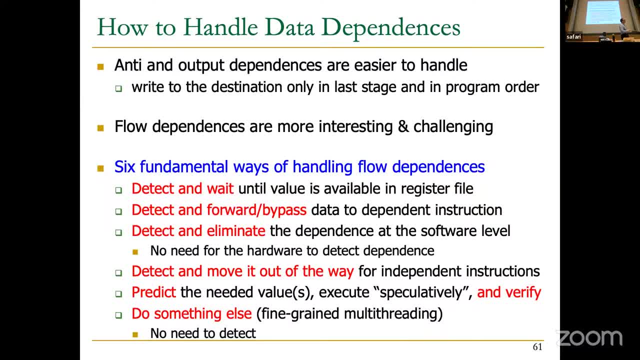 GPUs are actually very powerful because they heavily exploit fine-grain multi-threading. They have tens of thousands of threads that are in multiple different pipelines. This way, you basically don't need to detect anything. It's kind of a cop-out, but it works if you have many, many threads. 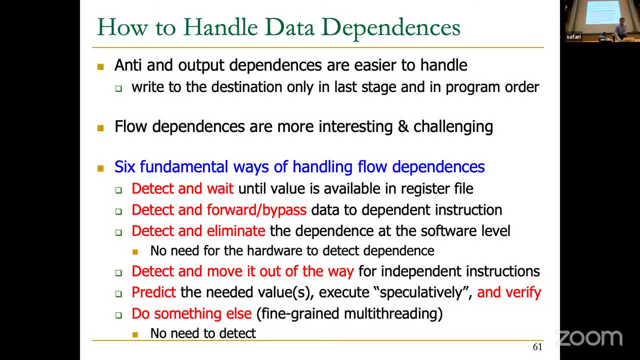 It doesn't work if your goal is to improve the performance of a single thread. Okay, so all of these require detection. Well, all of the four at the top require detection. Let's take a look at how this detection is done. So this was an overview of how we handle things. 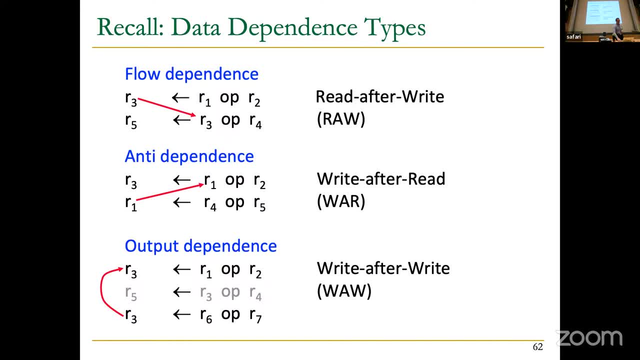 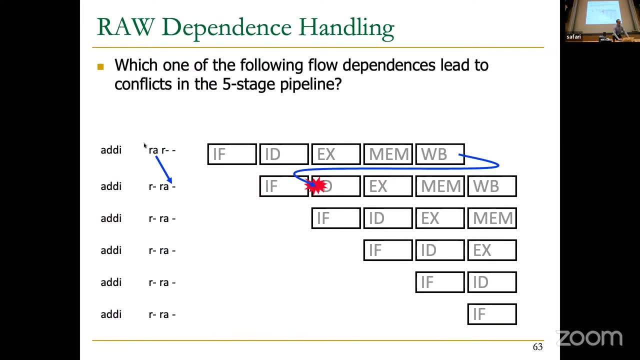 So we're going to go into more detail into each of these techniques. So, recall, we want to detect the data dependencies, So let's take a look at how this exhibits itself in the pipeline. So here we have an example. This ad is writing to register A. 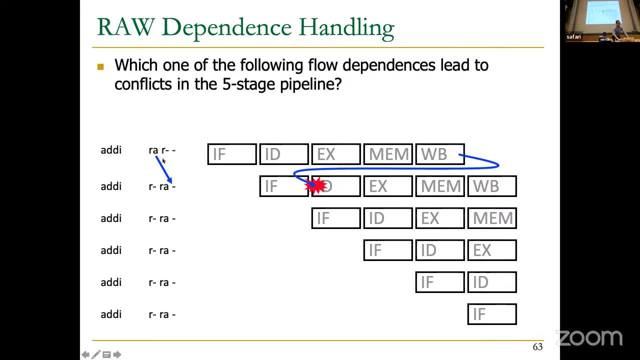 And it so happens that all of the other ads that come later are reading from register A. Now this is the pipeline. Technically, this ad is supposed to write to the register file by the end of the writeback stage. Now, if you don't do anything about this, what happens is this ad will read from register A, an older value that was in the register file. if it keeps going, 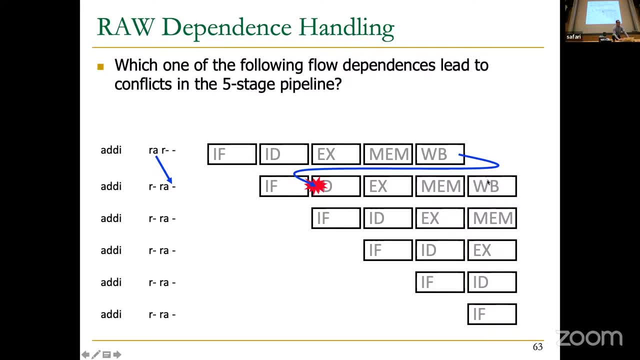 And it will execute. it will write back a wrong value, potentially wrong value. probably a wrong value in the writeback stage Makes sense, right? So you should not let this ad go until it reads the correct value. It gets the correct value from the first ad. 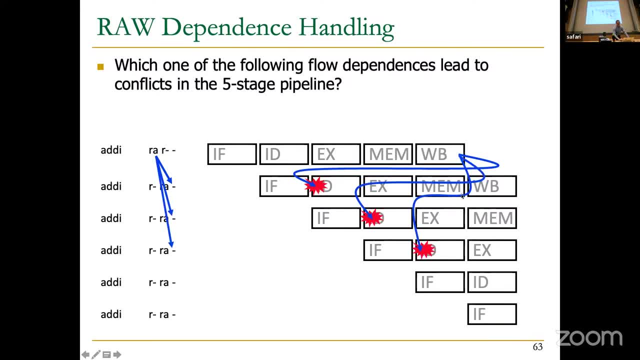 And that's true for other ads also. actually, Basically, the only ad, well, the first ad that will read the correct value of RA is this one, Because there's a separation, There's enough separation between this first ad that's writing to RA and this ad that's reading from RA. 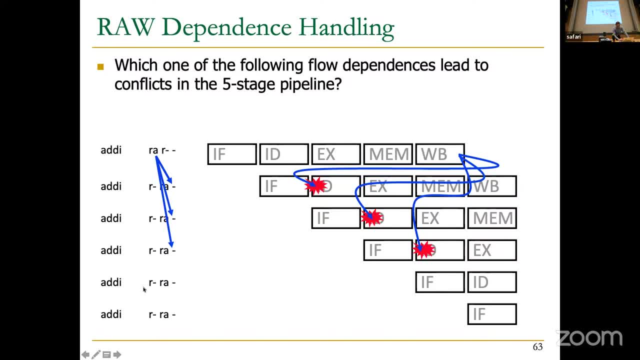 So if you look at this, This ad over here starts reading from the register file in this instruction decode stage, And at that time the register file is properly updated because this ad finished. So now you can see some ideas over here, right? 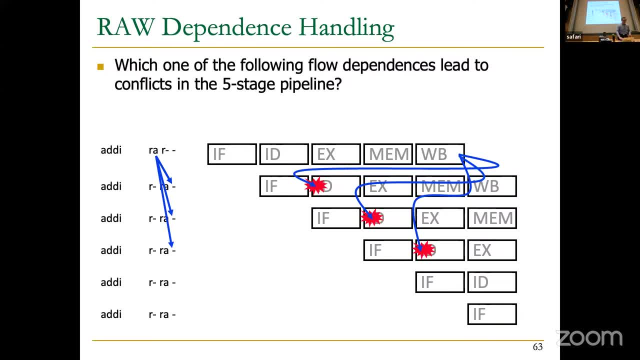 You need to separate these instructions that are dependent on each other in some way, Meaning this ad actually should not have read anything until the register was updated, So you should have waited for three cycles until this ad went through the pipeline, And this ad should have stopped in the pipeline. 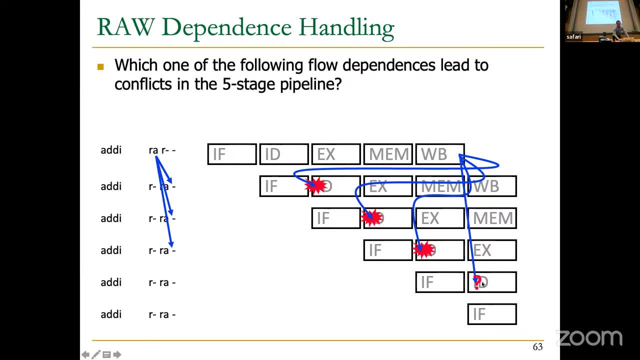 Okay. So basically, hopefully this will get the right value. There's no question mark over here. Okay, Now, of course, this could have gotten the correct value also if we actually did what I just suggested. If this ad actually writes in the first half of the clock cycle: 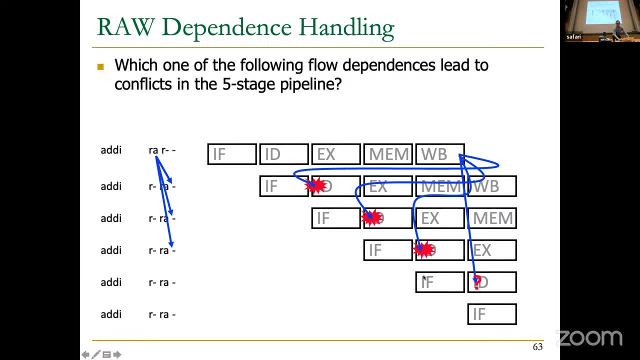 And this could read in the second half of the clock cycle. Actually, you just needed to wait only two cycles, right? So we're going to assume that later on. Right now, I'm going to assume that you wait until the data value is written into the register. 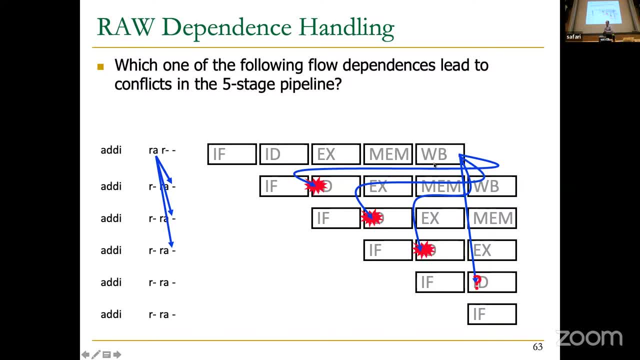 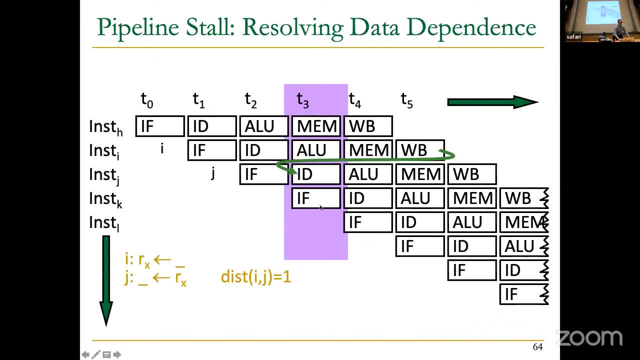 And you don't have this, let's say optimization that you do in the register file, Because that optimization is actually very much similar to data forwarding, if you will. Okay, So let's take a look at how you dissolve the pipeline. data depends. 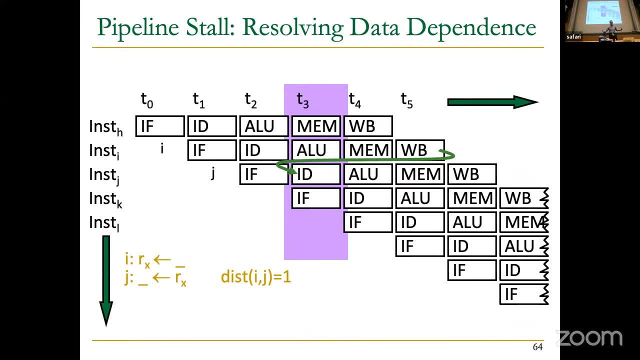 Based on what I said, you need to provide distance between dependent instructions, right? So if an instruction is writing to a register and a later instruction is reading from the register, and if the pipeline structure looks like this, a distance of one will not work. 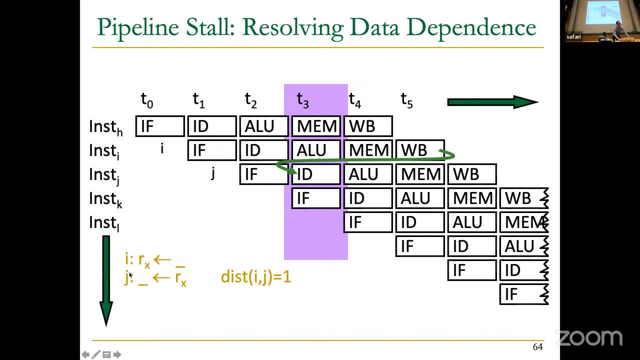 Basically, this instruction should not come immediately after the instruction J. should not come immediately after instruction I. This is distance one. basically, This is I, This is J. So I is writing to write back register here And we should not be reading over here. 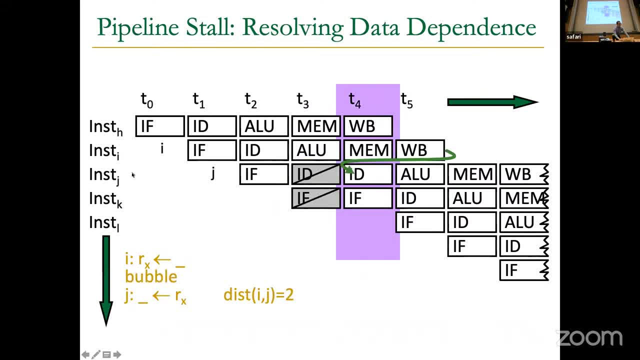 So let's add some more distance. Let's make distance two meaning stall or wait. this instruction J. So it's in fetch stage. Wait, We make it wait in the instruction decode stage. One more cycle. So let's take a look. 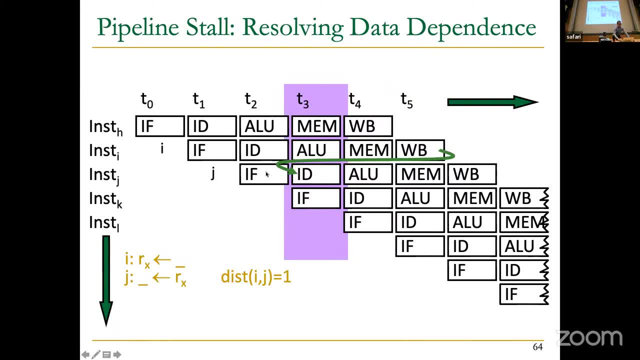 This was: we're not making it wait. The pipeline is flowing, But we figure out there is a dependence. Make it wait Just one more cycle. Well, we're still wrong. We should make it wait longer, right? So this is basically stall description over here. 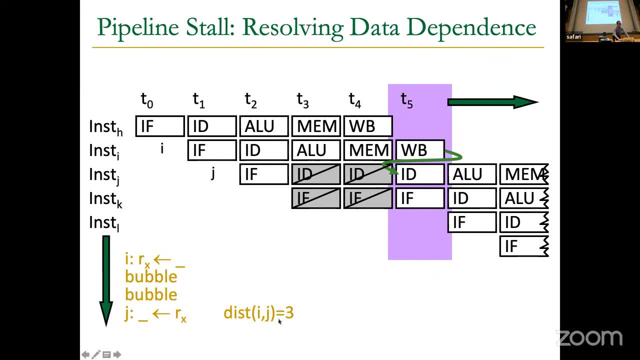 So let's make it longer, Let's make it wait two more cycles. So now our distance is like this: Well, we're still wrong because, based on the assumption, the value of the register that I is writing to is available at the end of the cycle. 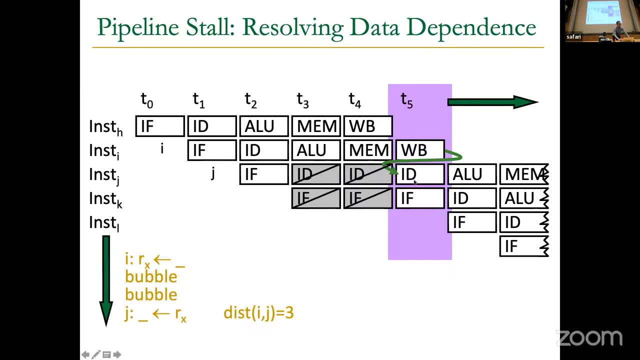 Whereas we're reading that register, A wrong value in that register during the cycle. So concurrently, this is writing and this reading, So you will get the wrong value. So you really need to make the distance four, meaning a short three bubbles. 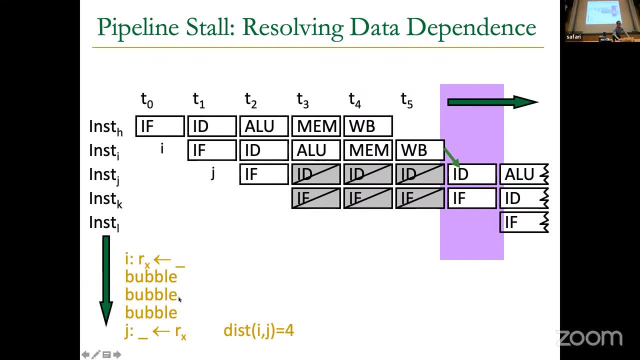 Three stall cycles, in other words, such that this dependent instruction gets the correct value. Assuming this pipeline structure and assuming that the correct value in the register is correct. Assuming that this pipeline structure and assuming that the correct value in the register is correct. 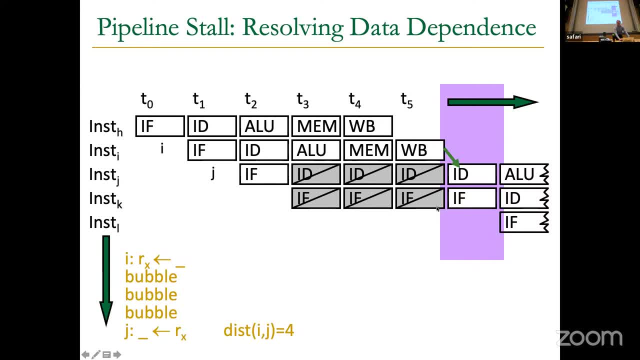 the register file is available at the end of the write. backstage Makes sense, right? So this is the idea of a bubble or a stall, basically. Basically, what we do is if we detect this dependence- and we're going to talk about how to detect that dependence- 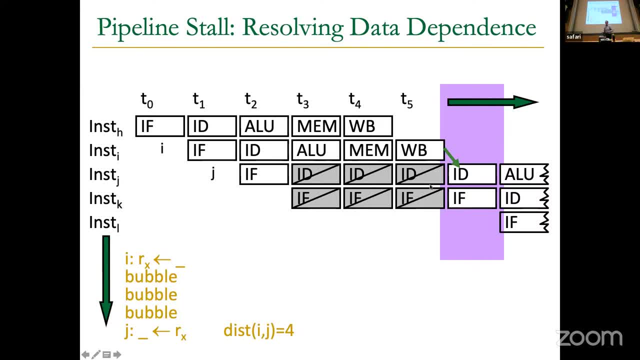 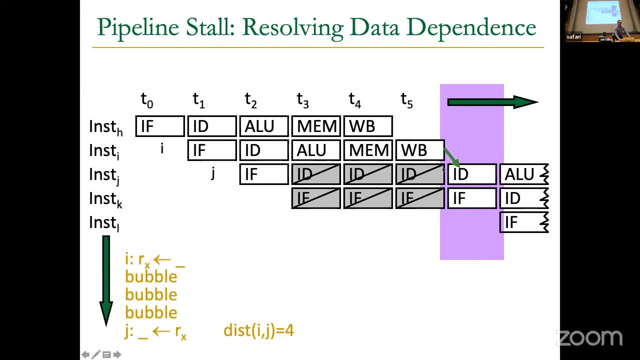 until the correct value that it needs is available in the register file. Or you could take another view and say: compiler can insert these bubbles, assuming it knows what's going on in the pipeline. Basically, compiler adds some no-ops, So the next instruction that comes after. 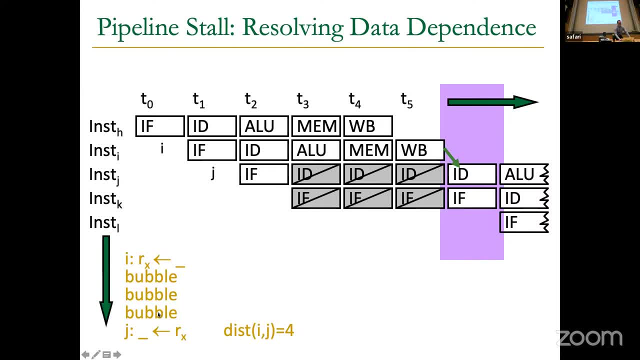 this instruction is a no-op, And the next instruction is also a no-op, The next instruction is also a no-op, And then the dependent instruction comes. That way the compiler orchestrates the scheduling of operations on that pipeline if it knows the pipeline structure. 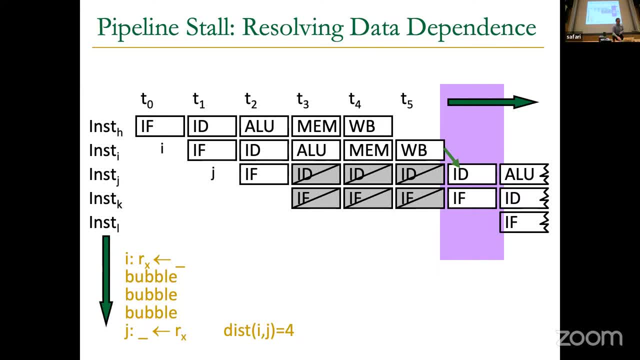 Makes sense. right, You can do this as an assembly programmer also, But if you do it in hardware it's nicer because the compiler or the software doesn't need to know about the pipeline structure, which is a good idea in general. So basically, to more properly define: 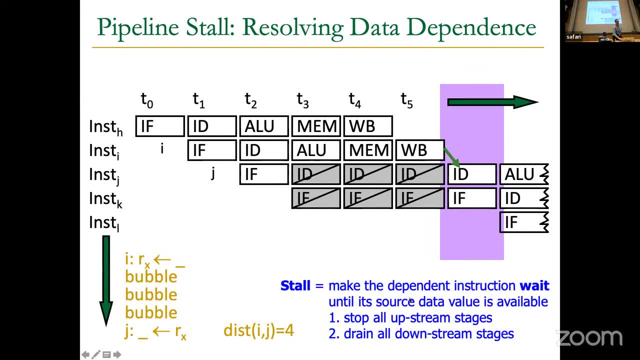 a stall. a stall is. you make the dependent instruction wait until its source data value is available. And how do you do that? You stop all upstream stages, basically earlier stages in the pipeline. You stop them And you drain all downstream stages such that this instruction goes. 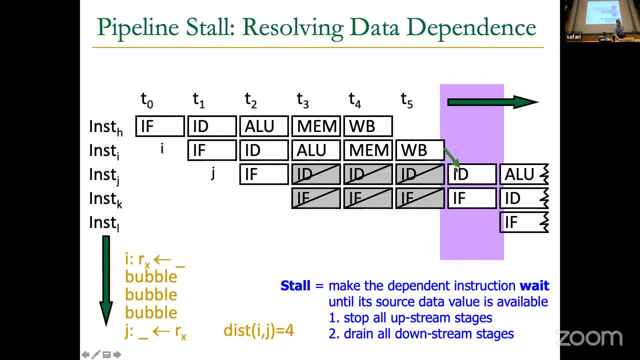 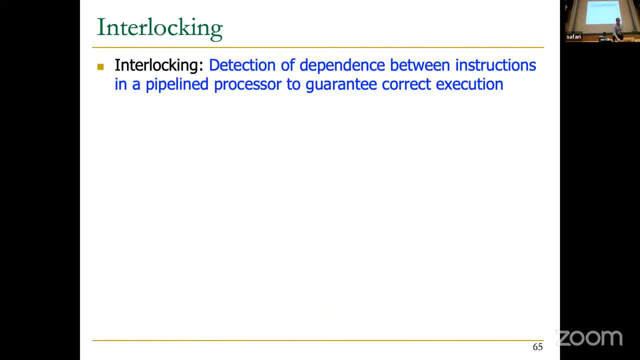 So you drain these two instructions that may be in the pipeline, but you stall all of the instructions that are coming, starting with the dependent instruction. So that's the idea of a stall. So, basically, in order to be able to determine whether or not you should stall, 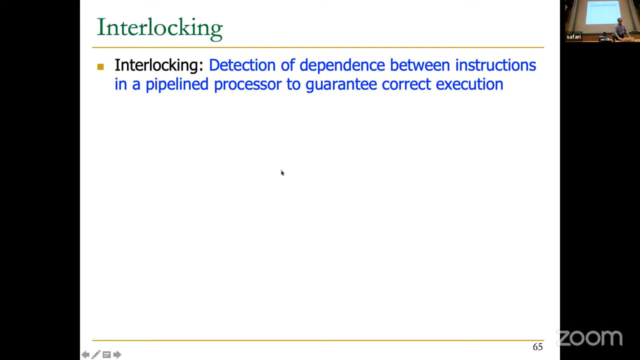 the pipeline, you should detect the dependence between instructions, And this is called interlocking. This is the detection of dependence to guarantee correct execution, And there are two ways of doing it. We've actually talked about both of them: software-based and hardware-based. So software-based is the responsibility of the software to inject. 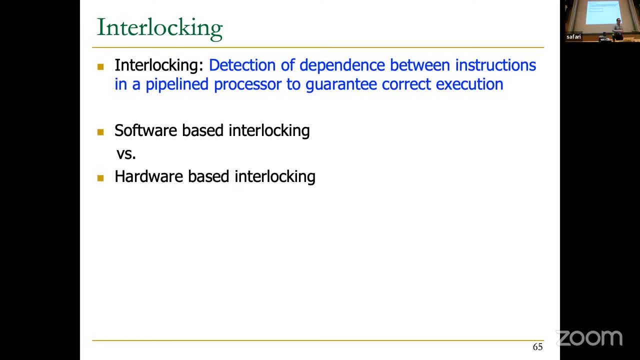 enough NOPs, for example, or reorder the instruction, as we will see later on, such that these dependencies don't happen, And hardware-based is hardware detectees. Does anybody know what MIPS acronym stands for? This is the ISA that we've been looking at. Anybody This is actually interesting. 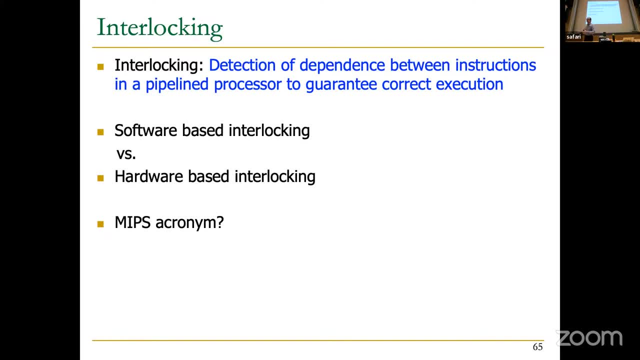 because the designers of MIPS has the philosophy that hardware should be a standard And they designed it as simple as possible and the compiler should do a lot. So they actually went for the first one. They designed pipelines and they said, basically, pipelines should be. 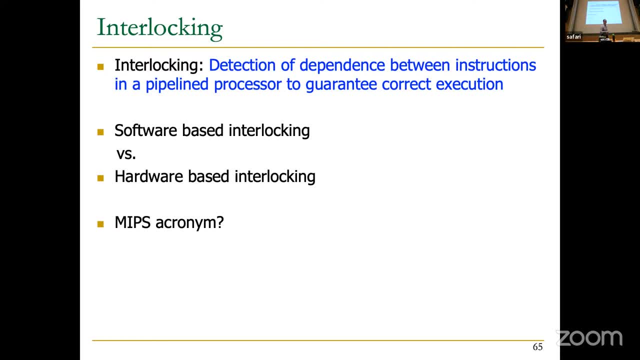 controlled by the software and hardware should not have any interlocking. So MIPS actually stands for microprocessor without interlocking pipeline stages. So now you know how that ISA is designed. But they quickly figured out this is a very bad idea and they went. 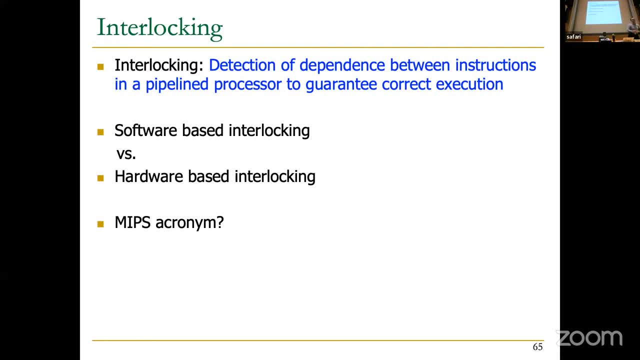 to hardware interlocking. Why? Because it's too much work on the compiler and the software to really schedule these things, These instructions, without any help from the hardware. And once you change the pipeline structure, old software doesn't work anymore, right? So now you have a story about MIPS. 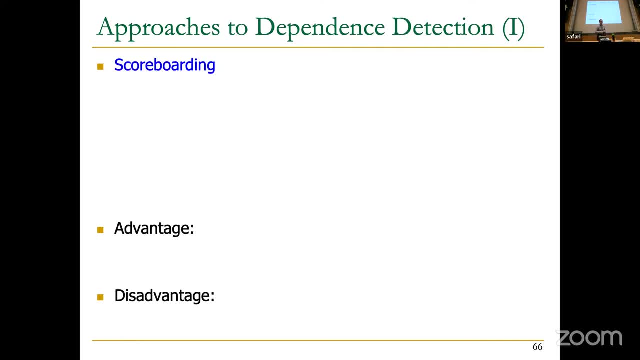 So that's why we're going to cover a lot of hardware, but I'm going to talk about software a little bit also, just to give you the ideas. But there are multiple approaches to hardware dependence detection as well. Scoreboarding is one, So each register in scoreboarding. 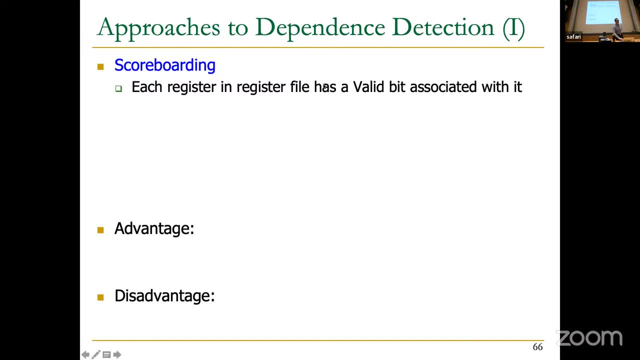 – so this is a technique that's used in some computers. Each register in the register file has a valid bit associated with it. It basically says the value that's in the register file is correct. Okay, that's good. An instruction that is writing to the registers resets the valid bit. So if you're in the 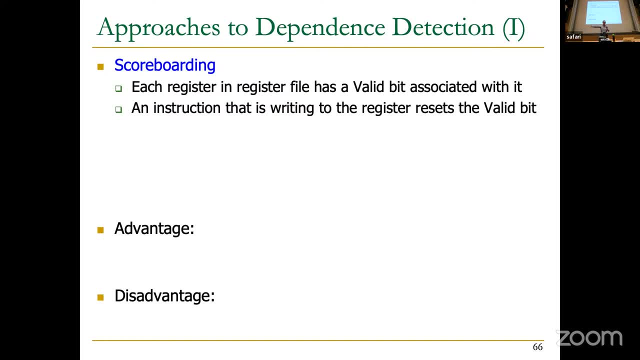 decode stage and if you're going to write to the register after some point, three cycles later, if it's actually a five-stage pipeline, like we have seen, you reset the valid bit saying this instruction is not valid. So if you're going to source this register, wait. 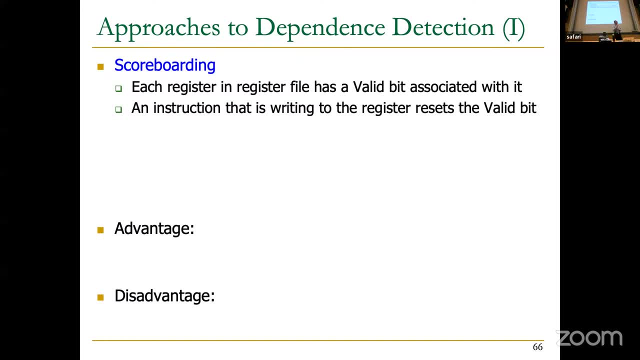 until I make it valid Right. So this is a synchronization. as you can see, It's a bit slow for synchronization – synchronizing between instructions. So basically an instruction in the decode state checks if all its source and destination registers are valid. If both. 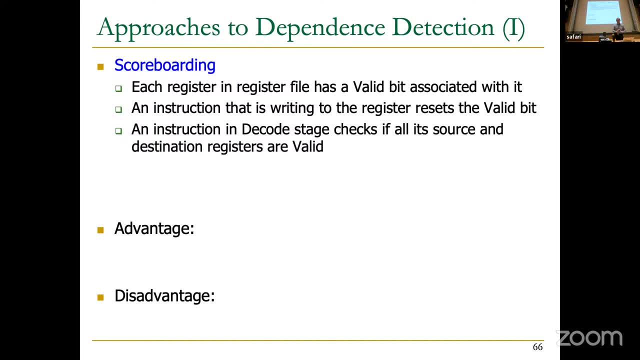 of them are valid, the instruction can move. That's good Because it's guaranteed that there is no instruction in the later stage of the pipeline that's going to produce the value of its source registers. But if one of them is invalid, then the instruction is. 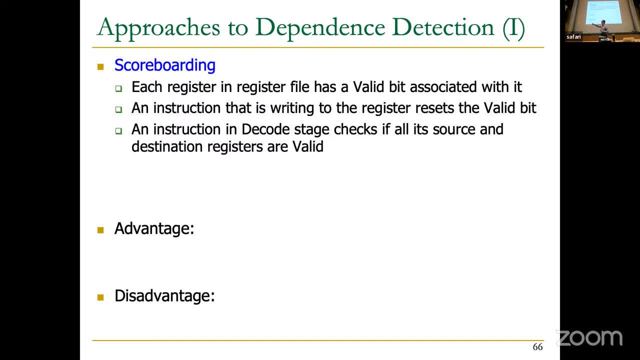 going to stall – until the instruction writes another instruction – or the instruction who set the valid bit to 0, writes to that register and resets the valid bit to 1, OK Yeah, basically that's the idea. So if both of the registers are valid, 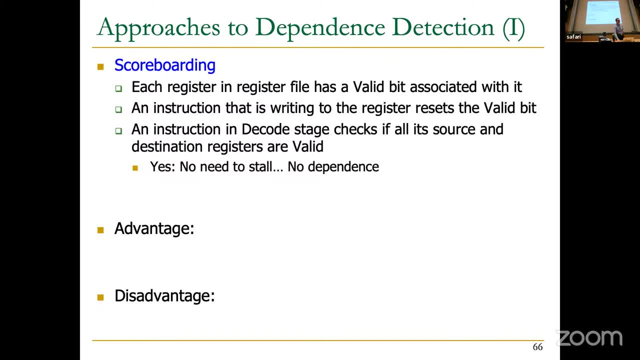 or any of the registers that you're reading, that you're required to read as valid, then you don't need to stall, Otherwise you stall. And this is a very simple dependence checking logic. It's kind of nice, But there's some advances and disadvantages we will see. 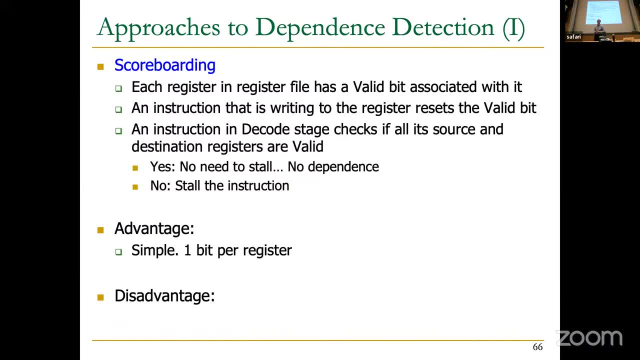 So it's simple. basically, Simplicity is its advantage. One bit per register. you synchronize in the instruction decode stage. when you're reading your sources or when you're writing to register, you reset the valid bit, And when you write to a register in the write back stage. 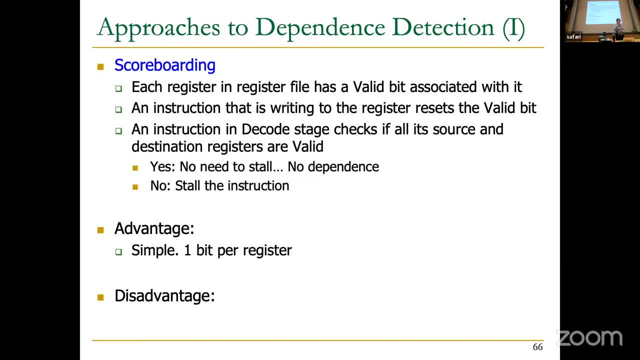 you reset the valid bit to 1 again, You basically are flipping the bit. The disadvantage is that you need to stall for all types of dependencies, actually not only flow dependencies. So really we want to stall only for flow dependencies, right? 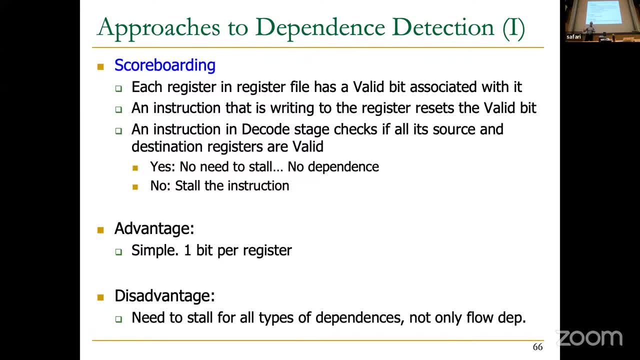 If one instruction is writing to a register and another instruction is writing to another register. we don't want to do that, We don't want to stall in that case, because there is no true communication between these registers. But the way I describe scoreboarding, it doesn't work. 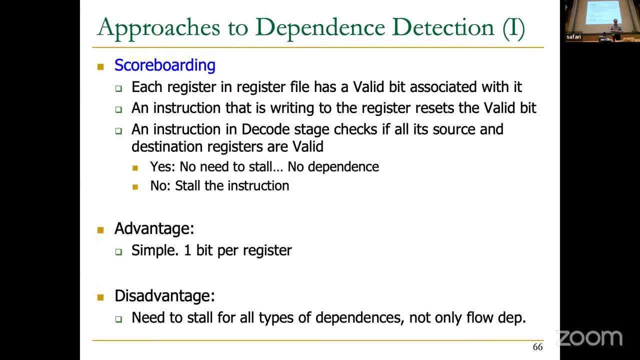 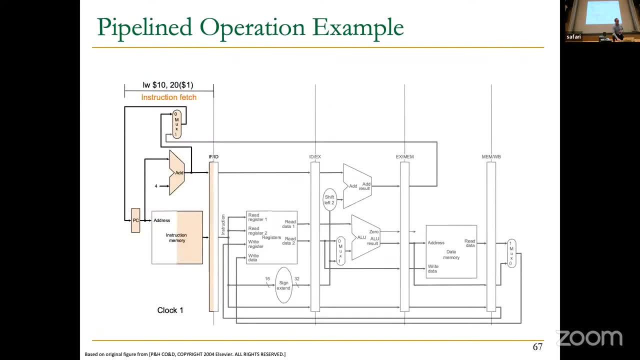 Basically, you need to stall when you have a write after write or write after read dependence. You could actually modify the scoreboard, make it more complicated and make it work, But I'm going to let you think about that. So the other approach: yeah, I think I already discussed this. 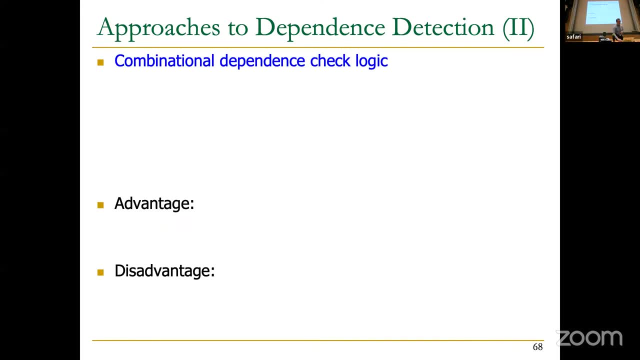 So I will skip this, because it was just basically saying what I just said. Any questions on scoreboarding? It's simple, right? It's a simple way of synchronizing between registers, and the synchronization is done using a single bit per register. 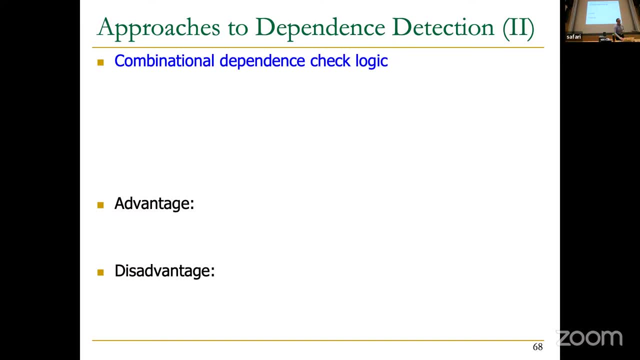 But there's another approach to data dependence detection which doesn't have the disadvantage the first one has, And this is combinational dependence check logic, And the idea is design hardware logic, specialized logic that checks the following: whether any instruction at a later stage is supposed to write to any source. 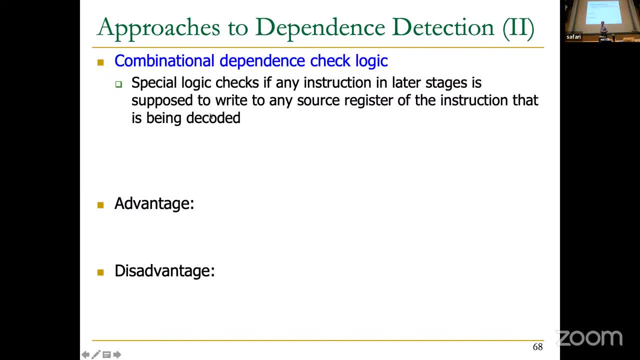 register of the instruction that's being decoded currently. So in the decode stage, you know your source register, You know whether you're reading from a source register because you decoded the instruction. You take some later signals from a later pipeline stage, all later pipeline stage actually. 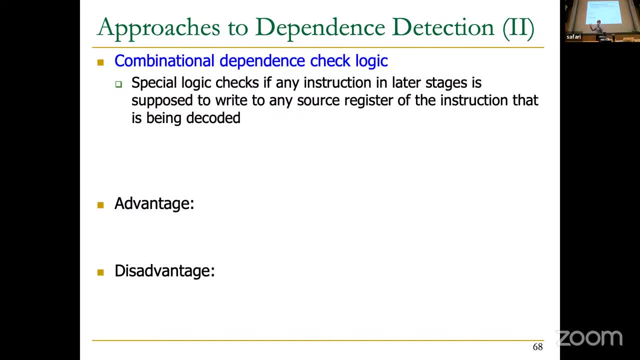 and compare whether the source register you're reading from is the same as the destination register that a later instruction is going to write to, And you should also check whether that instruction is going to write to a register from that stage. Makes sense, right? 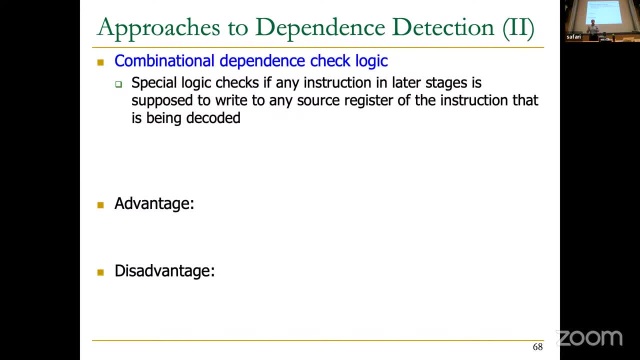 Now you have a hardware computational logic that's an equality check Checker on the source register and destination register numbers across different stages- And we're going to see this probably in the later lecture- And if this logic says I detected some dependence, you stall the instruction and the pipeline. 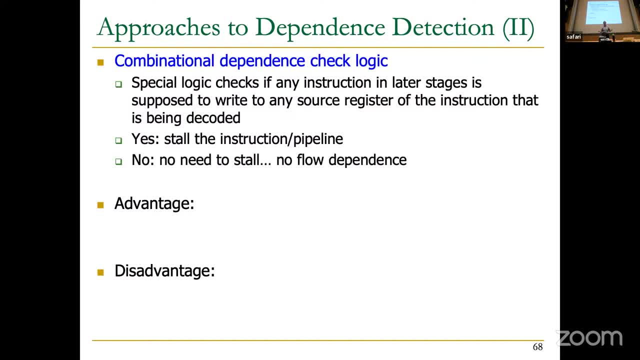 If it says no, then there's no need to stall because there's no flow dependence. Now you can make this logic, But basically the way I describe this logic is just for flow dependencies. You don't need to check whether this instruction that's. 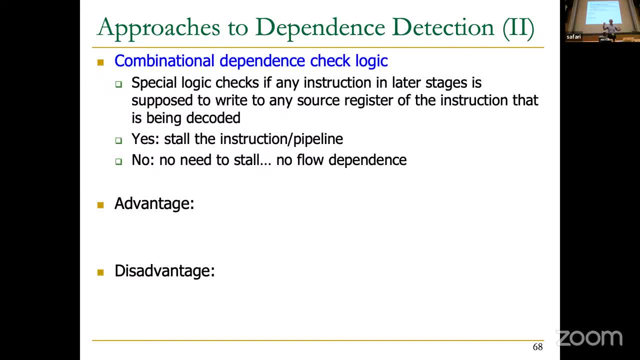 writing to register is writing to register. That's also written by an instruction that's later in the pipeline. You don't need to do that checking because that's not a real dependence. So that's the big advantage: There's no need to stall on out and tie an output dependence. 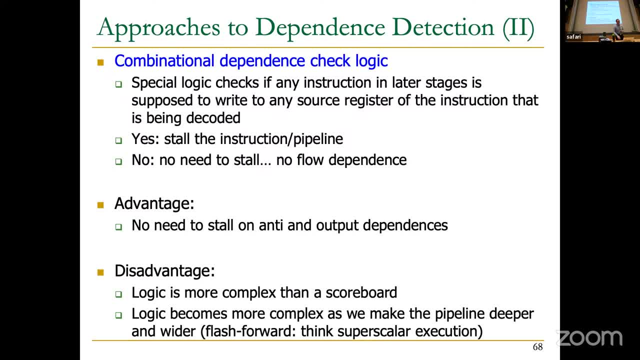 in this particular case. But the disadvantage is, logic is more complex than a scoreboard. It's not as beautiful and simple as a single bit that's used for synchronization, And actually logic becomes more and more complex as we make the pipeline deeper. So if your pipeline is five stages, 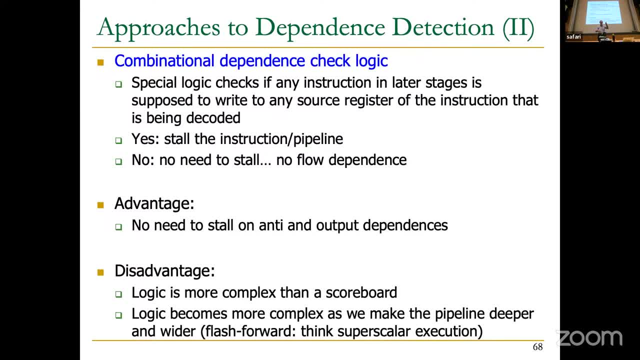 in the decode stage- that's the second stage- you stall the instruction. That's the second stage. You basically compare to three possible other stages. Now, if your pipeline is 25 stages, assume that decode stage is your second stage. still, you need to compare to 23 other stages. 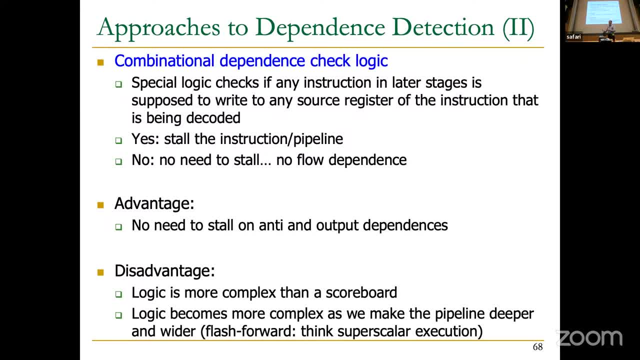 because all of those 23 other stages can potentially be writing to a register that you are going to source. So now you see the complexity. Now we're going to also see something called super scalar execution. So your pipeline can be deeper, 25 stages, let's say. 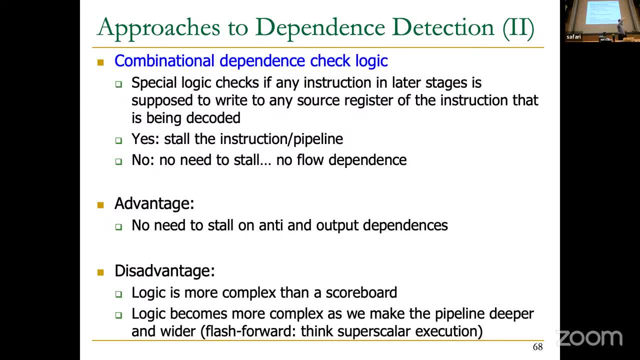 We're going to add actually, concurrent execution across instructions, Right? So instead of fetching one instruction, we're going to fetch four instructions or eight instructions, And that's going to increase our parallelism. Now, dependence checking logic like this becomes very, very complicated once you do that. 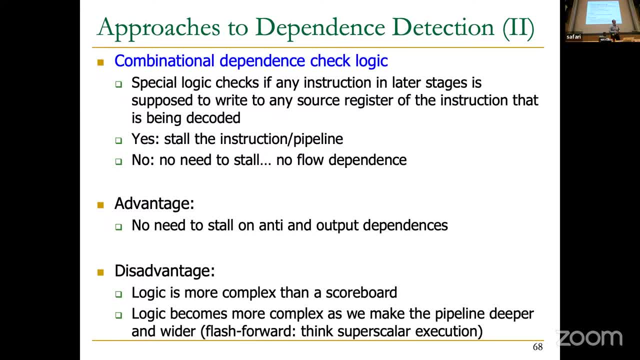 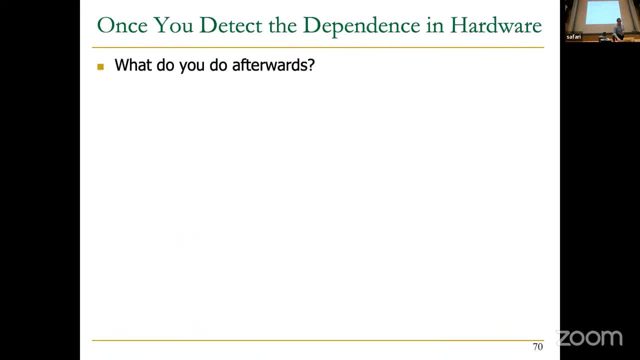 OK, so let's not get ahead of ourselves. but now you kind of know the concept of where we're going: towards super scalar execution. OK, I think I've already talked about this. So once you detect the dependence on hardware, what do you do afterwards, is the question. 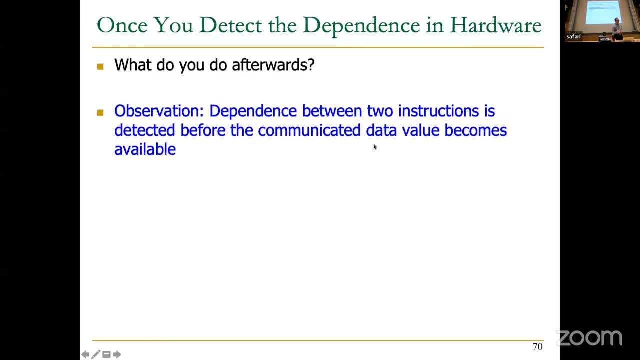 Basically, dependence between two instructions is detected before the communicated data value becomes available. That's an important observation. You can detect the dependence before the data value becomes available, So there are multiple options. as a result, You can stall the dependent instruction right away. 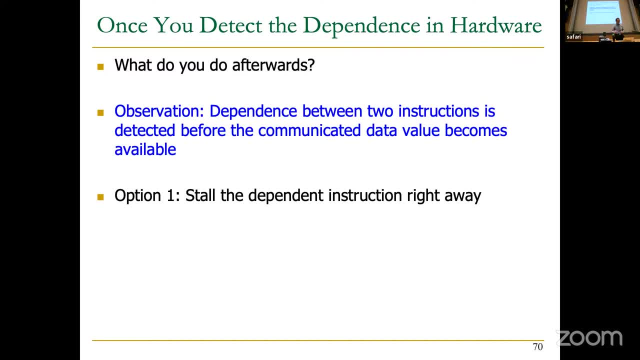 saying I'm not going to move this instruction from the decode stage and wait until the value is available in the register file. Or you can be a bit more aggressive and move the instruction in the pipeline, as long as it's going to get the correct value. 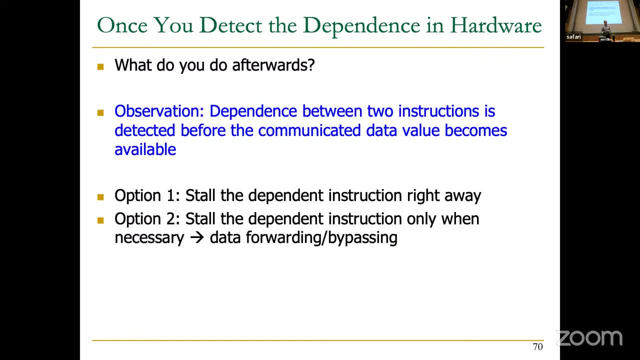 Stall the dependent instruction only when necessary. This is called data forwarding, meaning if you can actually move this instruction a little bit and you can have a bypass path from a later stage to wherever you move this instruction, you're going to still get the correct value. 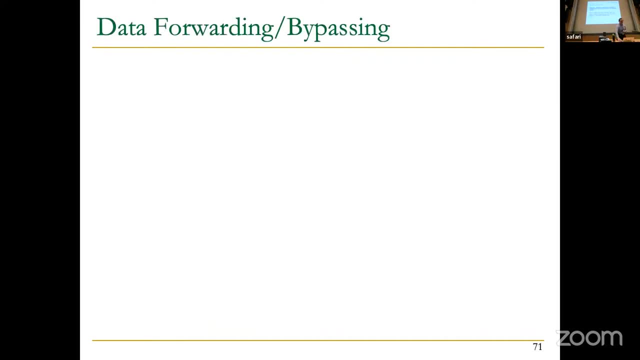 This is called data forwarding and bypassing, And there could be other options, as we will see. So let me introduce this concept and then we're going to be done for today, And then we're going to pick up with how to do data forwarding. 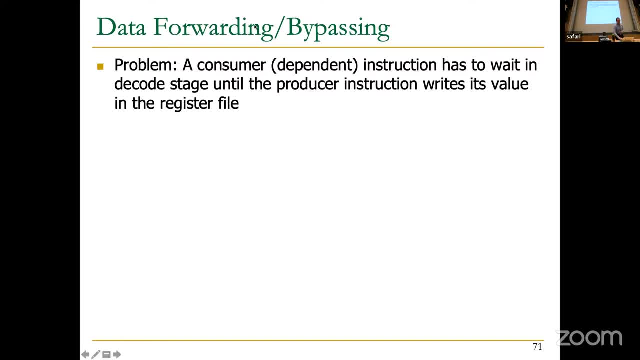 how to do these relatively aggressive optimizations. So the problem is, if you just stall right away the dependent instruction decode stage, a consumer or dependent instruction has to wait in the decode stage until the producer instruction writes its value into the register file. And we said that this is conservative. 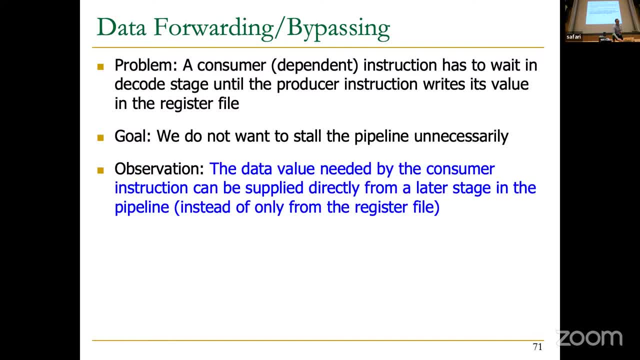 Basically, our goal is not to stall pipeline unnecessarily, And the key observation is: the data value needed by a consumer instruction can be supplied directly from a later stage in the pipeline with a wire. This is the value I produced. Here's a wire. 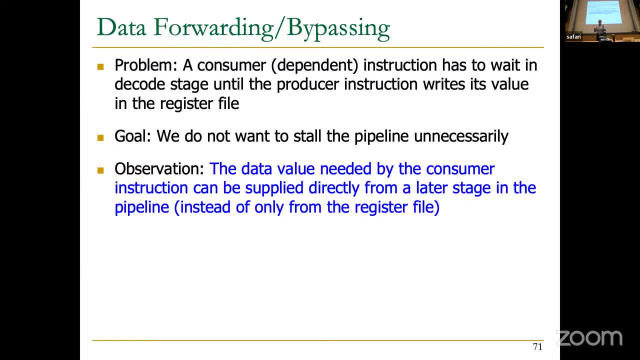 Get the value. We don't need to go through the register file. basically Cut the communication latency Let's, instead of from the register file. Basically don't wait until the value is written into the register file. Add more hardware to supply the value. 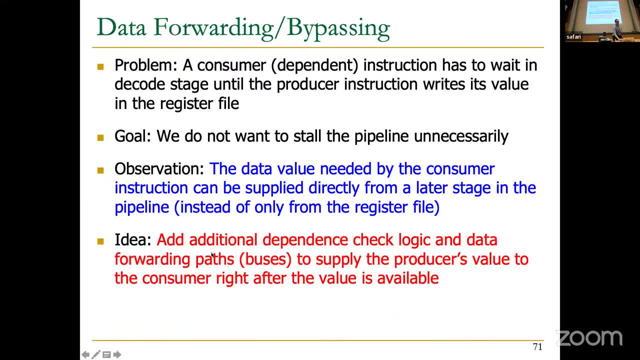 So, basically, the idea is to add additional dependence check logic and data forwarding paths, meaning buses or wires- to supply the producer's value to the consumer right after the value becomes available. Of course, you need to add the control logic, which is the dependence check logic, over here. 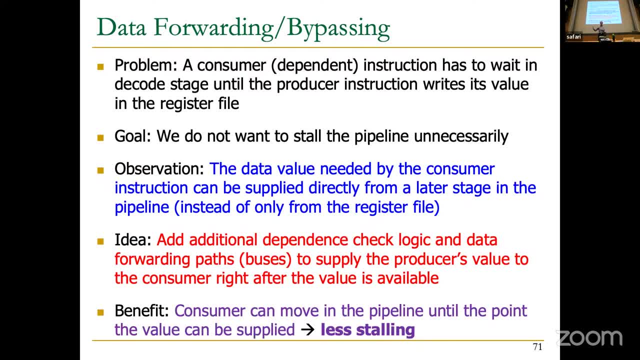 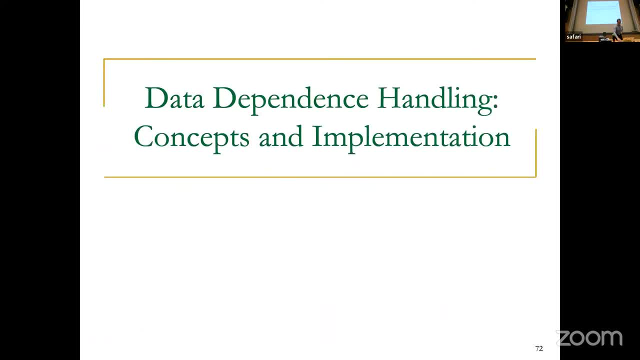 Now, the huge benefit here is: consumer can move in the pipeline until the point the value can be supplied, so you have less amount of stalling. OK, So this is a great place to stop, as you can see. Now the next lecture will start from here.